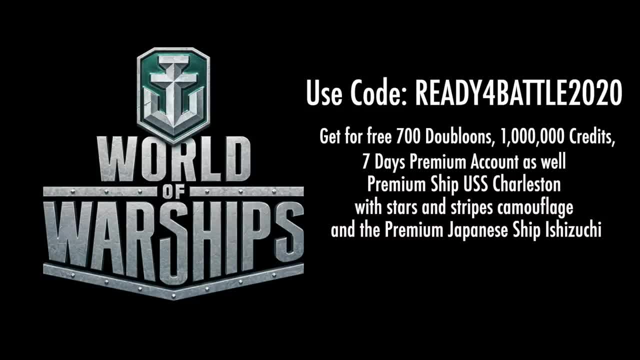 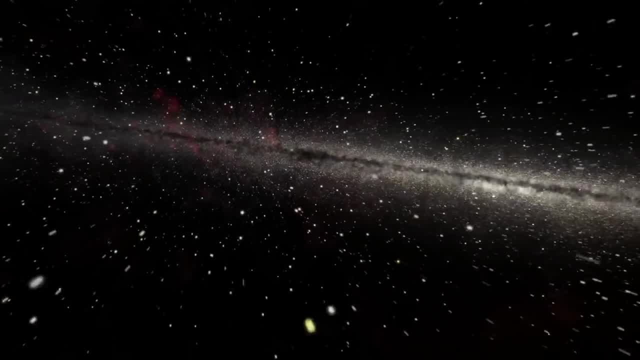 This video is sponsored by World of Warships. As we stare out at the great wilderness that is the Milky Way Galaxy, one thing stands out: We see no one else, at least so far. This has led to one of the more intriguing and perhaps even probable. 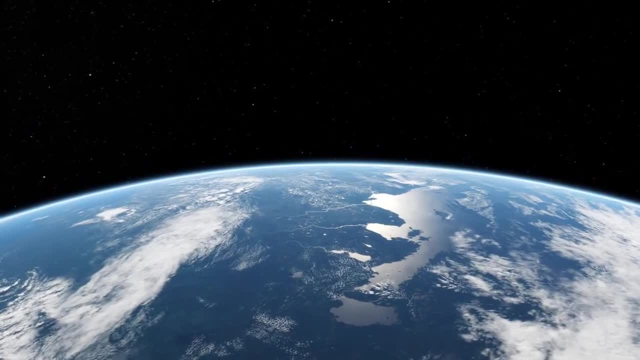 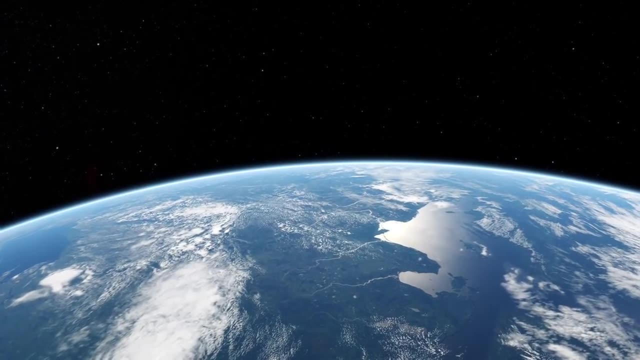 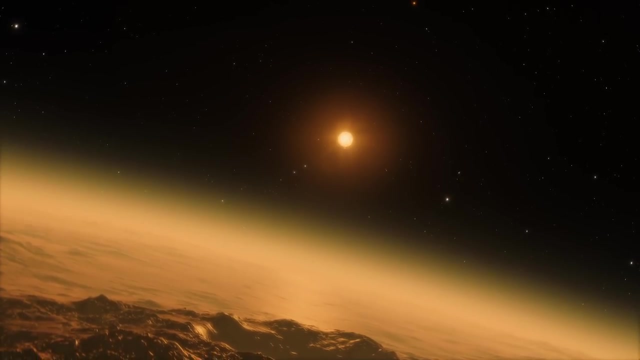 solutions to the Fermi Paradox, that we humans are very early in the game and have only just appeared, right at the time that such a civilization is possible in the galaxy, This idea that there is or was something out there that simply reset any surface life on exoplanets. up until this point, 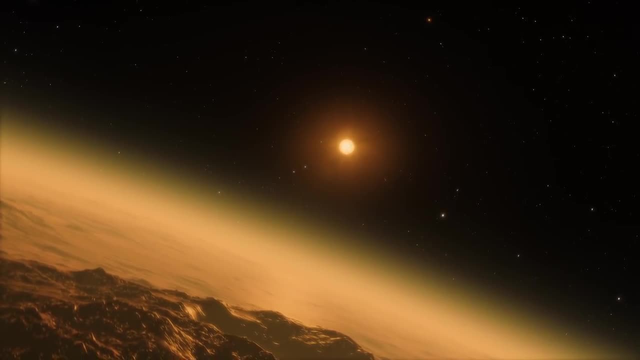 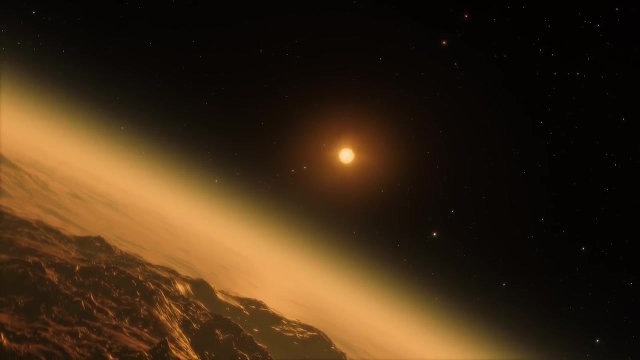 that has since declined in frequency enough for us to exist is one of the solutions that's gaining traction within astrobiology. My guest today has advanced just such a solution: that gamma ray bursts may have been the culprit and as they decline, we may see. 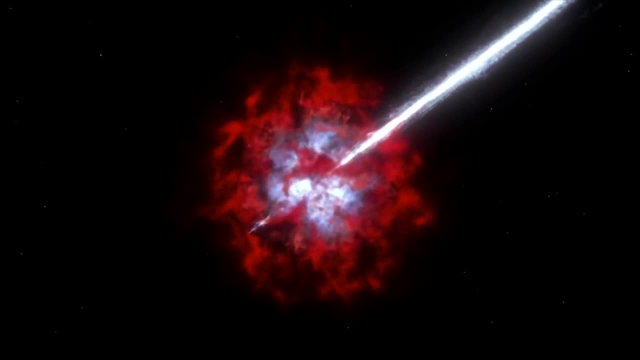 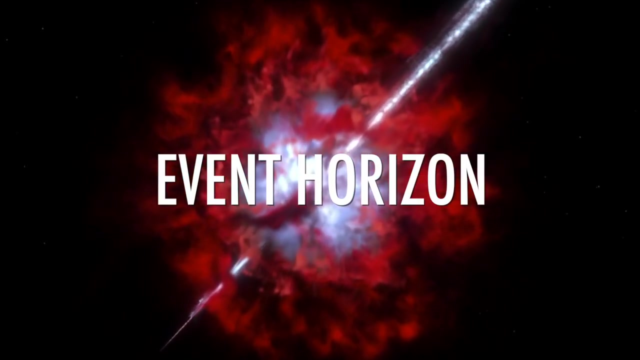 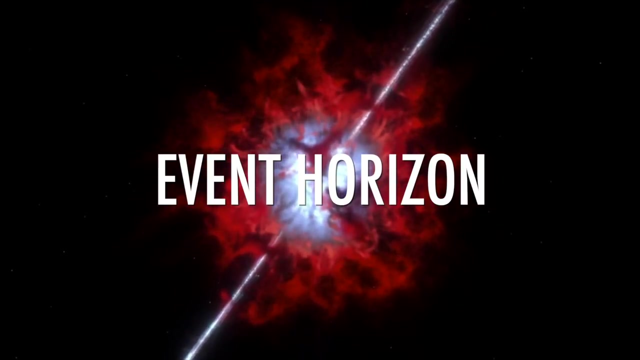 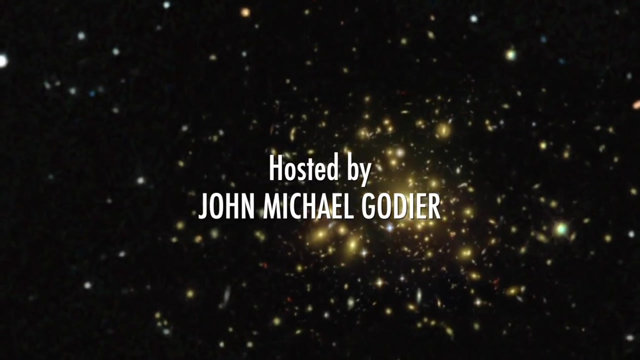 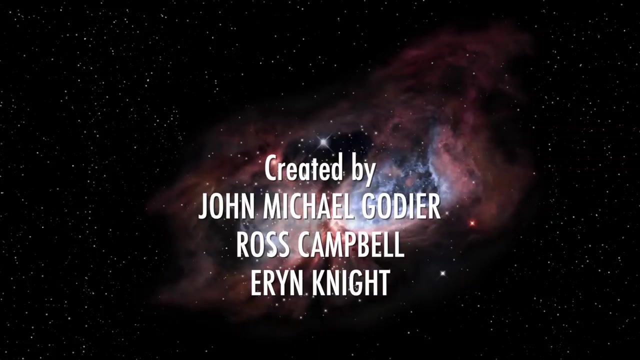 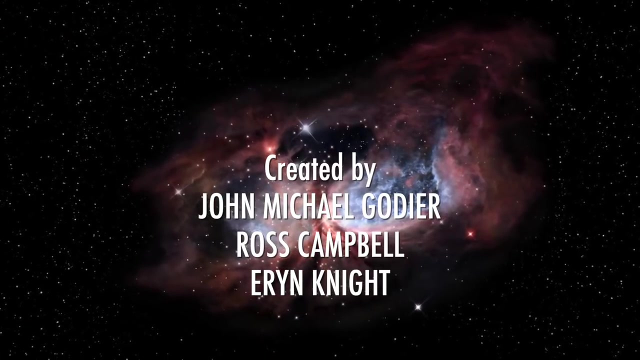 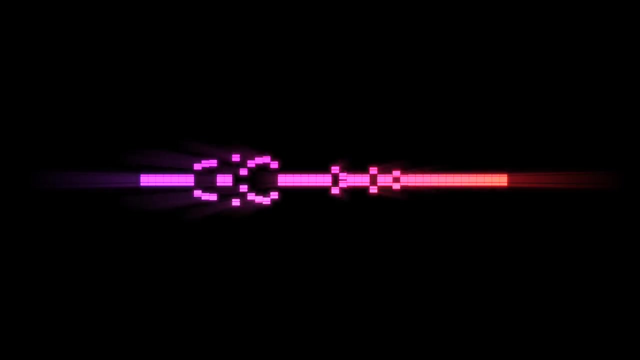 a blossoming of intelligence in the universe as it finally becomes safe for intelligent life. You have fallen into Event Horizon with John Michael Godier. In today's episode, John is joined by Dr James Annis. Dr Annis is a senior scientist at the. 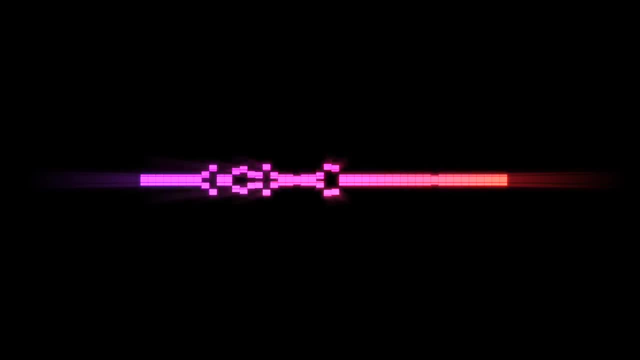 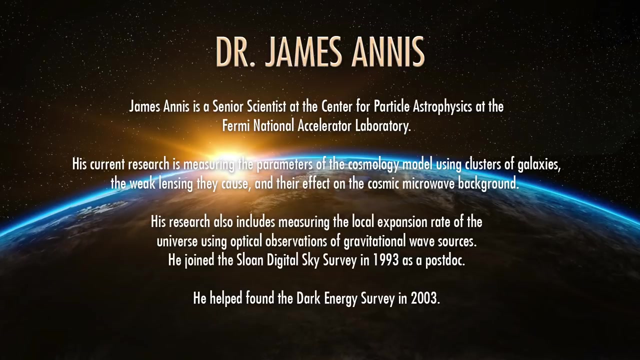 Center for Particle Astrophysics at the Fermi National Accelerator Laboratory. His current research is measuring the parameters of the cosmology model using clusters of galaxies, the weak lensing they cause and their effect on the cosmic microwave background. His research also includes measuring the local expansion rate of the universe. 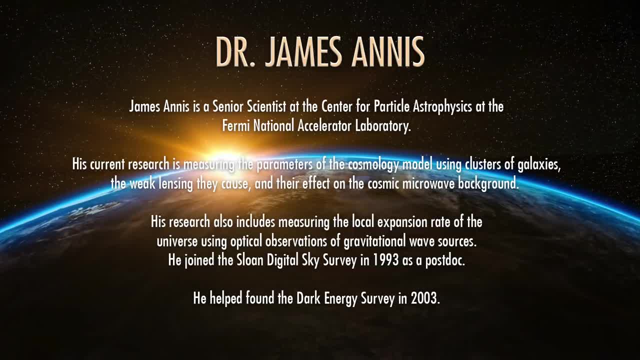 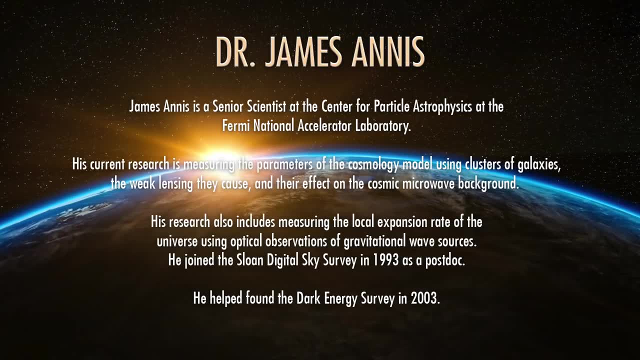 using optical observations of gravitational wave sources. He joined the Sloan Digital Sky Survey in 1993 as a postdoc. He helped found the Dark Energy Survey in 2003.. James Annis, welcome to the program. Well, thank you. thanks for inviting me. 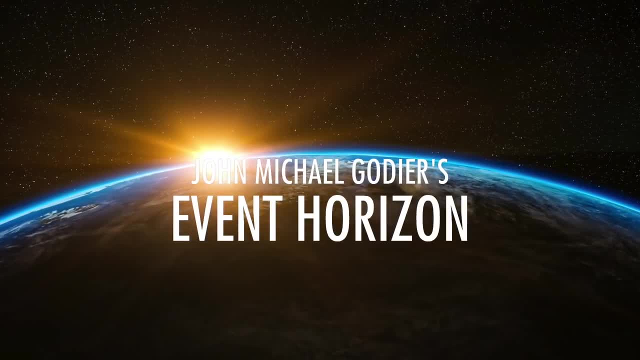 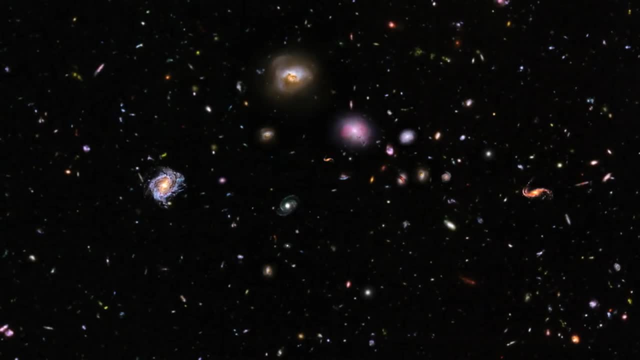 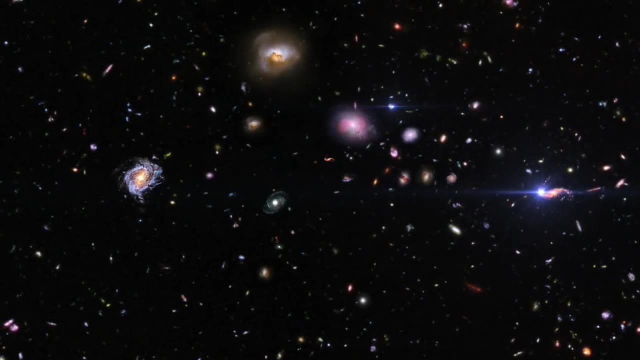 Now, Jim, in 1999 you authored a paper detailing a solution to the Fermi Paradox, one of many, many which you know. I've heard of tens and tens of solutions to this, But yours is interesting because it's astrophysical in nature and says that well. 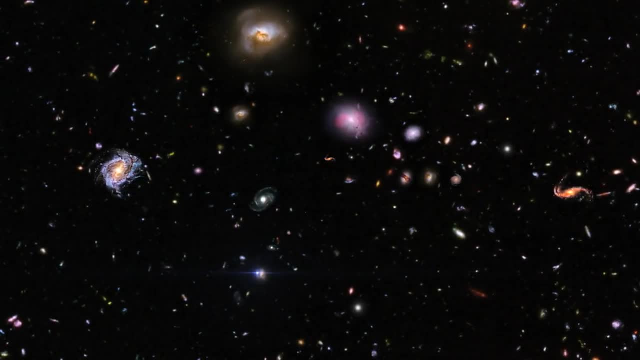 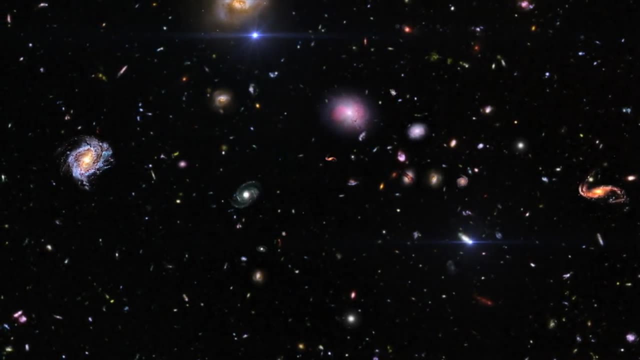 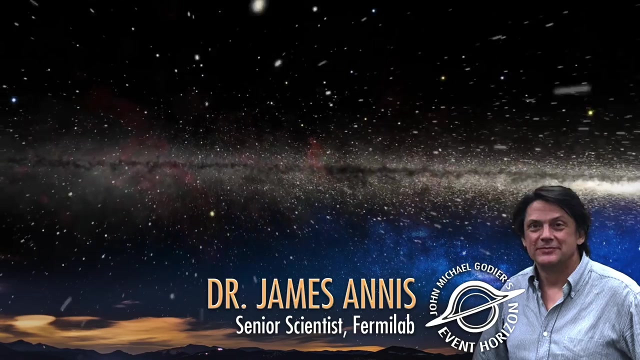 maybe there was something- gamma ray bursts- present in the universe that made it dangerous and that intelligent life was not possible here until now, or not possible in the Milky Way at large. Can you give us an overview of that? Sure, I'm going to start with the Fermi paradox. 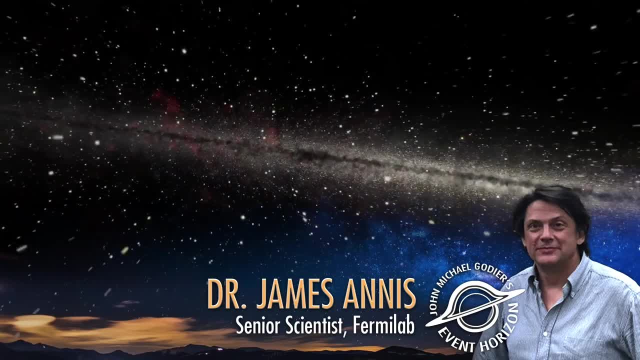 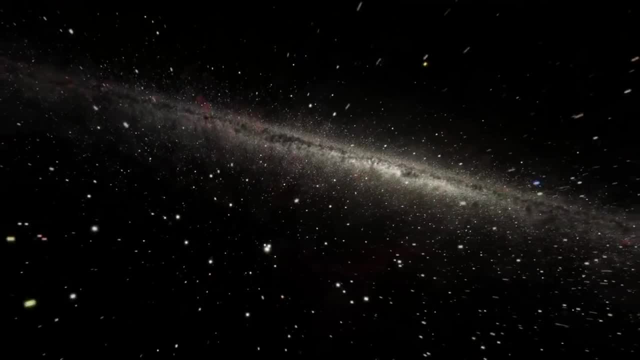 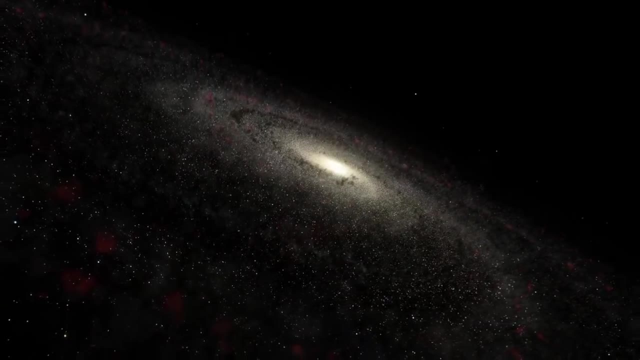 I know your listeners have heard this before, but it's the starting place and it leads me into the question of time. So the Fermi paradox, essentially, is that the galaxy is quite old- 10,000 million years- but it doesn't take very long for a space-faring civilization to go across. 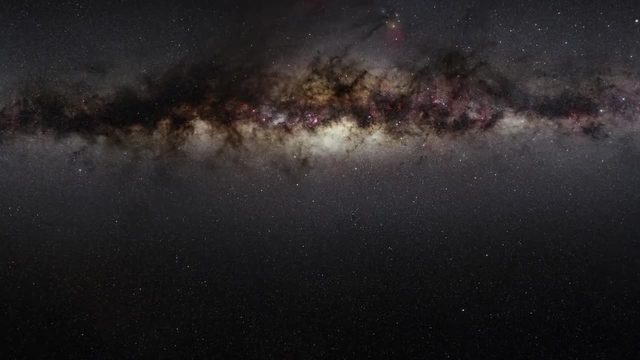 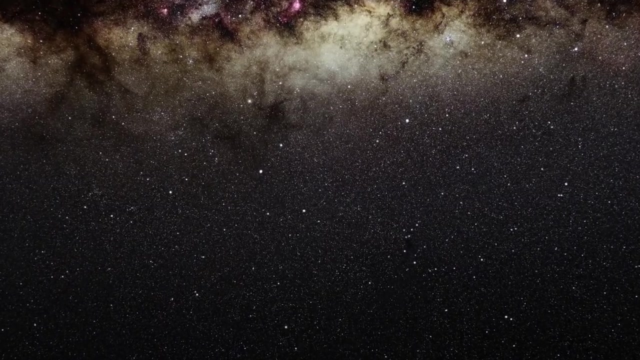 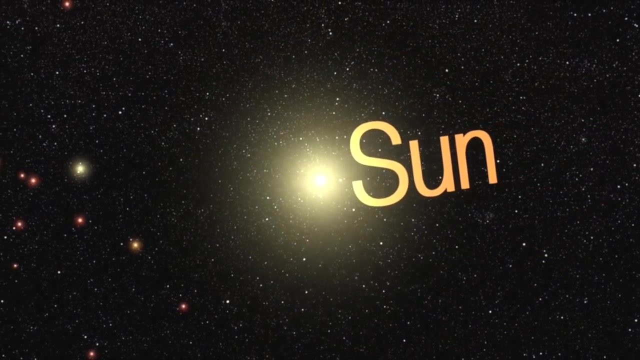 it at any decent speed. Even Earth orbital speeds take maybe 10,000 years to get to the next star over. That sounds like a long time, but that's not a long time to cross the galaxy. To cross the galaxy takes 100 million. 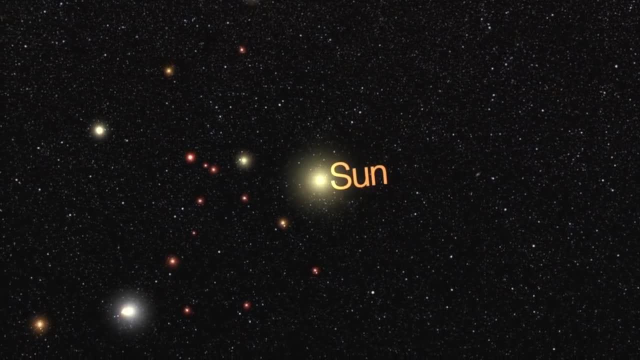 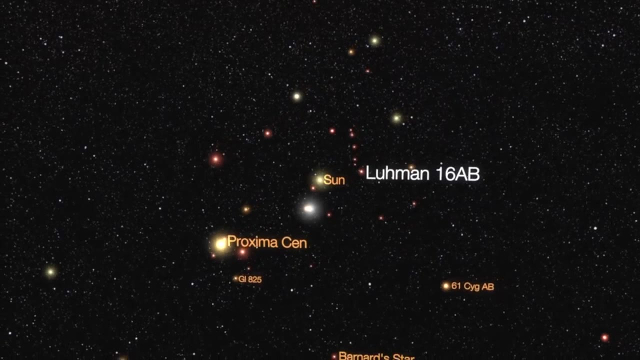 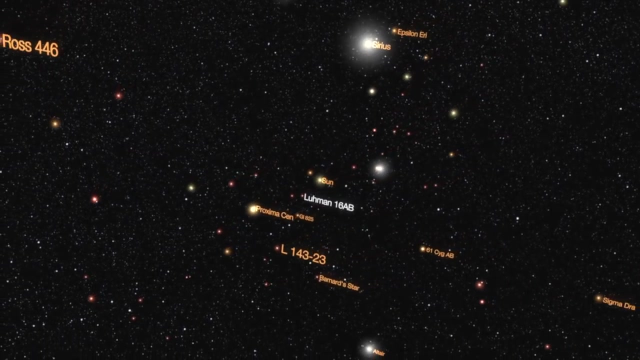 years. We're not used to thinking about time in that way. We're not very good at it. The astronomers are. but the astronomers tend to work in units where the number is one like one age of the universe or 1 billion years. I'm going to work in millions of years because 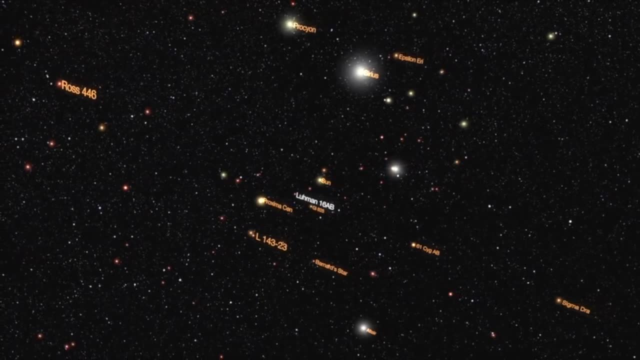 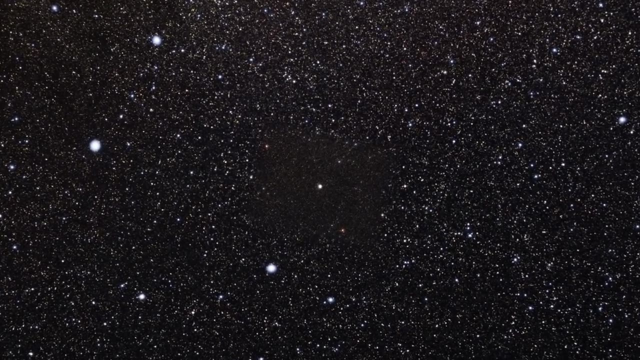 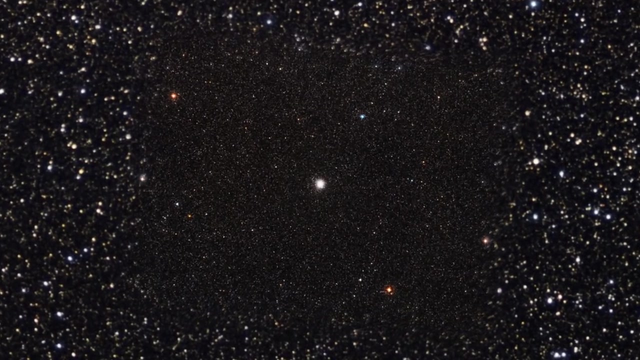 a million years is the lifespan of the most massive star and it's the lifespan of the species. It's kind of the right time scale for this problem And in this problem if it takes 100 million years to cross the galaxy, but the galaxy is 10,000 million years old. 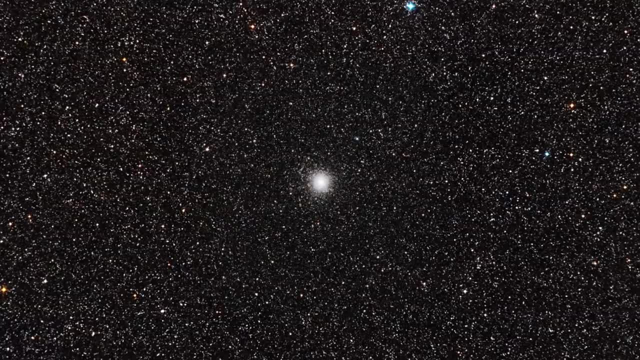 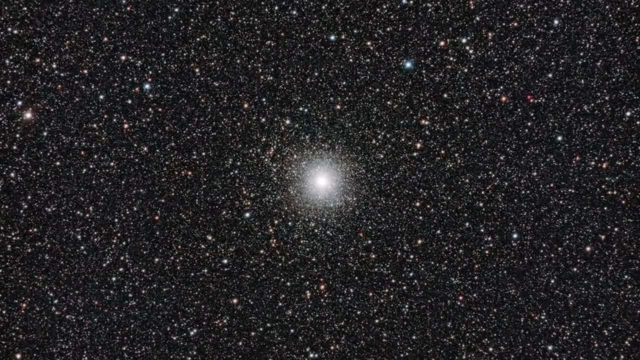 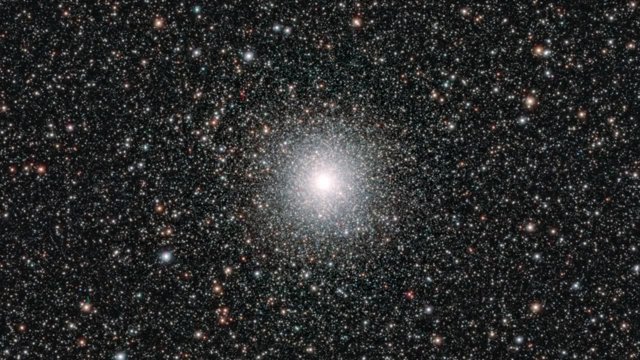 that's practically no time at all. If intelligent life becomes space-faring civilization, then it should cross the galaxy like a wildfire seen by the galaxy. And that's a problem because there's not a whole lot of evidence that ever happened. Our idea of what time 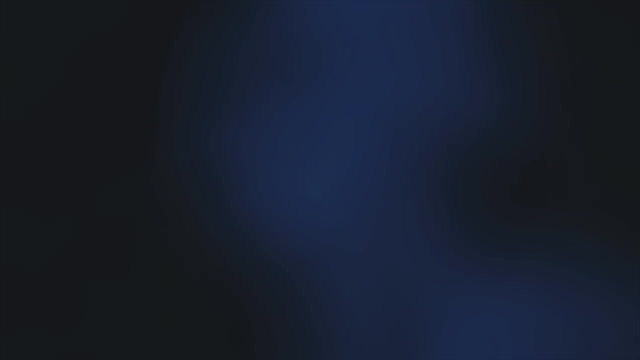 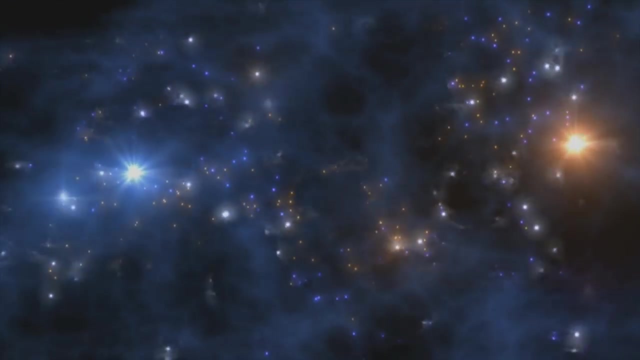 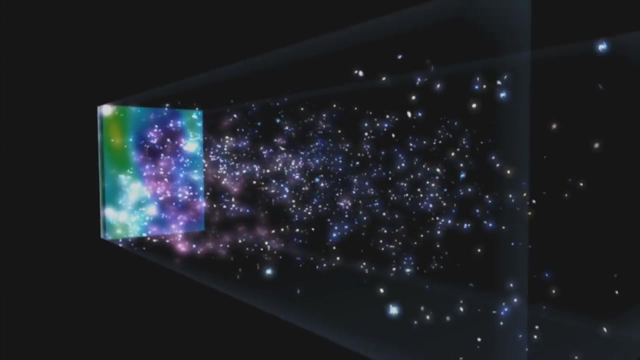 is is based on human time scales. a century A century is long if we're looking for proof of some theory, But in astronomy a million years is nothing. It just doesn't mean anything to us. 100 million years is getting there. The galaxy takes 200 million years to rotate. 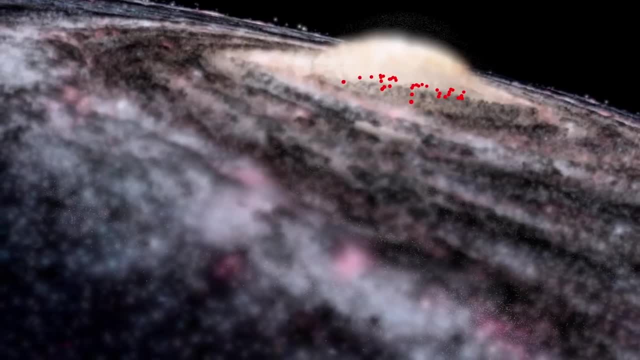 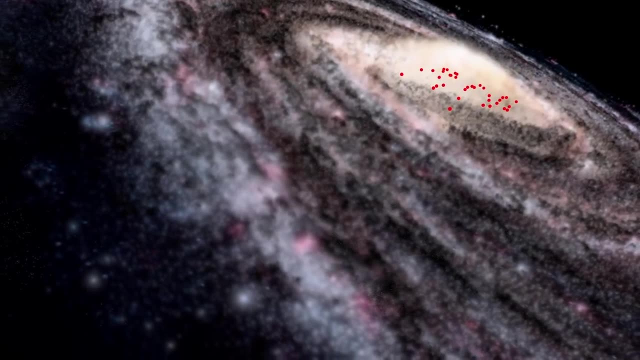 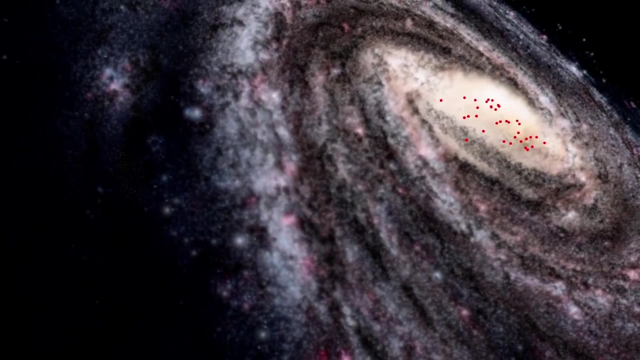 That might not be relevant, but it is. If you're just diffusing across the galaxy, star by star, because that's what you do as a space-faring race, the galaxy rotation itself will smear out your culture, your planets that you have reached, the stars you have seen in a smear pattern around the whole. 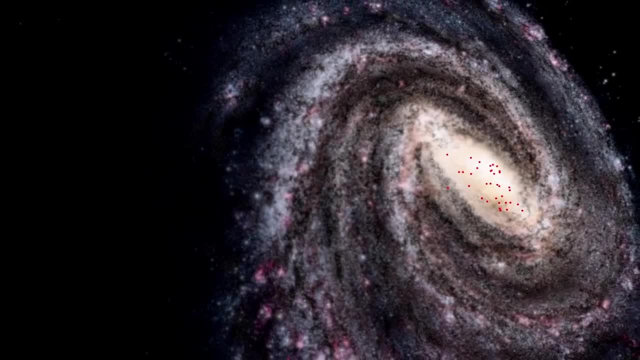 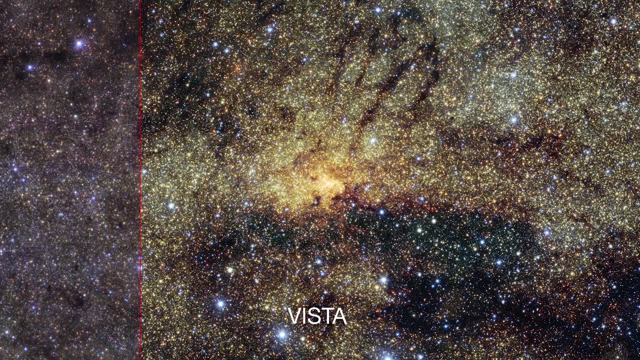 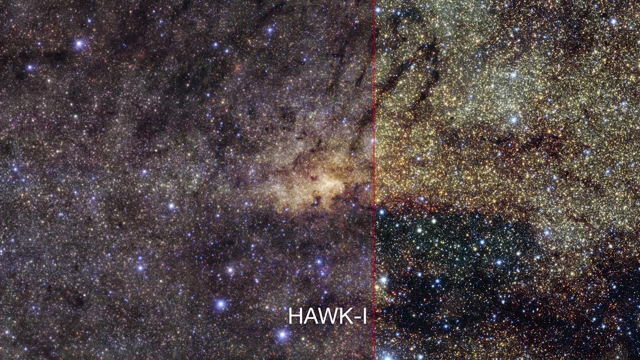 thing in 200 million years. It's just pretty easy for a space-faring civilization to cover a galaxy in a short amount of time. Yet we see absolutely no evidence that it has. You know, the solar system appears to be exactly as it formed. You know, we look out. so far we don't see radio signals. we 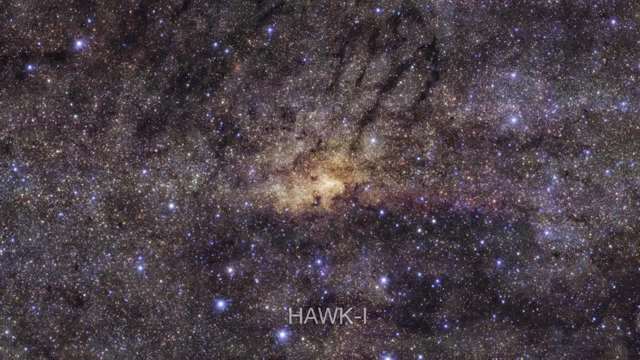 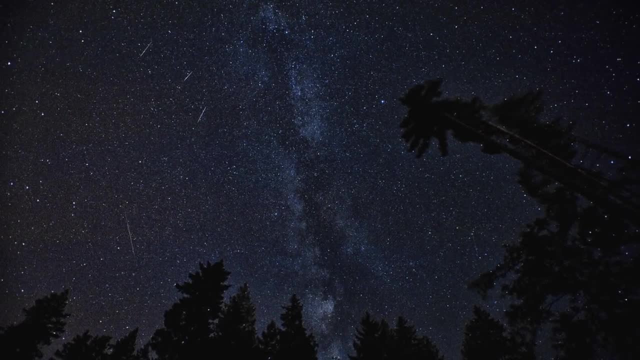 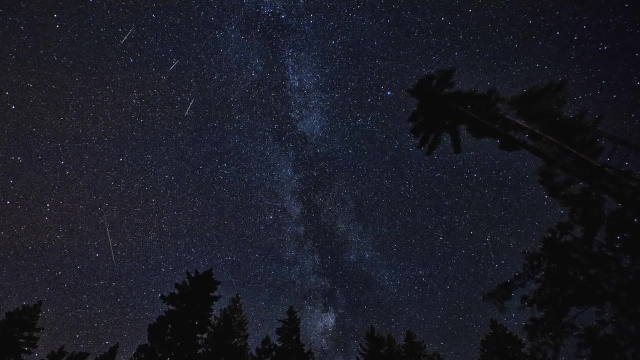 don't see giant alien megastructures. no evidence of anyone out there, And this has been called the Great Silence- that we simply see no evidence of anyone except ourselves. It's incredibly natural-looking, very wild-looking out there. I mean, it may be a bit underappreciated If you look around the solar system it's. 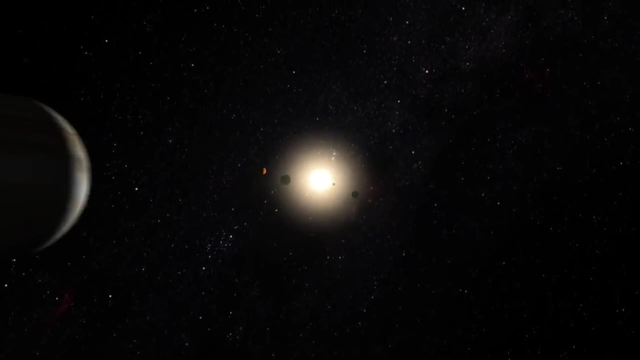 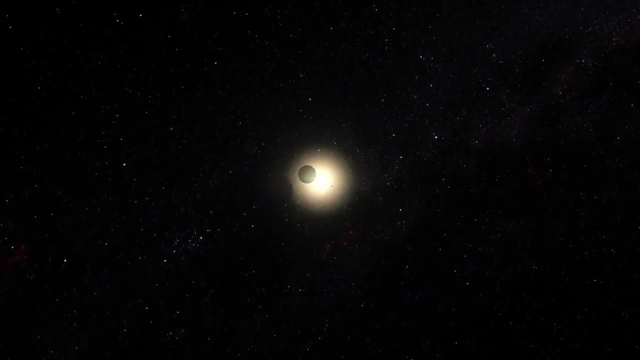 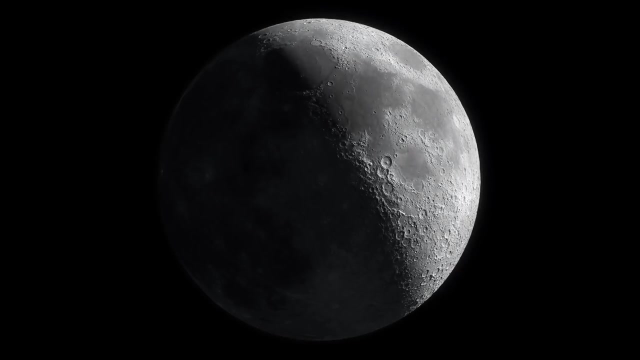 more than it doesn't look like. there's evidence for it Today. these days, people are looking for single probes, Or this great idea I heard was to use lunar orbiter data to go looking for a non-Apollo artifact on the moon. There'll be Soviet spacecraft, there'll be a Chinese. 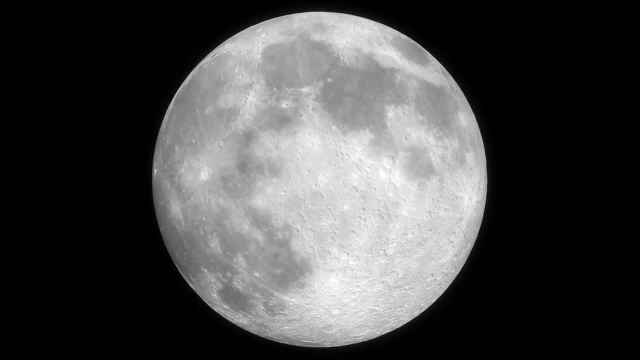 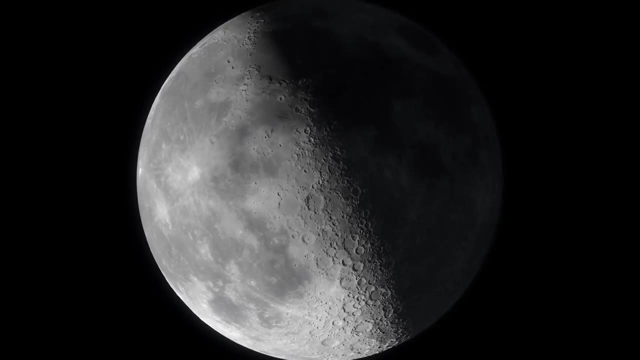 spacecraft. Is there anything else you can see? But if the- I mean you have to understand on a million-year timescale- if there were aliens that had moved through the solar system and were here for a million years, the solar system would look. 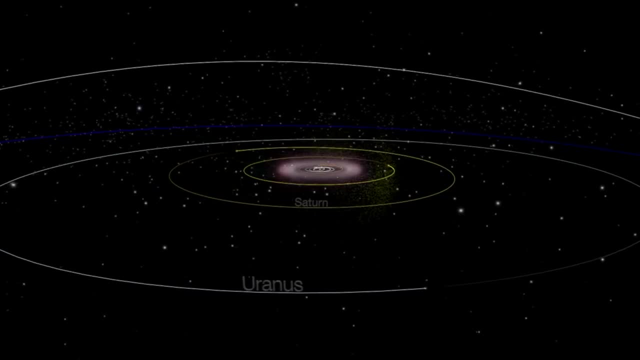 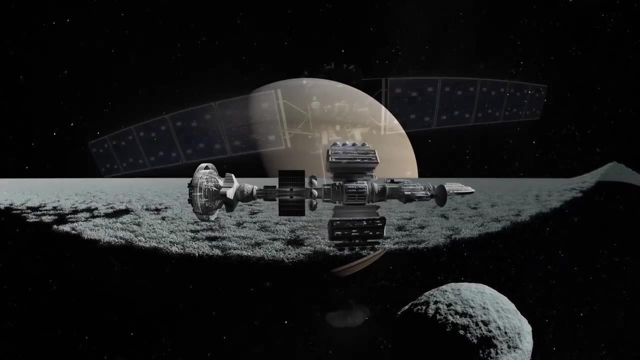 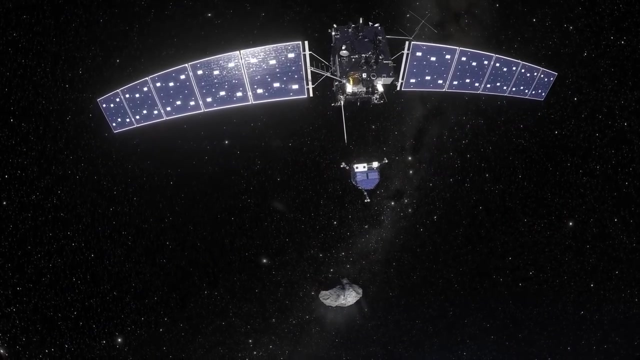 nothing like what we're seeing. It would be engineered, it'd be tamed. it would look vastly different than rubble piles that we see from the moon to most of the asteroids. You know, the most exotic thing in the solar system might be Miranda, and even that looks. 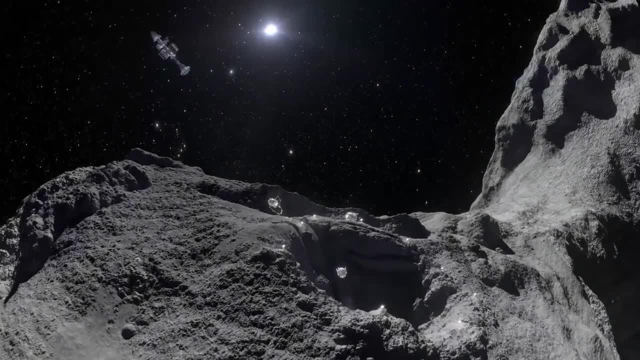 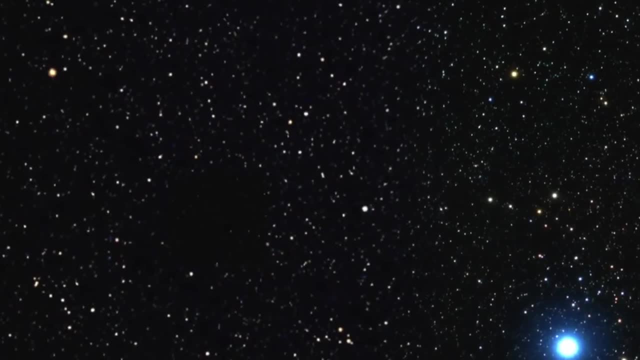 like a reconstituted rubble. And if you move out into the other rest of the galaxy, it's the same thing. It just looks natural. And I mean, I'm an observer, I study galaxies by trade, by craft, That's what I've. 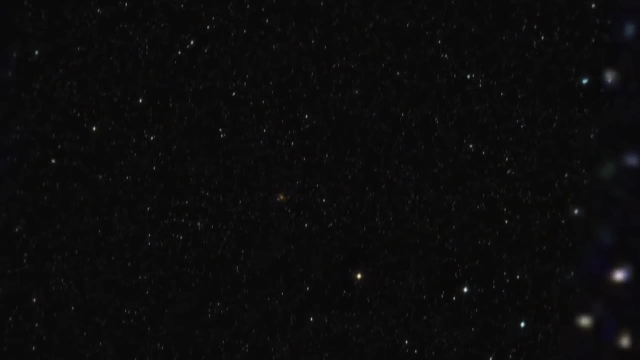 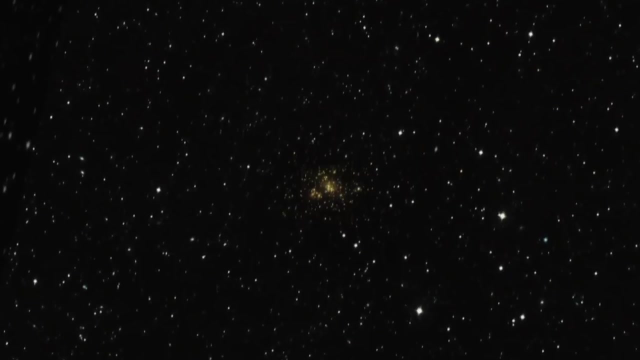 been doing for my entire career As observers. we have a whole bunch of these exotic galaxies. We keep them in our pockets, we talk about them. One is Hoag's object and it's this giant ring of gas and stars around the galaxy. 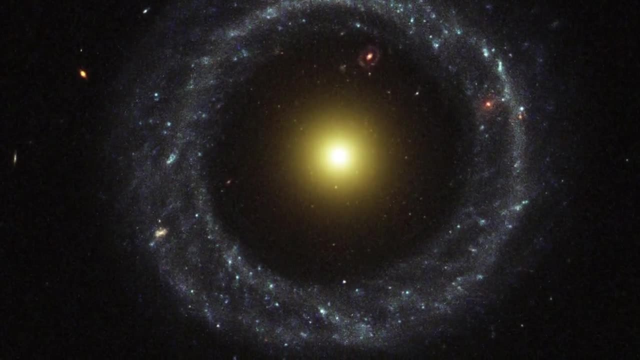 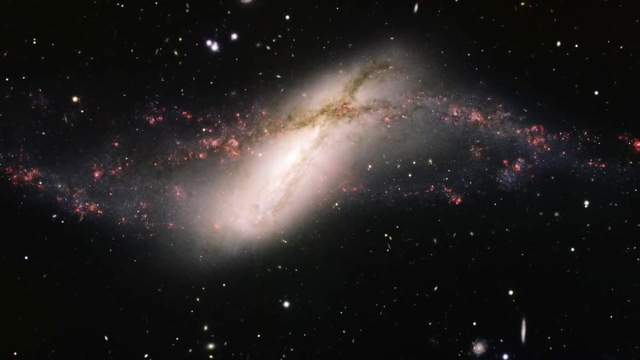 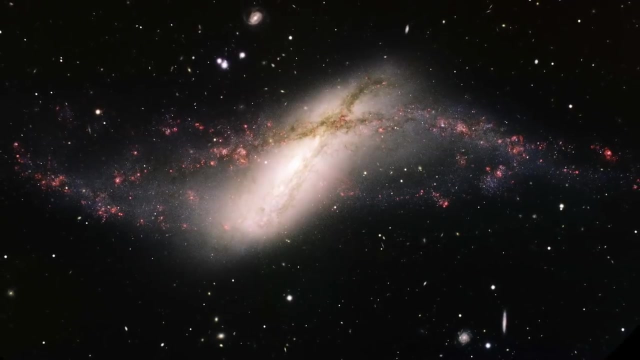 And there are things called polar ring galaxies, That's, more stars around the ring galaxy, That's like NGC 660, to give you a code number which you can Google and see these things. You look at them and they look natural. They don't look engineered, even though they're. 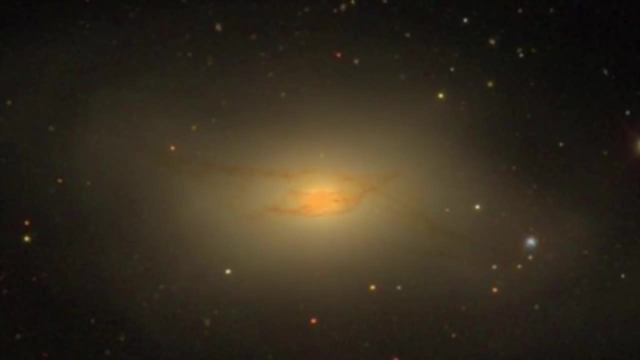 exotic galaxies. There's this great galaxy in Virgo. If you look at it, it's NGC 4753.. You go look in the center of it. it has these dust lanes, But dust lanes even they. they look like a Lissajous pattern, But that turns out to be really easy to produce when you 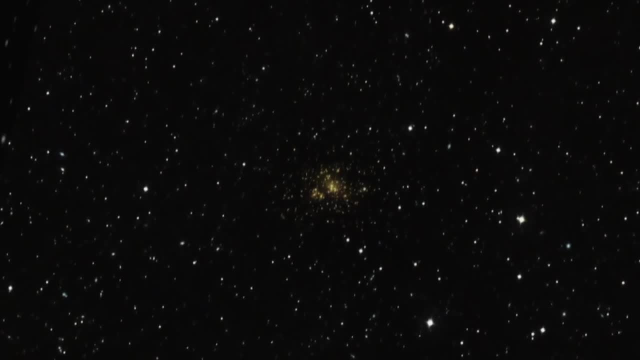 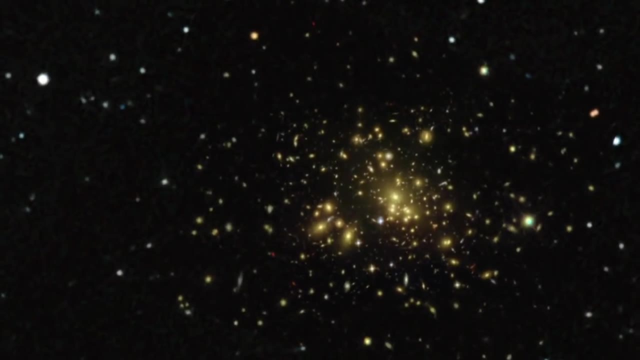 throw galaxies at each other. When we look around, you know, as a scientist, we want to interpret everything as natural and we do that well. But if you just look at the images- the solar system, the galaxy, the nearest galaxies- they all look wild and natural, like they've not been touched by. 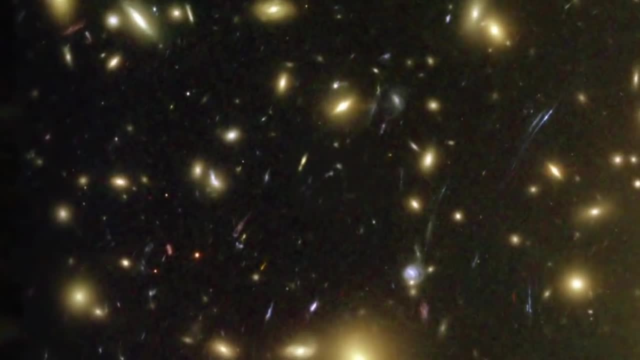 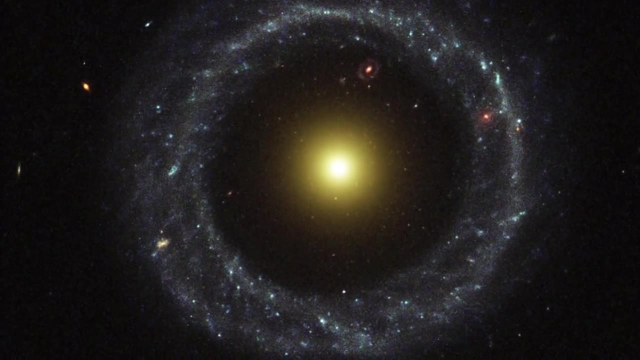 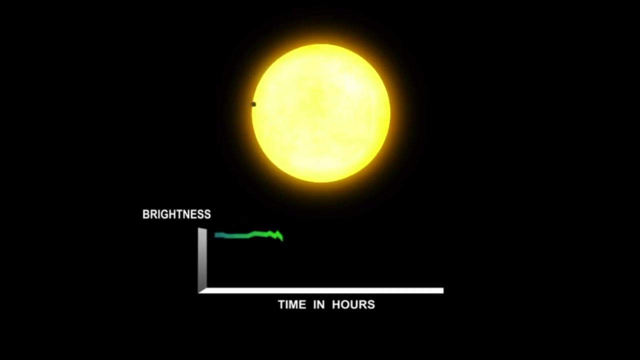 engineers Now to flip that around. what would you expect an altered galaxy to look like? Well, the classic one is: is that you imagine a civilization that wants to use starlight to power whatever endeavor it's up to? Dyson actually imagined just putting Earth around stars and just having Earth-like? 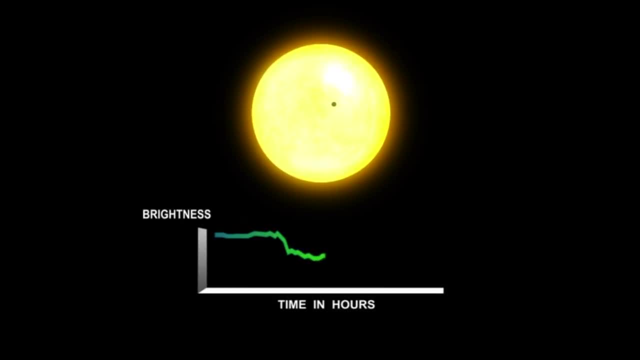 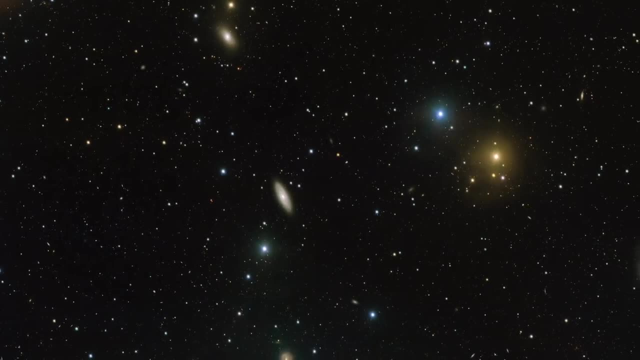 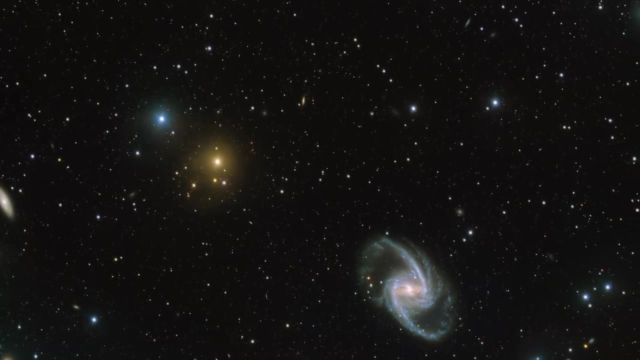 planets taking up most of the light from a star. You could do that over most of a galaxy and then you get a dim galaxy that had the normal mass and have a lot of waste heat coming out around 273 degrees. Wow, We don't see those. We've looked. Dyson Wright did this great search for dim galaxies. 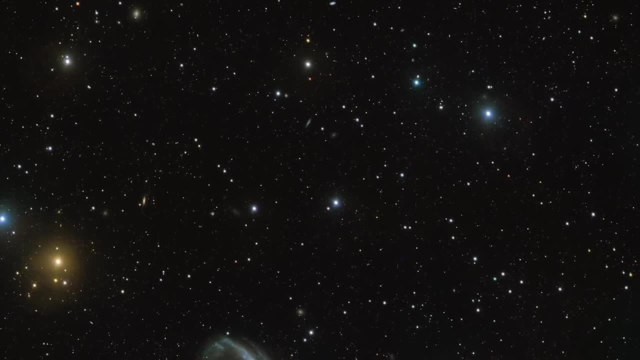 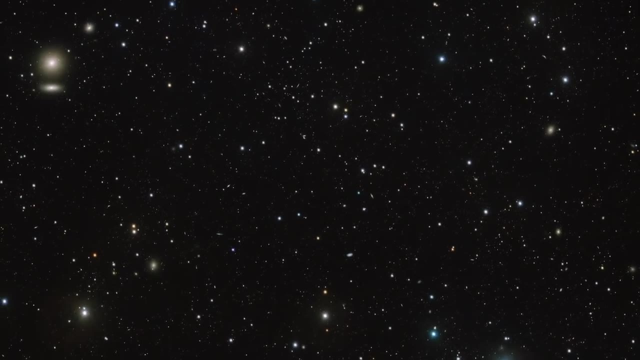 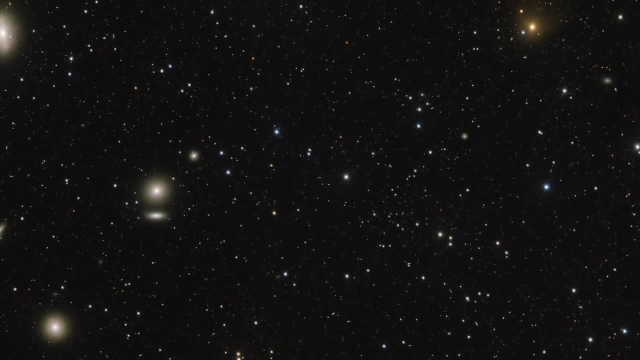 with waste heat, and didn't find a single one. Now is it possible, too, though, that there are certain types of galaxies that just would not be habitable. Is that an option That maybe perhaps a majority of galaxies just couldn't even have a civilization because of too much radiation or something along those? 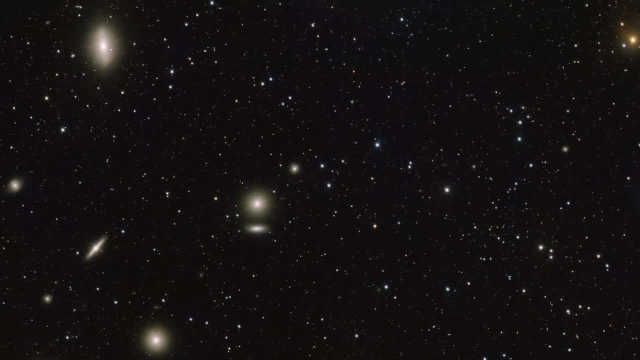 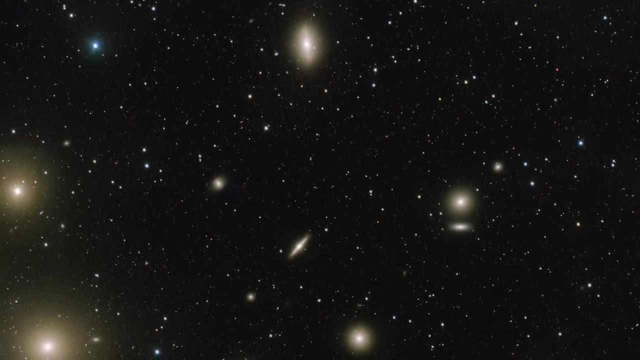 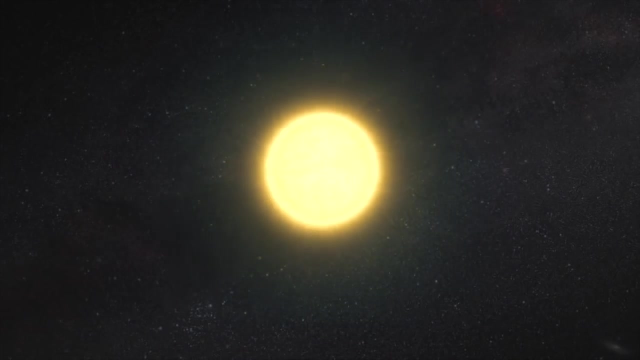 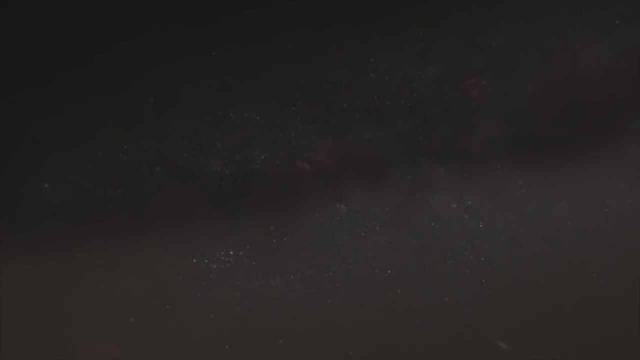 lines, Putting aside explosions for the second. It doesn't look to me like most galaxies are very different than our galaxy, And in our galaxy it looks to be a wide range of galactic centric radii are fine for habitable planets and therefore for life-bearing places. I sort of don't think that we are in a position. 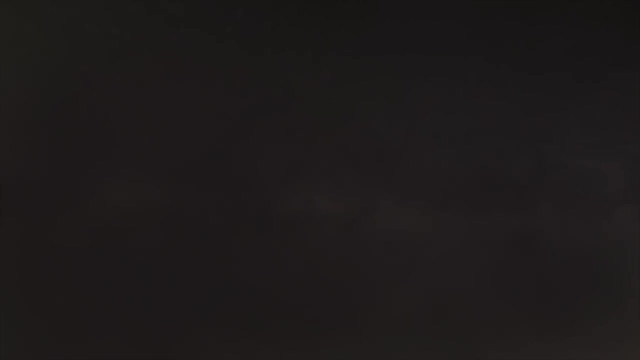 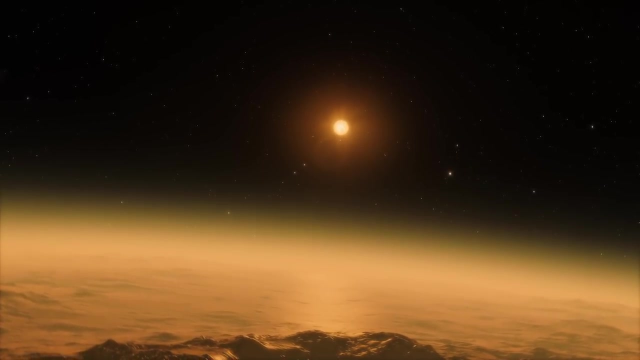 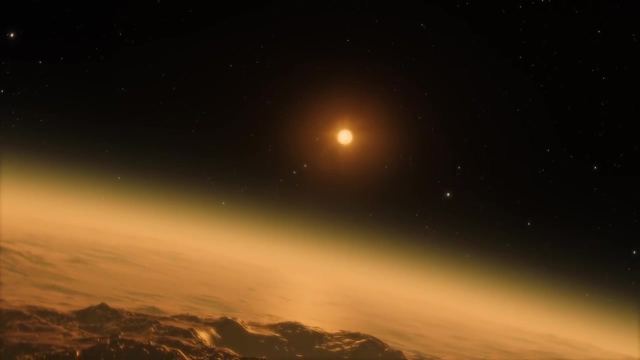 to rule out habitable planets in galaxies? Yeah, That's just a lack of imagination in my point of view. Now in your paper you go into the idea that maybe everything up until this point was simply getting sterilized, presumably by gamma ray bursts. Can you go into that? 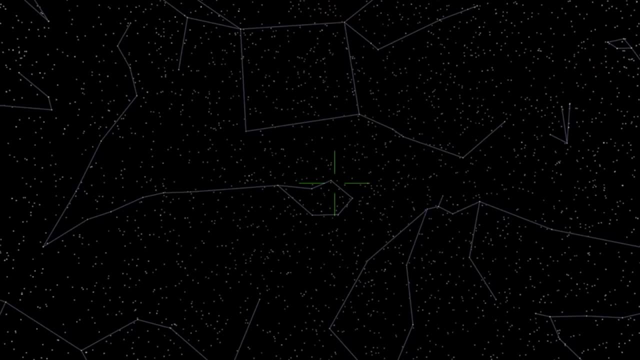 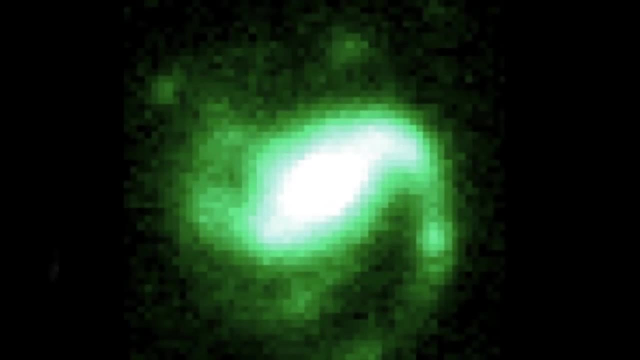 Sure, I'd be happy to. So we're back to this timescale issue. The galaxy is 10,000 million years old and it only takes 100 million years to basically fill it up if you're moving at anything like space-time. 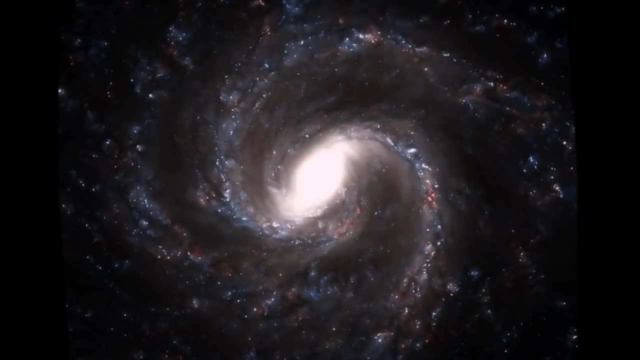 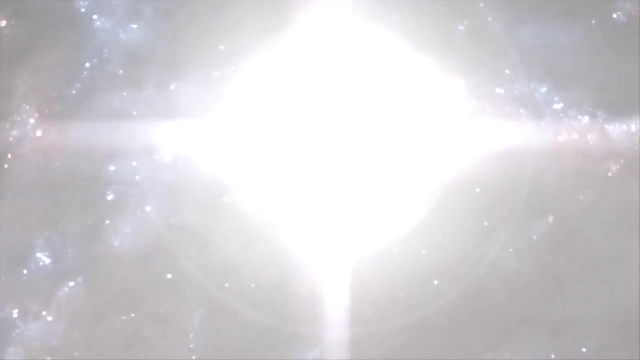 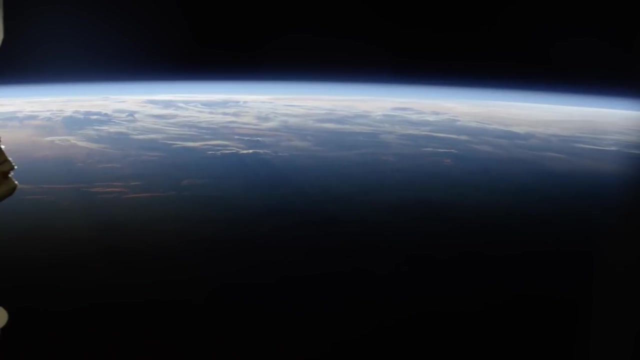 Yeah, And it takes velocities of 0.1 or 0.01 C. So that suggests that if life forms anywhere and that it's easy, therefore, to make intelligent life and space-faring life, then the galaxy should be full of space-faring civilizations. We don't see that, So you have a timescale. 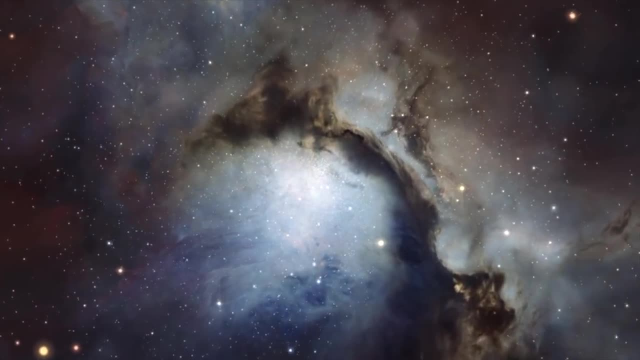 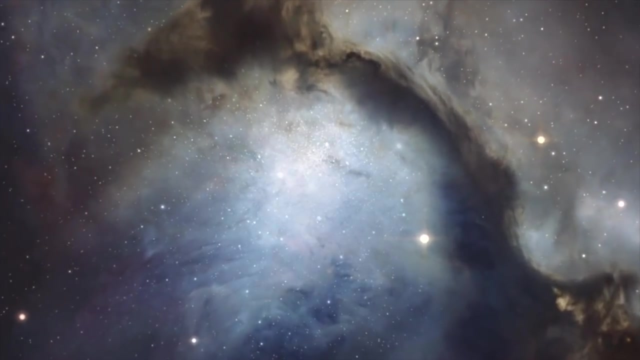 problem: How do you cut the timescales down? How do you cut 10,000 million years down to a couple hundred million years? Yeah, Yeah, A 1,000 million years, maybe a billion years, a thousand million years, And that is not. 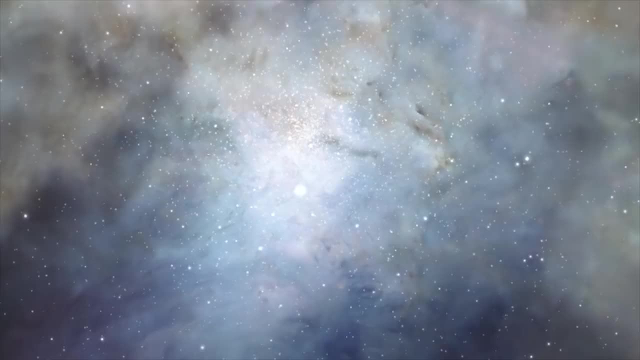 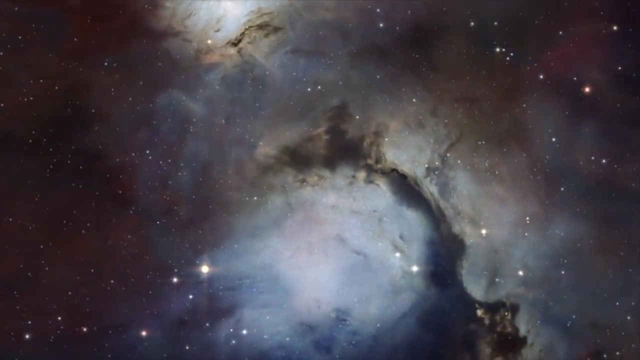 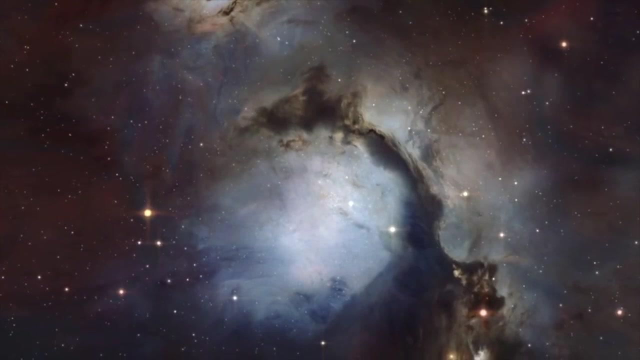 unreasonably done. You are getting at the idea of a galactic habitability zone. It has to do with the production of metal-rich stars. In my point of view, metal-rich stars form super early: in elliptical galaxies in the first billion years And the bulk of star formation universes in the first 2,000, 3,000. 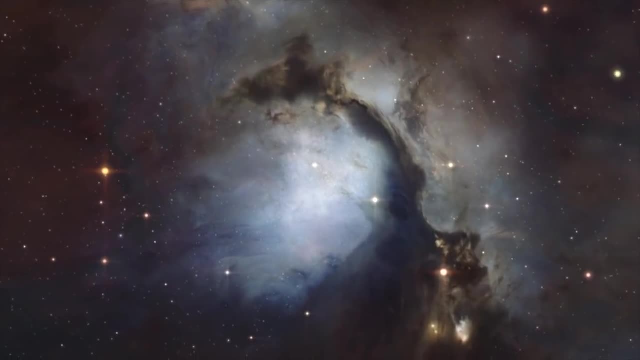 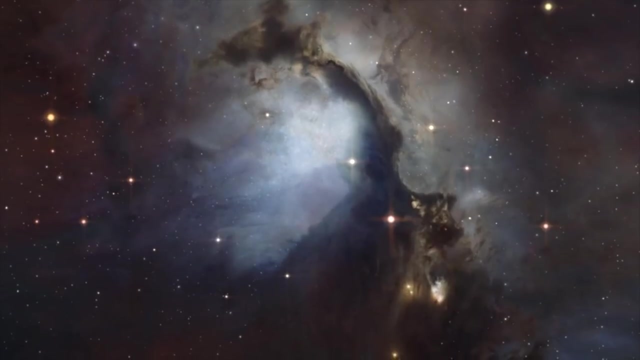 million years. So for life in galaxies it's going to be a thousand million years, but the total star formation for galaxies it's going to be 1,000 million years, But the total galaxy's universe is still 10,000 million years. so how do you, how do you cut that time, scale down? 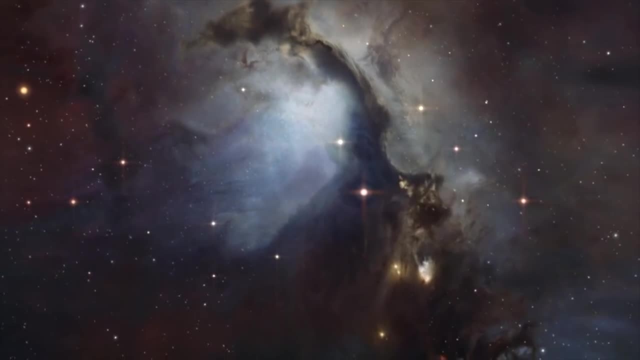 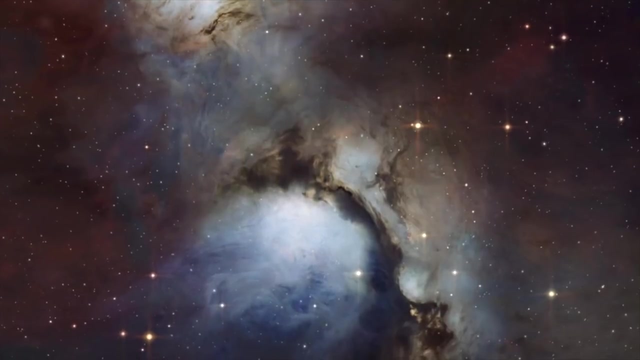 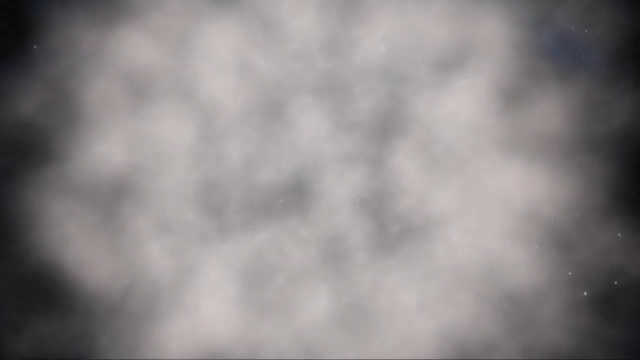 if you could cut that time, scale down, then you might have a solution to the great silence Fermi paradox. one approach is to imagine explosions. do it? supernova were thought of first. supernova is either where a star collapses, innards collapses to a neutron star or a black. 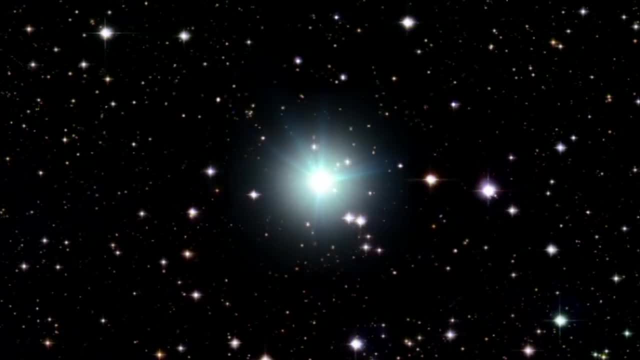 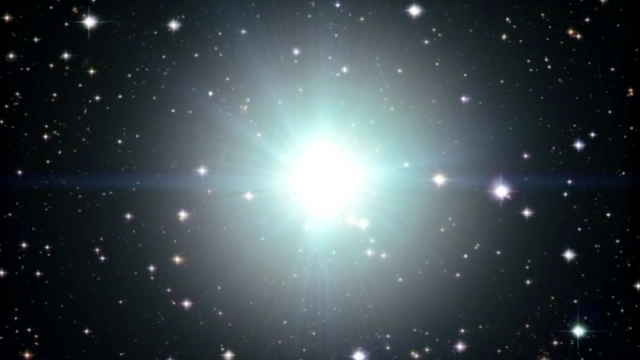 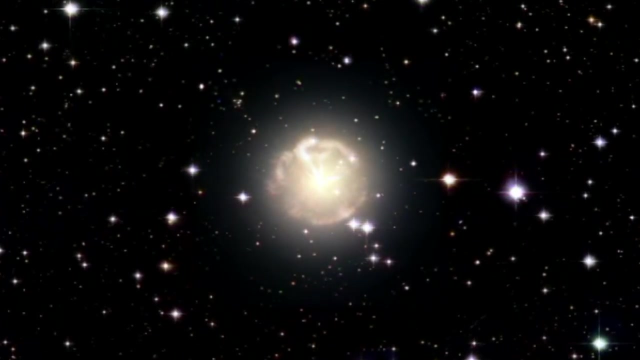 hole and the outskirts blow up, or this mass transfer from a star to a white door which then detonates. those aren't anywhere near powerful enough to affect anything more than a local regime, a few hundred light years at most. but gamma ray bursts, gamma ray bursts can do it. 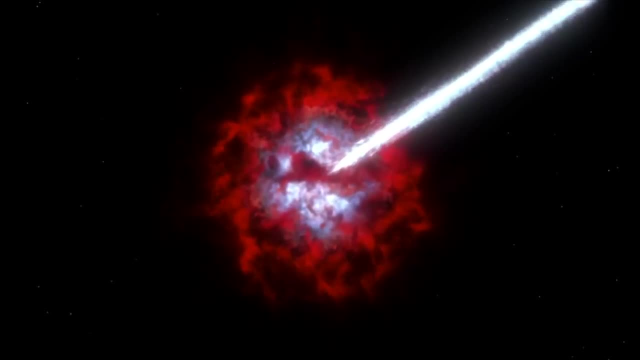 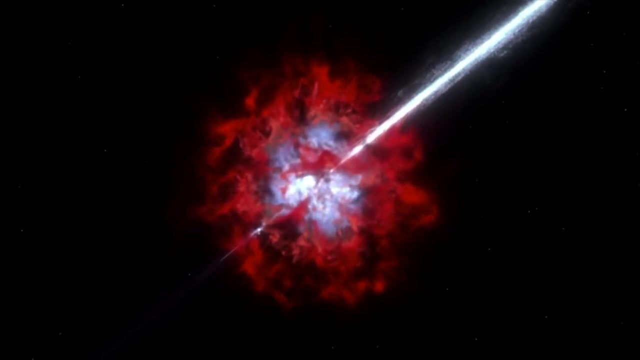 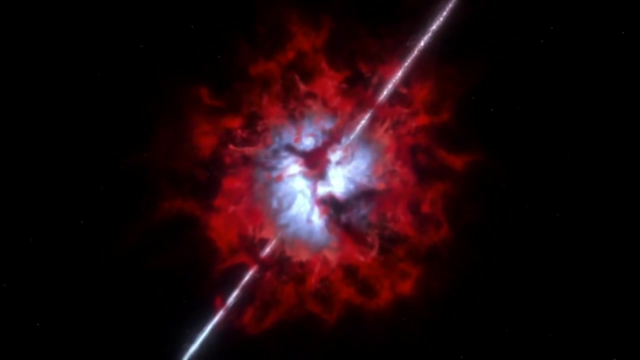 gamma ray bursts are as energetic as supernovae, but they don't produce the energy in neutrinos like supernovae do. they produce the energy as a beam jet. a beam jet of energy has lots of features to it, not least which is a long-term travel. a high energy density. high energy density jet could be considered a. 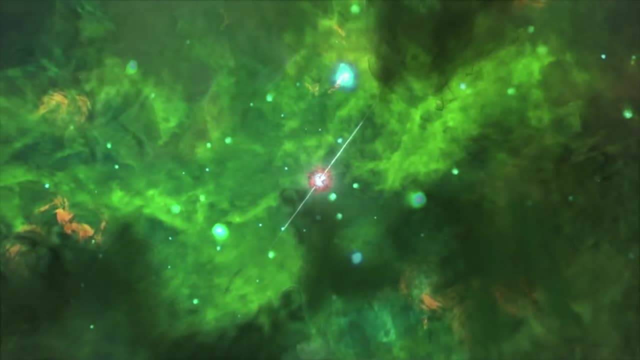 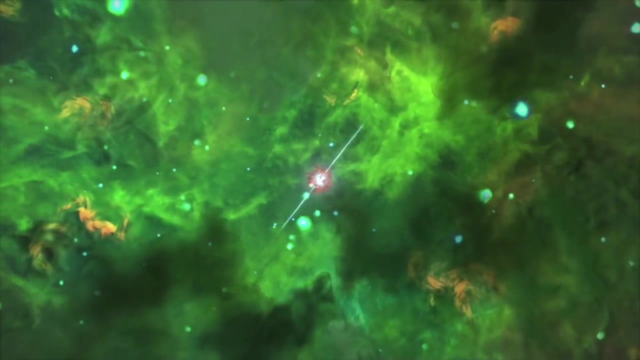 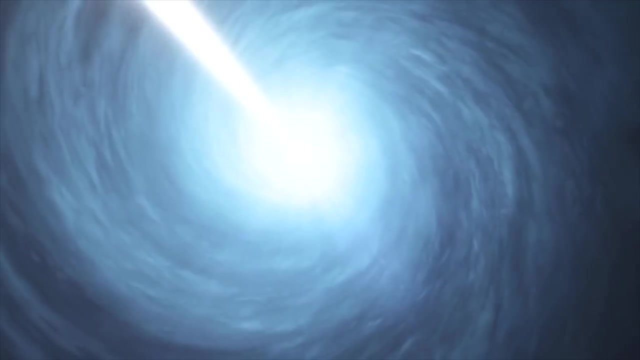 weapon- in fact you could consider a weapon- to wipe out life in star systems across tens of thousands of light years. ten to thousands of light years is a galaxy scale now. so if you imagine gamma ray bursts can sterilize planets, that's a big. if we have to come back to that, 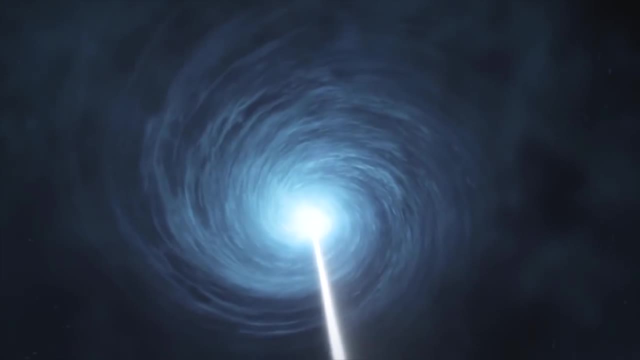 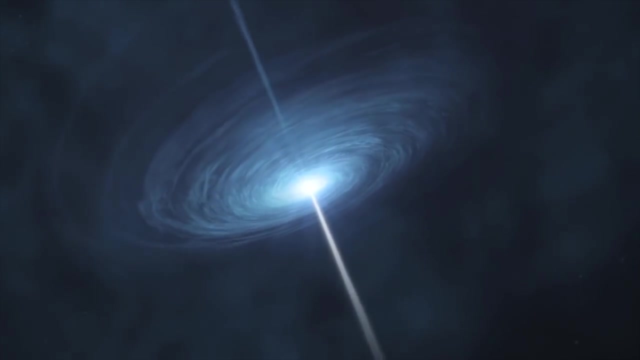 then you must start talking about: well, do they happen? how often do they happen? if they're once per galaxy per 10 000 million years, that's not sufficient, that's too rare, but it turns out that almost every scenario for a gamma ray burst. usually the trucks aren't not even near level, since it's still active, but it's not easy to keep up with the. but it turns out that almost every scenario for a gamma ray burst, usually the things you're really trying to do are scaling up and it's only a tiny, small step away. but it's actually the jamais Теперь. he's struggling to do it to some extent. 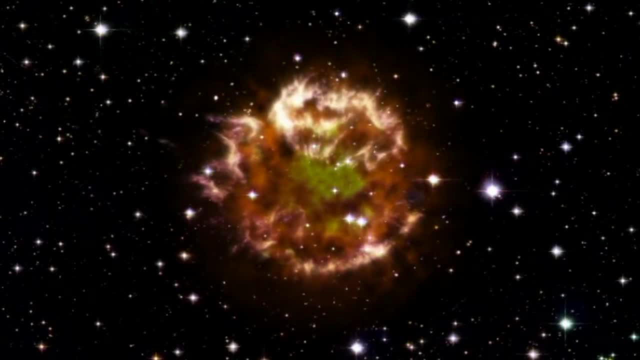 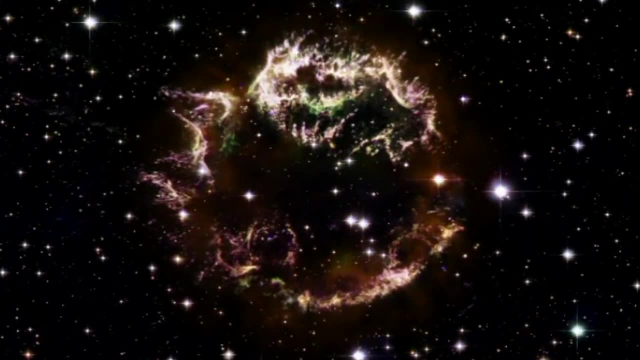 it's very hard to do it just once. every single step is difficult and it's pretty hard when you're going around the world. you're creating extra difficulty and it's impossible to keep up with it. they're young stars. Current scenarios involve young stars: magnetars. 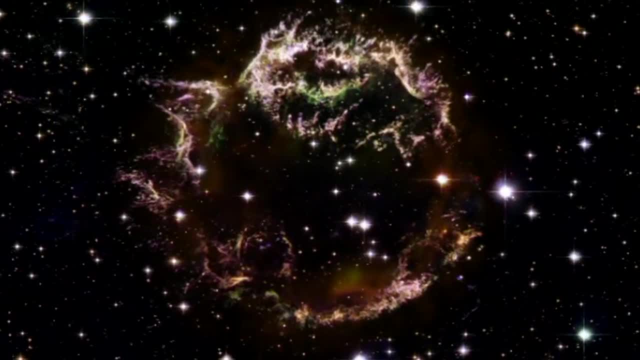 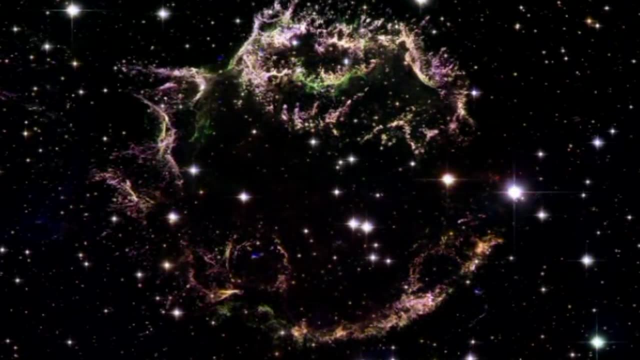 Follow the star formation history of the universe. The star formation history of the universe was mapped out about 20 years ago and it's known that most stars were formed in the universe in about 2,000, 3,000 giga years. There's an echo effect. there may be delay time between when the stars were formed and a gamma-ray burst forms. The short gamma-ray bursts are almost certainly neutron star mergers. almost certainly in all cases They may have a few hundred, a few thousand million year delay time. 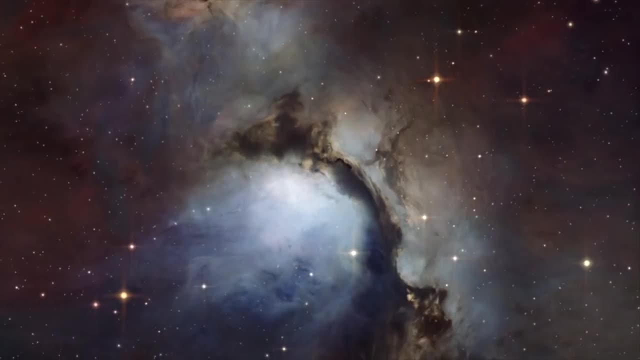 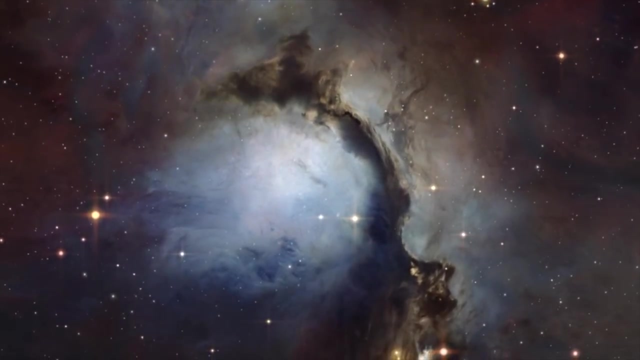 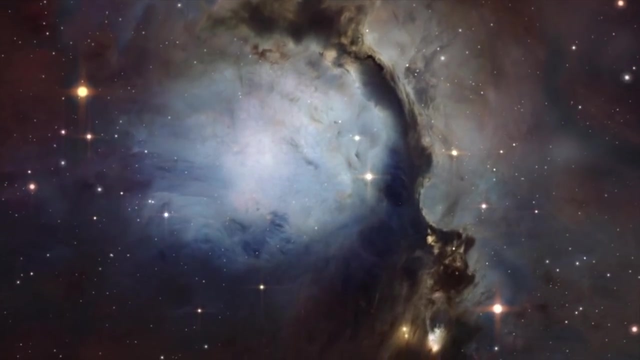 but the long gamma-ray bursts, the ones we're really talking about, almost certainly follow the star formation history. Now our galaxy's still forming stars at about one solar mass per year, so star formation's still ongoing. it's just a lot lower than it was 10,000 million years ago. 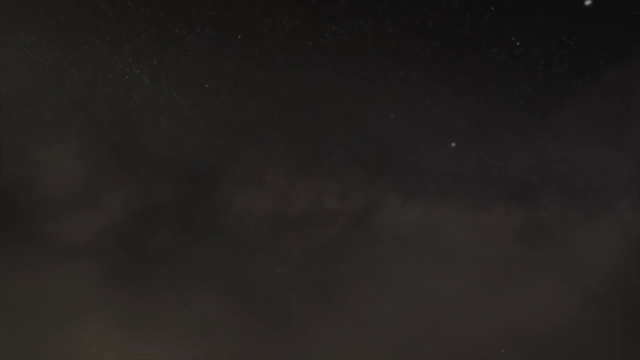 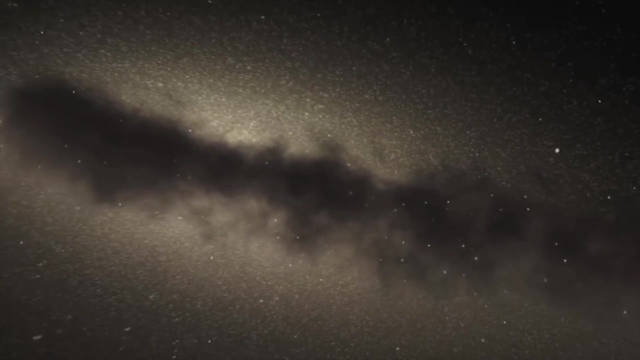 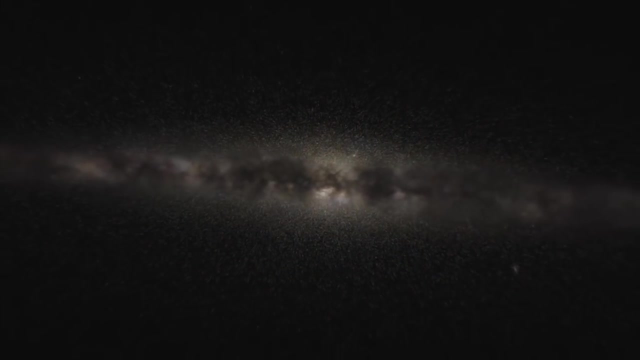 If gamma-ray bursts follow that they were much more common in the early universe and much less common recently. One reasonable model gives a rate of about one per galaxy per 100 million years. Now, that's the right time scale. Now we're talking. 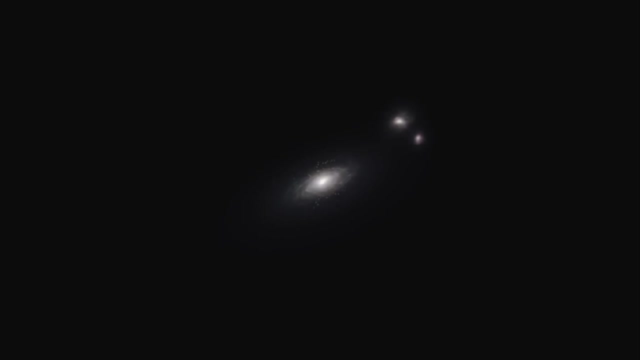 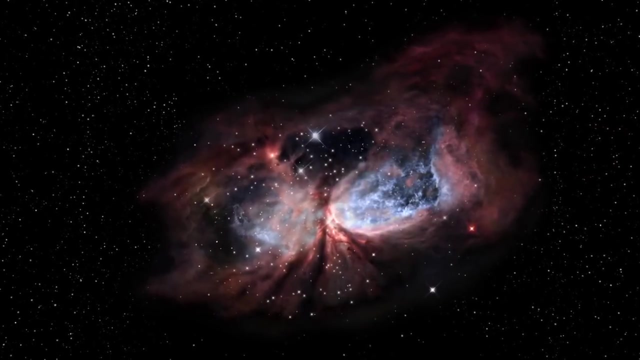 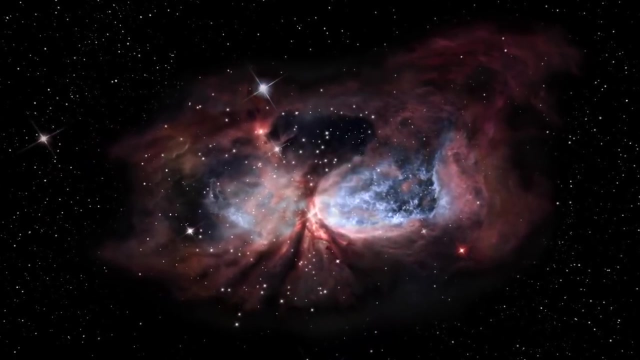 If gamma-ray bursts can sterilize large sections the galaxy once every 100 million years, then you have a way to cut the time span down. Instead of 10,000 million years to fill a galaxy, you might have 100 million years to fill a galaxy. 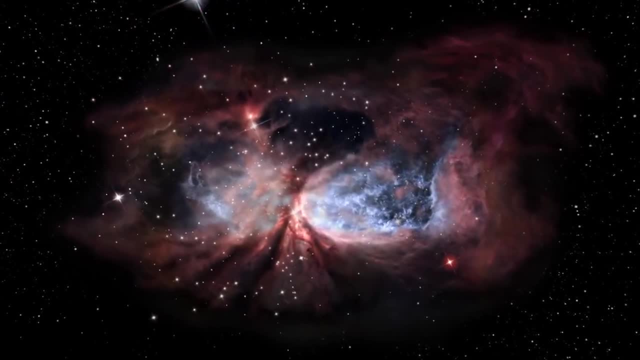 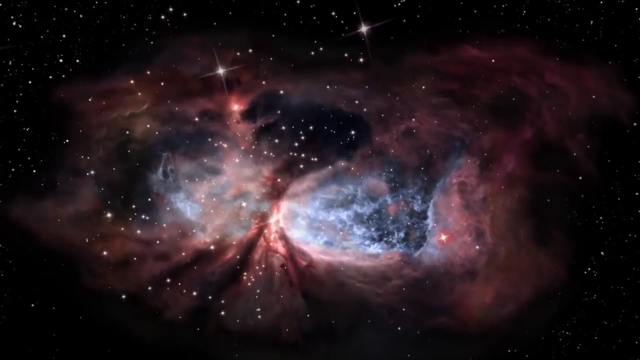 Then it's dicey if any galaxy will have a reasonable galactic-spanning life, space-faring life. That's the heart of this. We need to talk about where the gamma-ray bursts can actually do this. But in my mind, 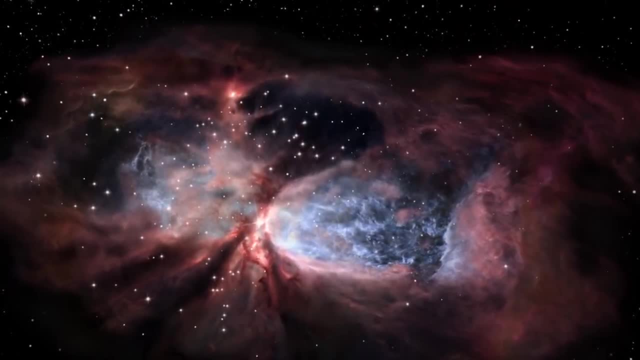 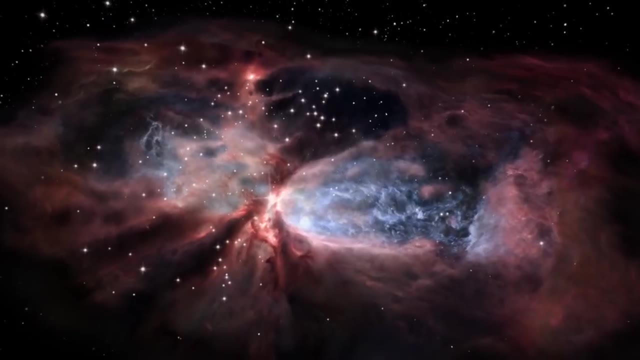 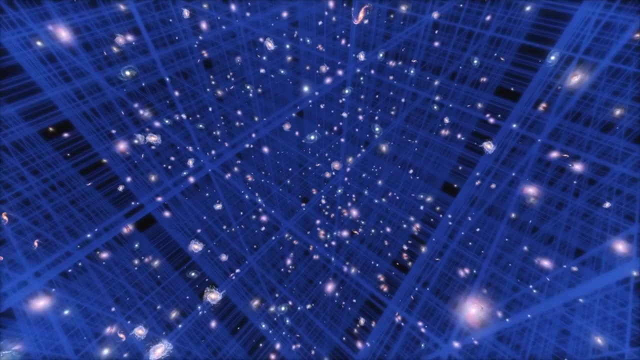 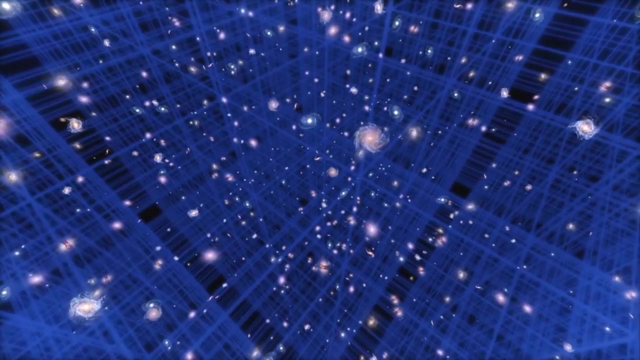 this is like another scientific endeavor in which there is a great scenario without a good mechanism. That's inflation. Inflation's this thing that happens in the early universe, where soon, actually well before the formation of elements, the universe expands at greater than light speed. 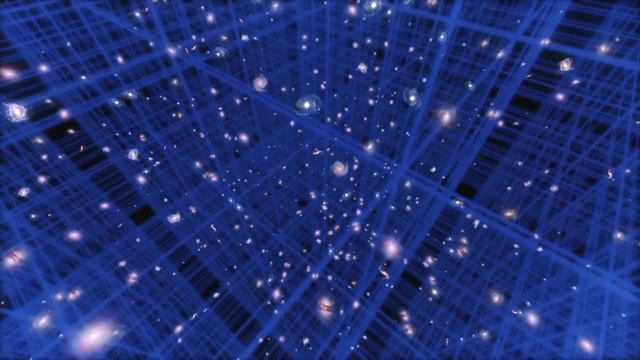 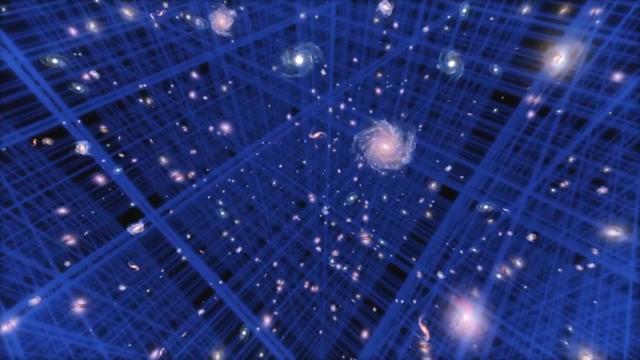 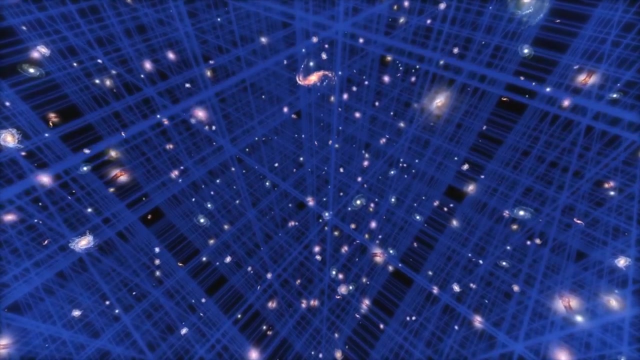 and quantum fluctuations are blown up into large-scale structure in our universe. That solves the geometry of the universe. It makes it nice and Euclidean flat. It solves homogeneity of the universe. Why is it the same in every direction? as we look isotropic in the universe? 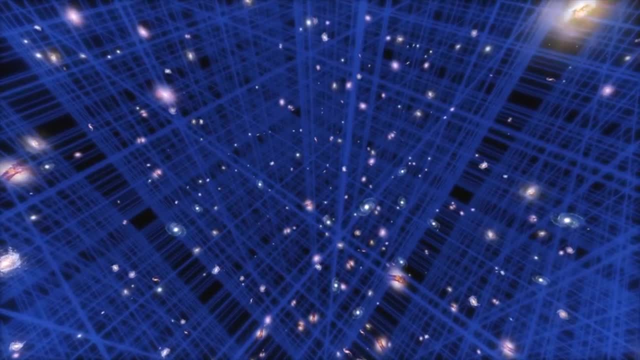 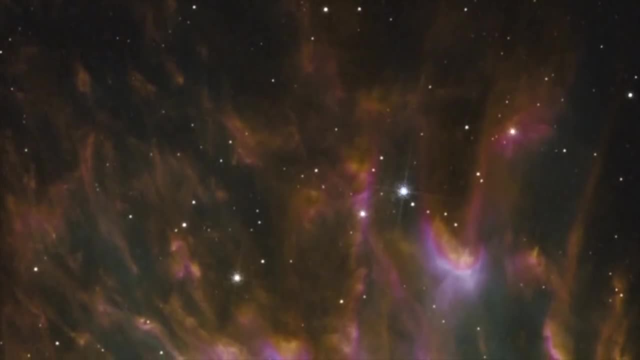 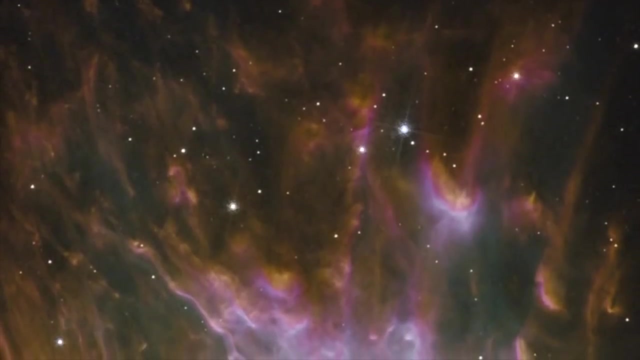 And it's a standard feature of modern cosmology, but there's no known mechanism to cause it. There's no known particle or field that causes inflation. It's a scenario looking for a mechanism And, in my mind, this astrobiological phase transition model. 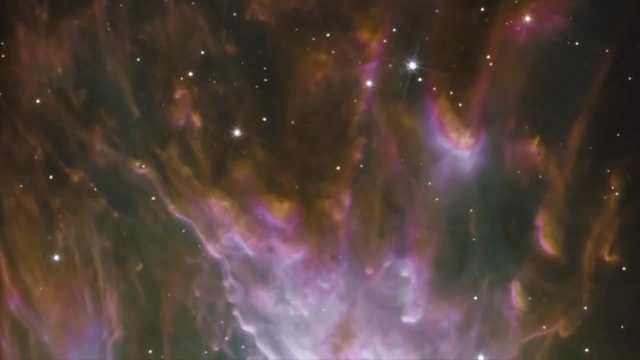 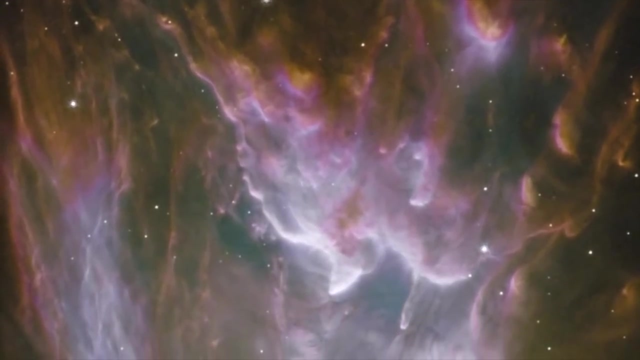 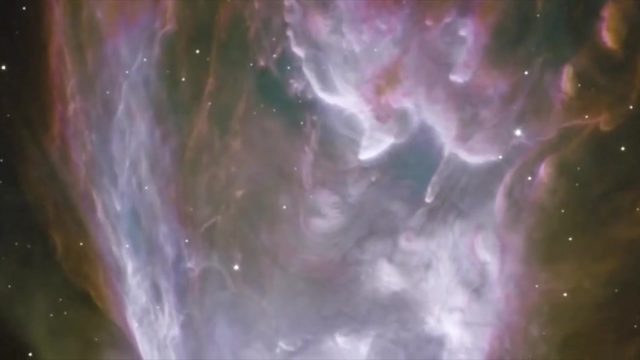 that we're talking about is rather like that: If there is a mechanism to suppress the formation of space-faring civilizations until that slowly decays the universe so that the mean time between suppressions after eons becomes long compared to how long it takes for life, 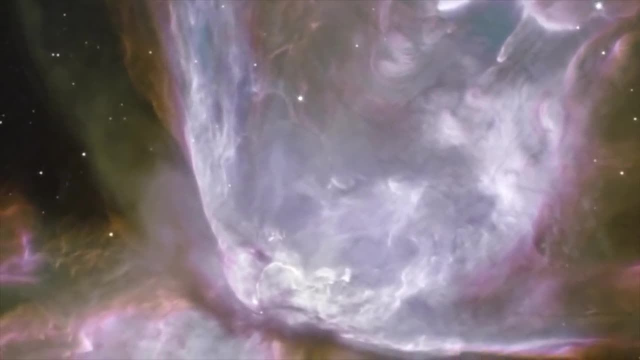 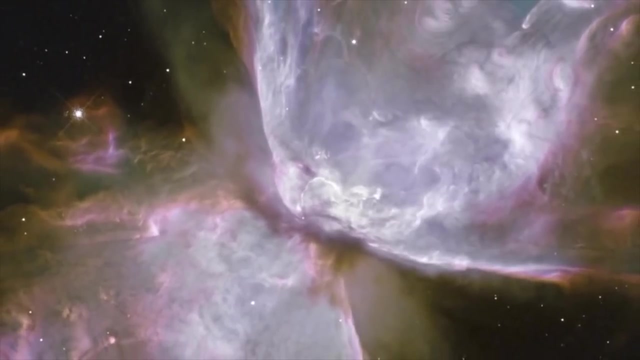 to become complex enough to form intelligent life and then to form a space-faring life. then you have a mechanism to explain the great silence, And gamma-ray bursts are the leading idea for it, but they're not a very successful idea for it. 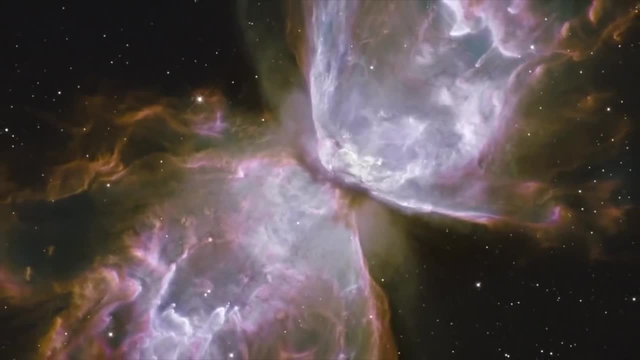 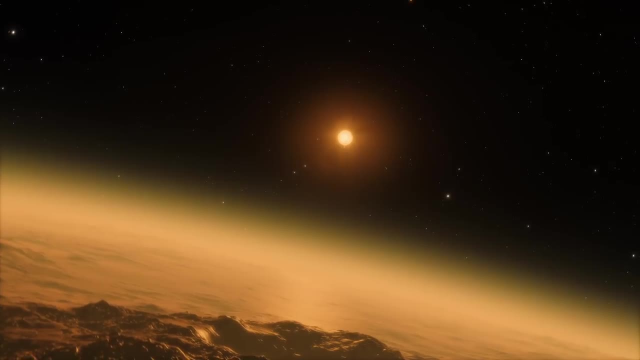 It'd be great. they're very energetic, they're very nice, but in detail it doesn't quite work. and we can go into that Now. before we do that, this idea of sterilizing a planet now could a gamma-ray burst if sufficiently close. actually sterilize a planet, or is this more of a question of atmosphere? You're destroying an ozone layer, like with Earth, or something like that. What is the way that the gamma-ray burst would actually cause an extinction? The easiest way is to knock out the ozone layer. 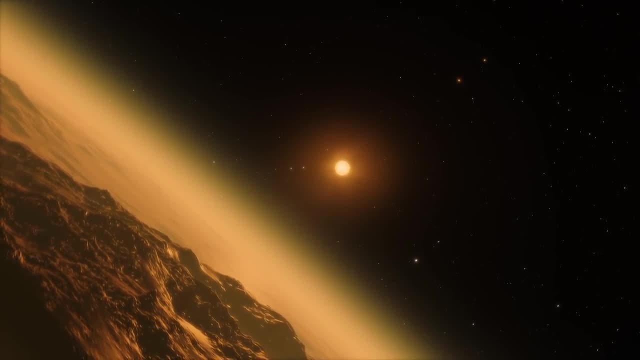 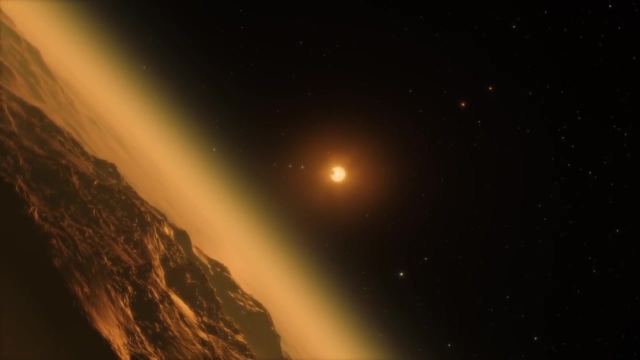 and then you get UV photons and you let the UV photons from the sun actually just kill off life on the surface. That wouldn't kill sea-based light, but it would certainly kill anything that was in the photon field from a G star. 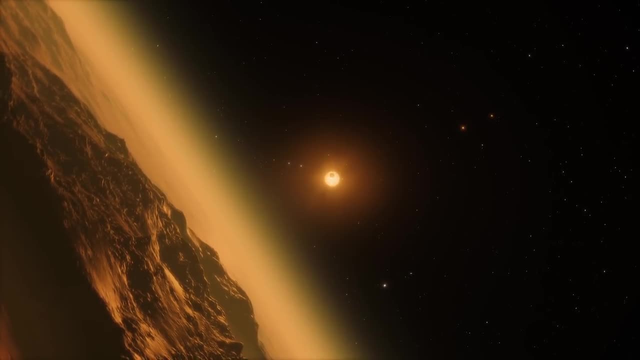 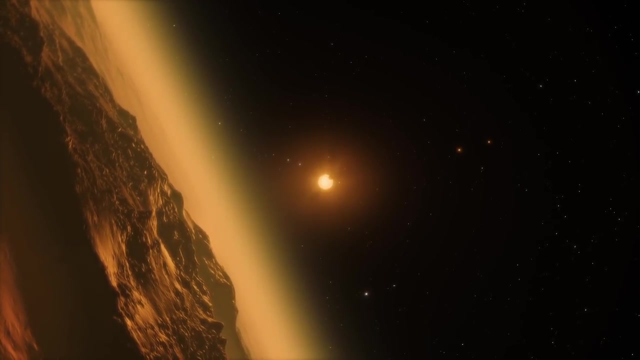 So stars like ours would kill off life? It may not be true for the redder stars, the cooler stars. they may not have enough UV photons to actually do that. A secondary way is to produce is the jets themselves, the gamma-ray burst jets. 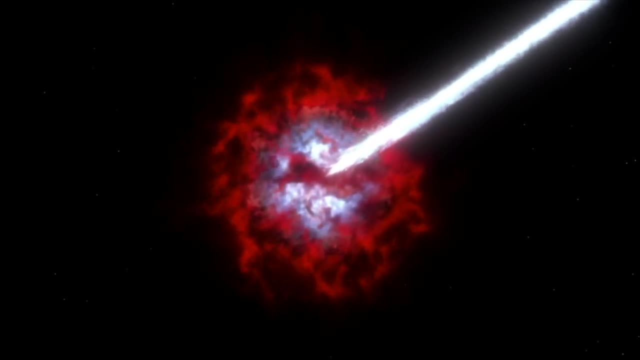 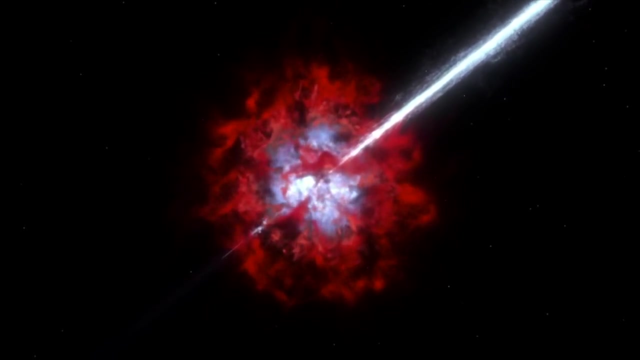 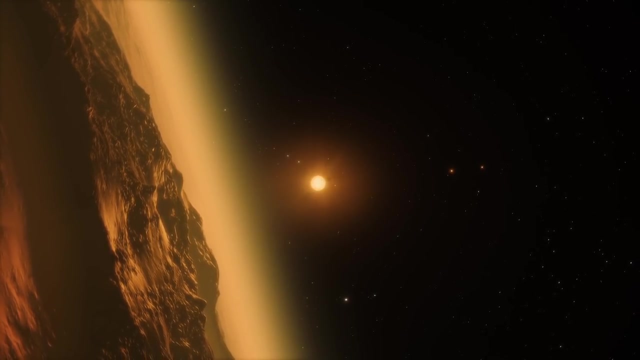 have enough energetic particles to cause a muon cascade in the atmosphere and the muons can cause lethal damage. That's less likely. So does it really? is it really sterilizing? No, it just doesn't. Maybe the muon flux would. 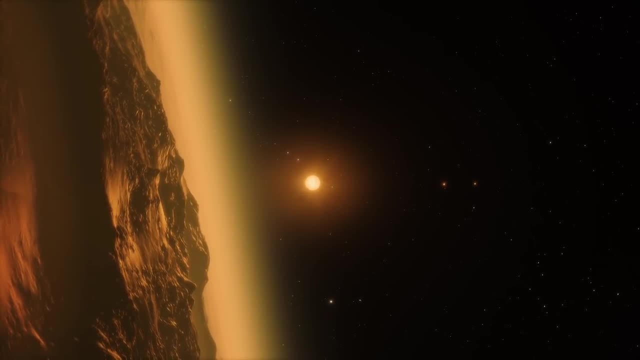 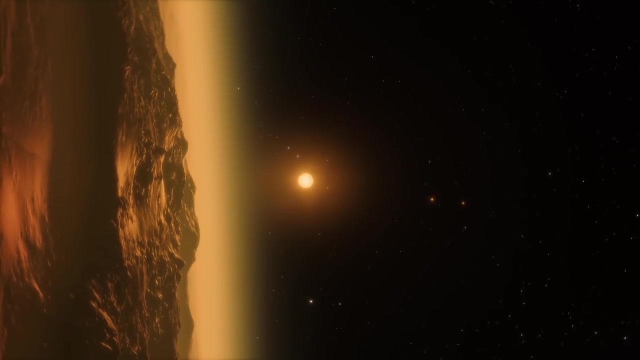 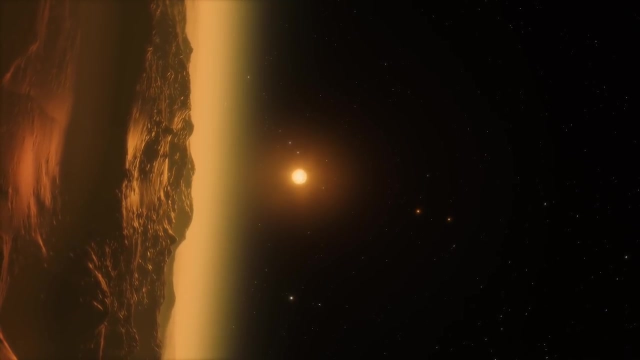 but the muon. the idea that gamma-ray burst jets can cause a muon shower in the atmosphere relies on closer proximity to the gamma-ray burst than gamma-ray burst jets knocking out the ozone layer. It's a little bit less like it. Just turning off the UV flux, letting allowing the UV flux from the sun to hit our ecosystem. we'd have disastrous consequences for animals on the surface, probably maybe for the shallows in the ocean, but that would do nothing to the deep sea vents. 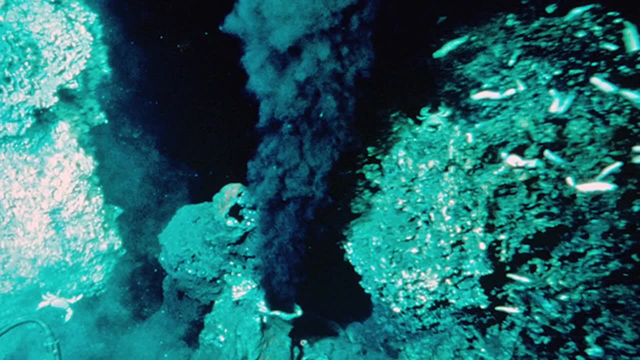 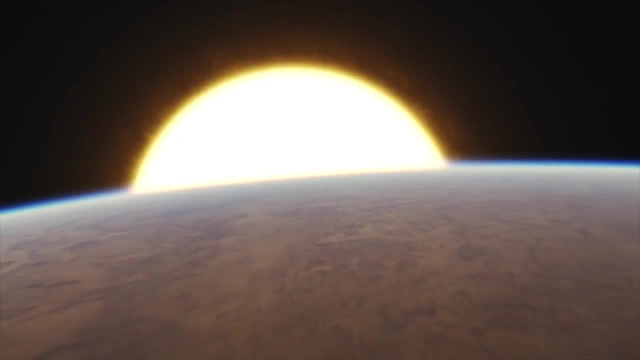 for example. So sterilizing is the wrong word. That's interesting, because then say the people that are looking at exoplanets and say, you know, as we move further with better equipment like the James Webb telescope and such, 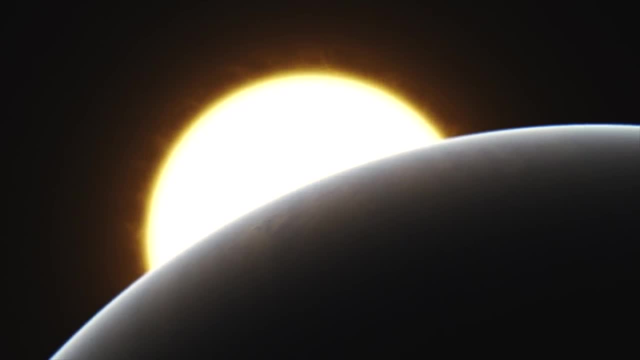 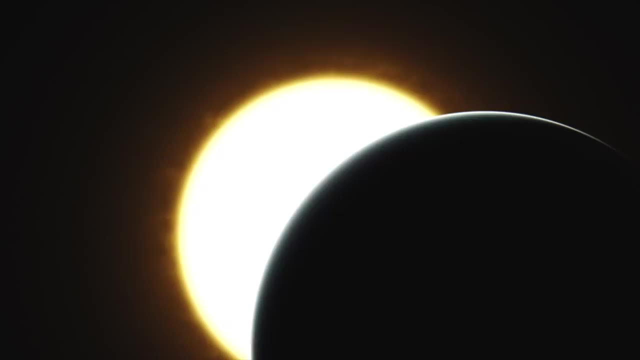 and we can start trying to characterize these worlds. wouldn't it make more sense to you know, to look at worlds that have a lot of liquid water, An ocean, meaning that there's more survivability for life on a planet with a lot of ocean, space? 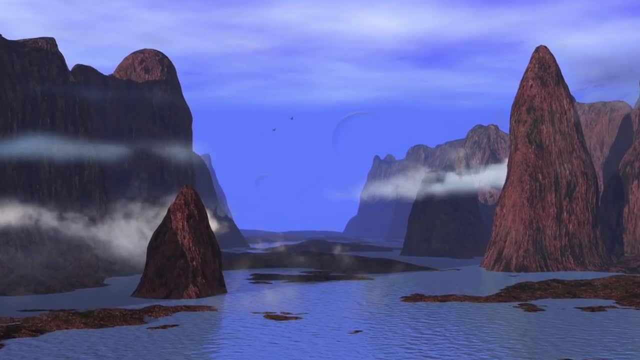 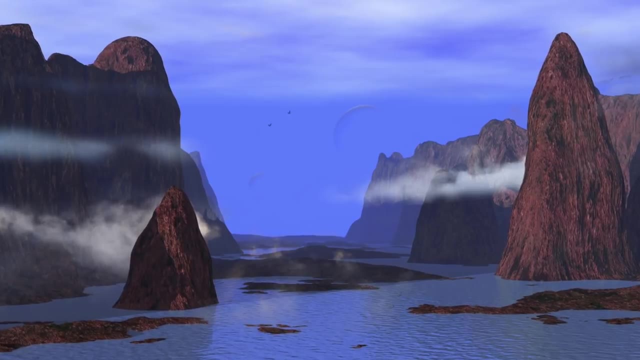 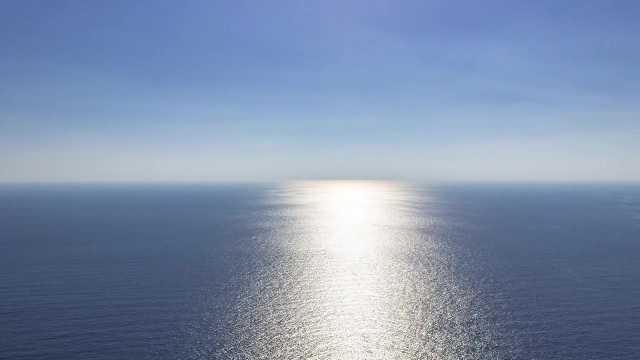 as opposed to say just a lot of land masses. Wouldn't it make sense to look at that, because those planets would be favored to have life that survived the gamma-ray bursts? Yes, but there's lots of reasons to favor ocean worlds. 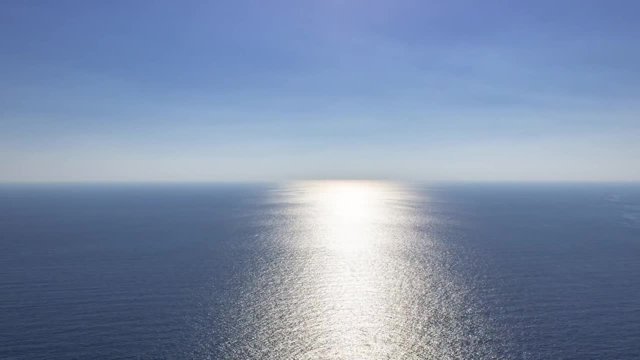 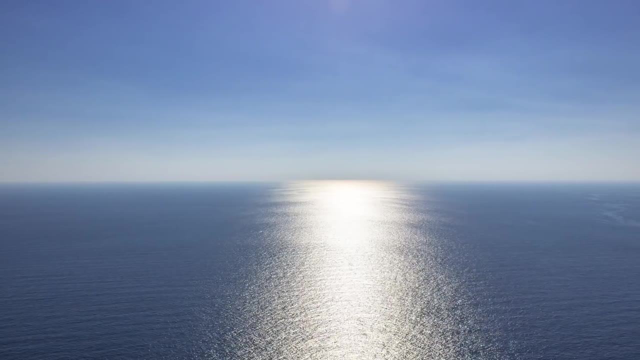 Water is great for life. I mean you don't need to reach for gamma-ray bursts being a problem for ground-based life. So back to deep sea vents. Deep sea vents are great, right. I mean they're warm, they're nutrient-rich. 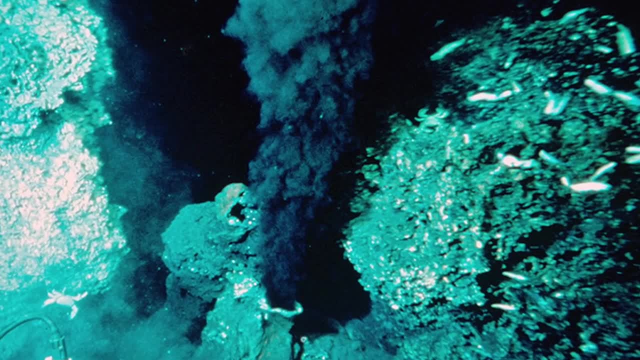 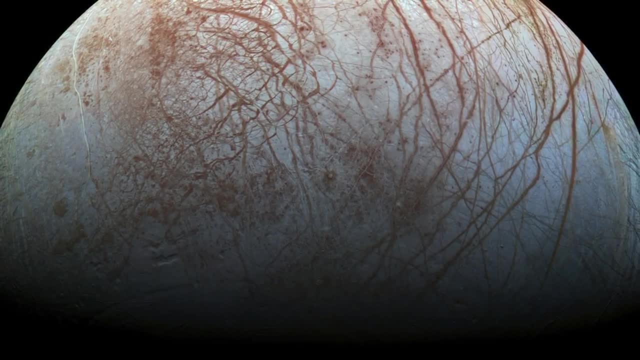 and life likes them on the Earth. The odds of them being on Enceladus or Europa are really high. I mean, that's the most likely scenario for life on those two moons. There's lots of reasons, Right, There's lots of reasons. 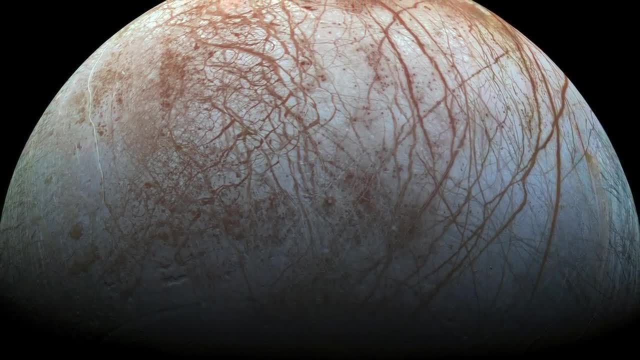 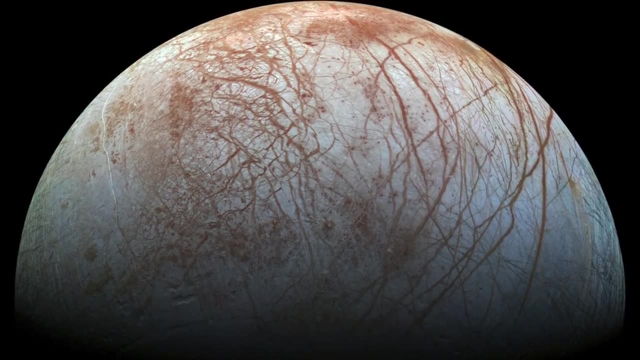 There's lots of reasons to look for icy planet or for ocean-bearing planets. Now, that's interesting. If you have that scenario: ice shell worlds like Europa and Enceladus. they would be impervious to gamma-ray bursts, wouldn't they? 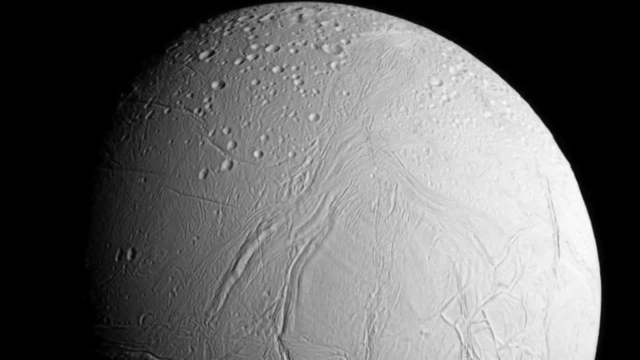 I mean getting through that ice. they would just see no effect at all. right? Well, there's no ozone layer to knock out, for example. Yeah, nothing. The muon shower could probably do it, but it depends on details. 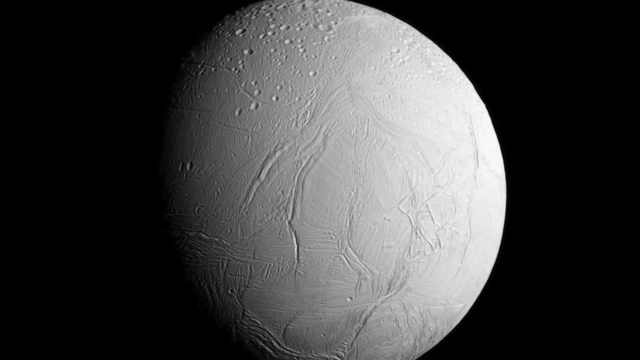 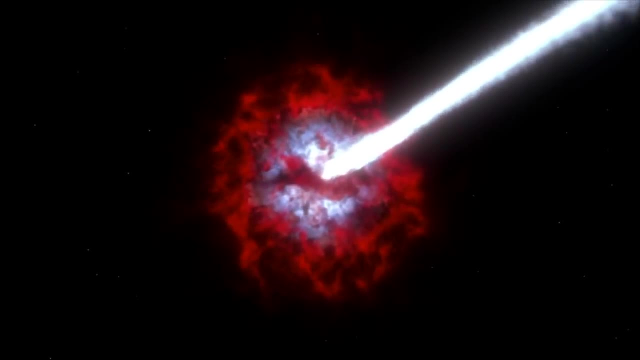 What I can't report on is the detailed structure, the structure of a jet from a gamma-ray burst, what kind of particle flux it produces, and whether that would cause a muon shower in the atmosphere or on the ice world. We just don't understand those jets well enough yet. 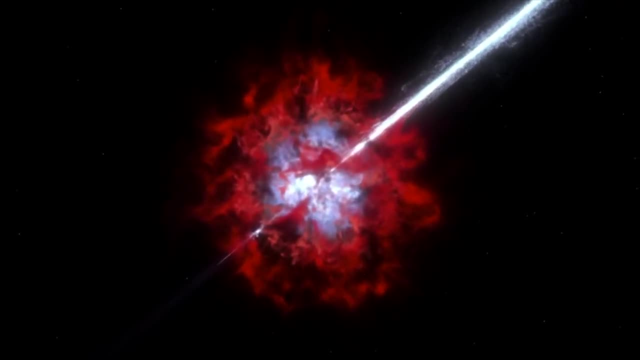 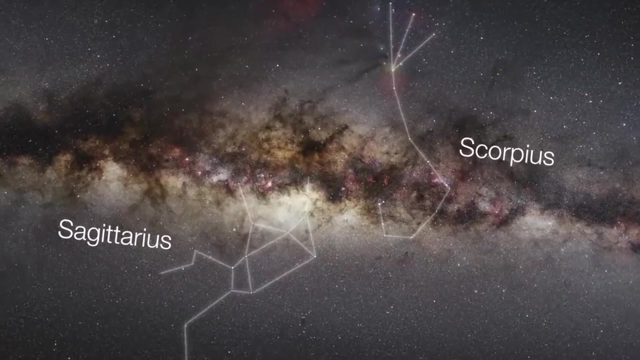 Now this all leads to an explosion of intelligence in the future, starting effectively now. So we could end up with a universe that the older it gets, the more intelligent it gets as far as civilization is spanning it. So is there anything that you can think of? 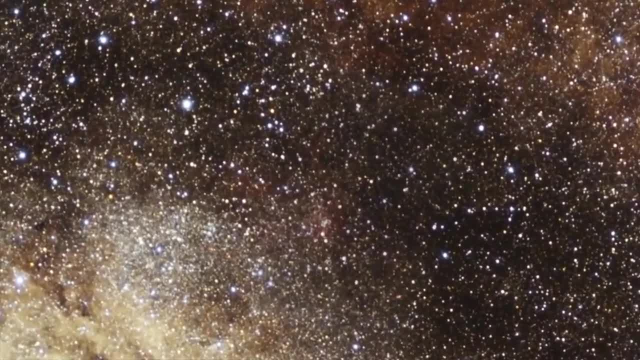 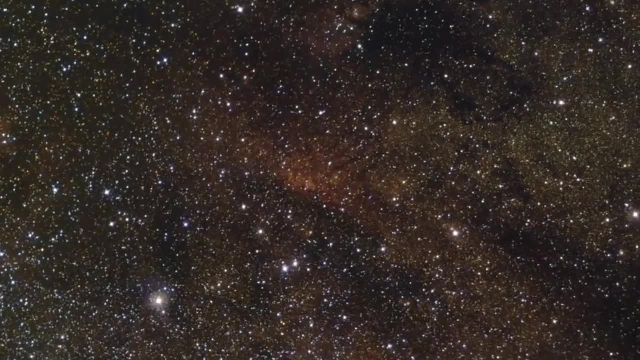 that would get in the way of that, meaning that are the gamma-ray bursts just gonna continue to get more and more sparse, or at least the type we're talking about, the longer gamma-ray bursts. Gamma-ray bursts are getting rare and they're becoming less luminous. 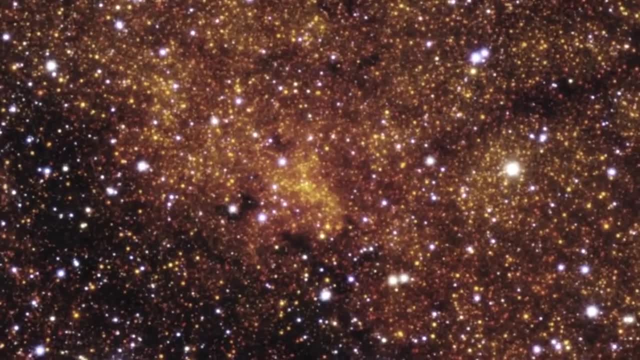 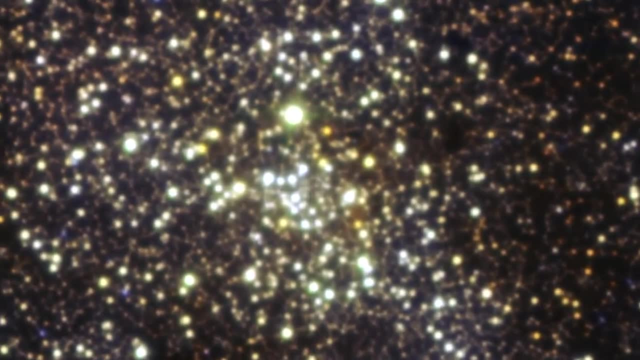 Everything about them goes in the right direction. So, if they are the suppression field, if they're, is what are? So in my mental model of this, they're not really sterilizing planets. Gamma-ray bursts are really good at killing off ground-based life. 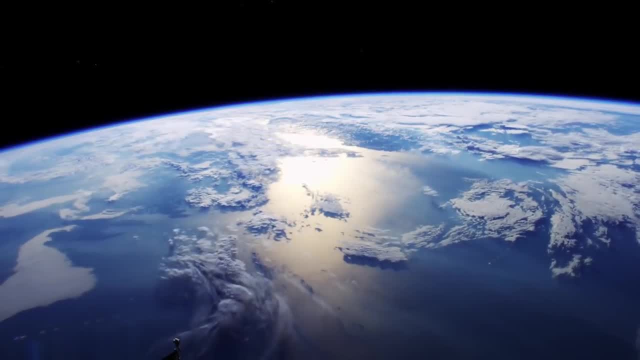 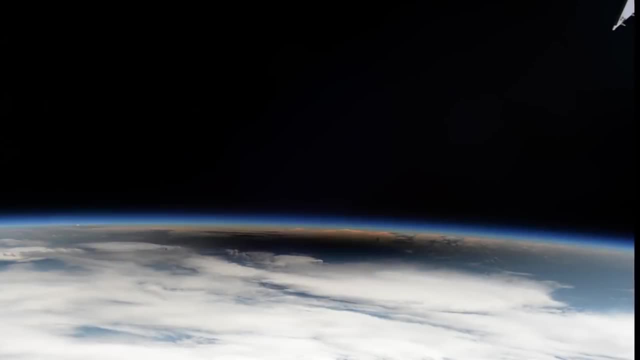 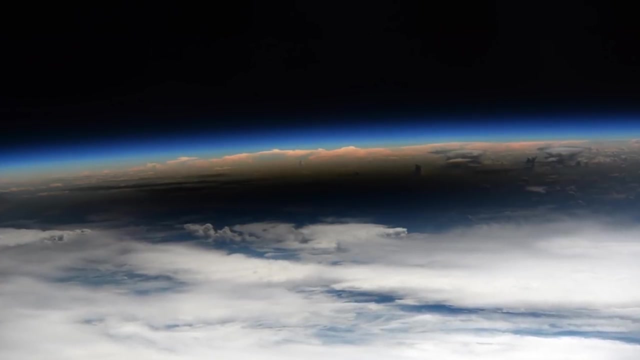 Not so great at killing off ocean-based life, And so in Earth's history, it's common for animals to migrate, species by species, from the water, from the ocean to land, back to the ocean and back to the land. Species just do that over tens of millions of years. 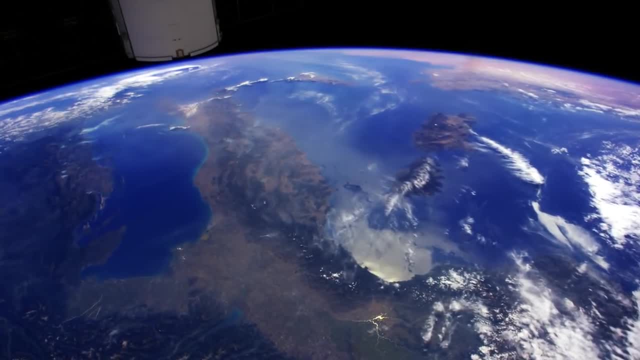 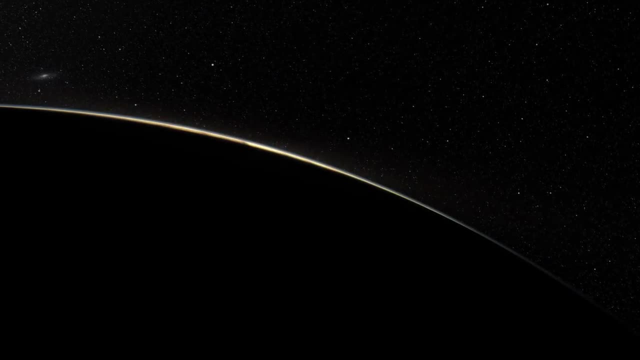 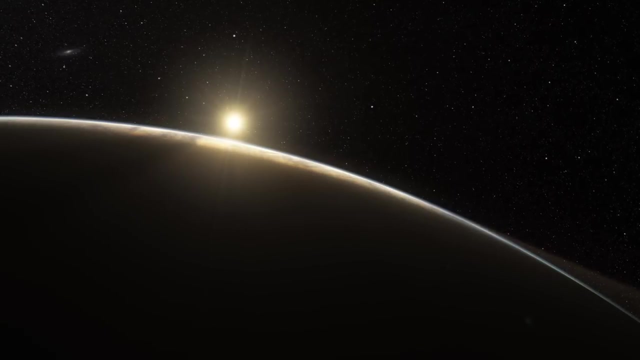 It seems to me that a gamma-ray burst in Earth's prior history would be a mass extinction and the Earth's ground-based stuff would just be repopulated from the oceans. So the fact that they're becoming more rare and less powerful just suggests that the ecosystems on the land, have enough time to grow, fill the niches, explore the more outlandish body plans, find out new things that work as life does in the general ecological and evolutionary system. So it's pretty clear, looking at life on Earth, that it's getting more and more complicated. 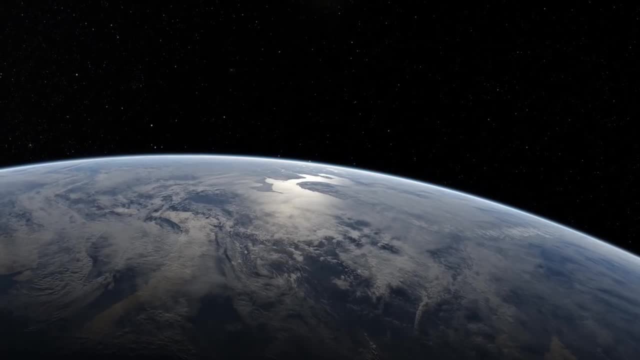 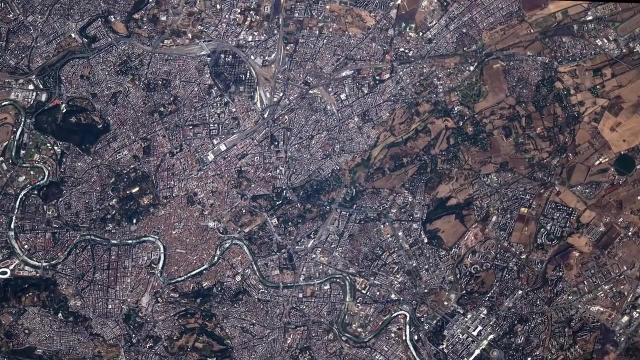 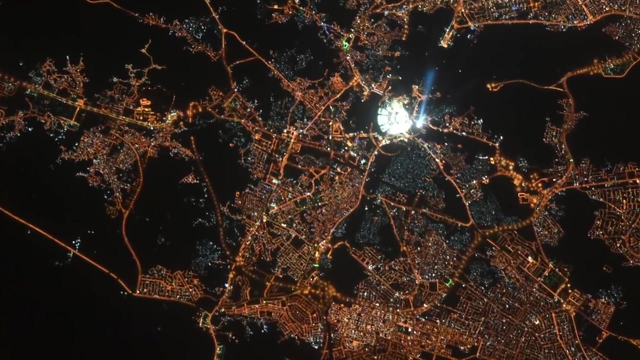 So you have to avoid the idea of progress or better. But being complicated isn't necessarily better. It looks like life on Earth is getting more and more complicated, You know, from one cell to multi-celled, from sponges to plants, to animals. 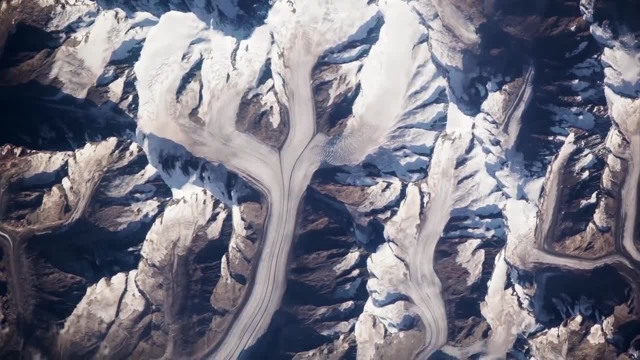 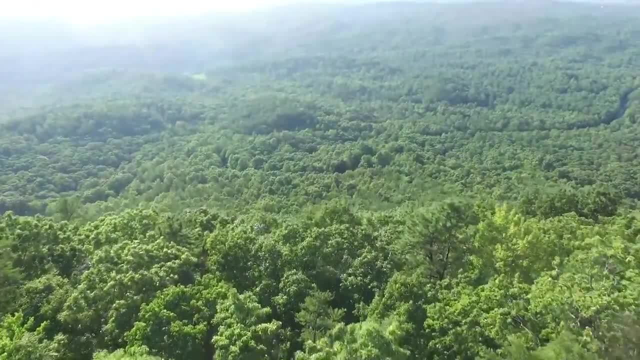 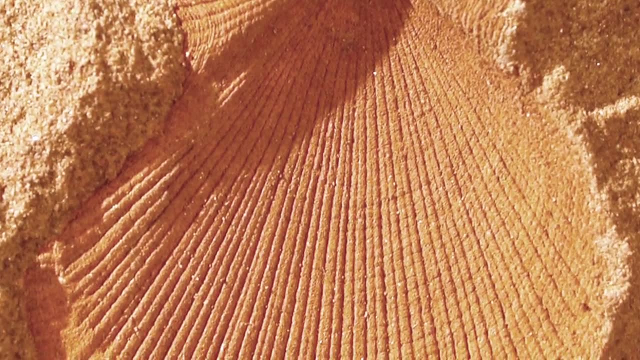 and larger organisms, And so one can go back to the fossil record and look at the sizes of the largest animals in the given epoch and geological time, And it turns out the largest one is the blue whale. I mean, it's alive now. 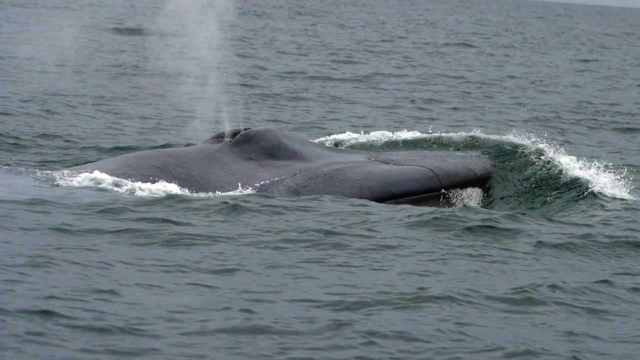 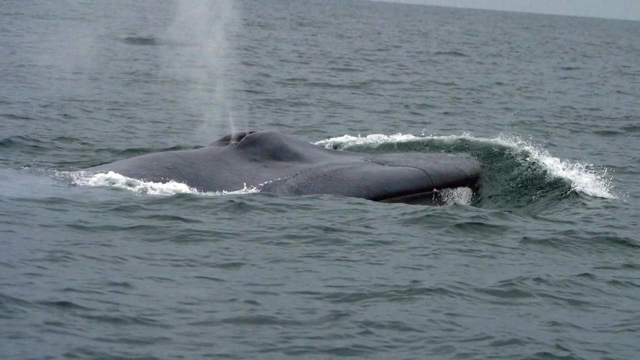 It's a mammal, It wasn't a dinosaur And certainly it wasn't an amphibian or a fish. As a metric for complexity, you have a thing in the geological record that lets you see complexity rising As well. it's just looking at the body layouts. 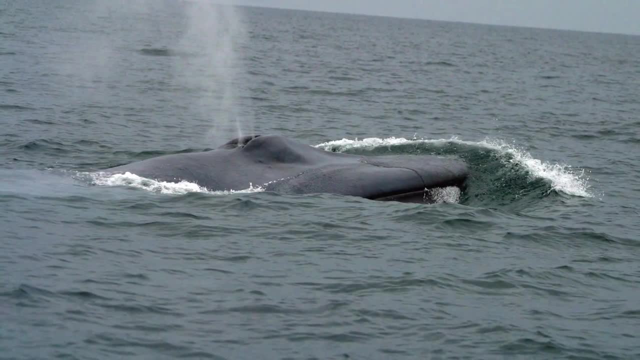 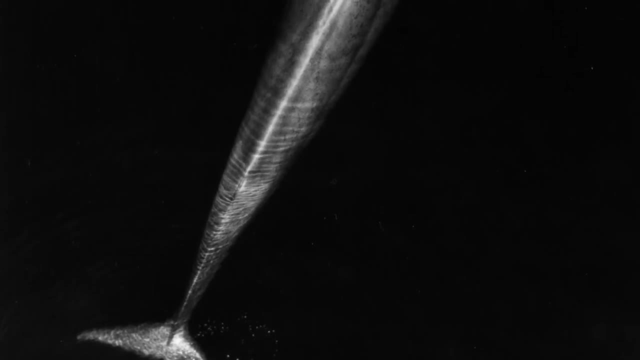 of the more exotic creatures that existed in each geological epoch. So this idea that complexity is getting more in the universe, I mean that's anti-entropic, But life seems to be anti-entropic. So what are we left with? 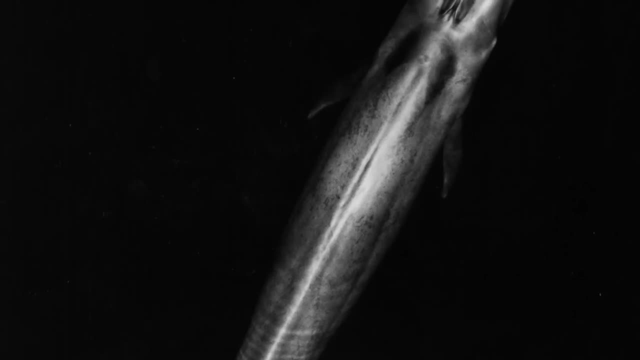 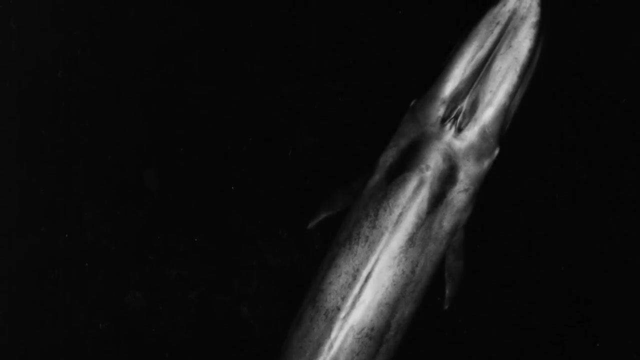 We are left with this idea that there's a suppression field, turning that reset to clock Evolutionary clock over and over again, while in the ocean, say, phyla are getting more complicated, At least they're like on Earth, they grew fish. 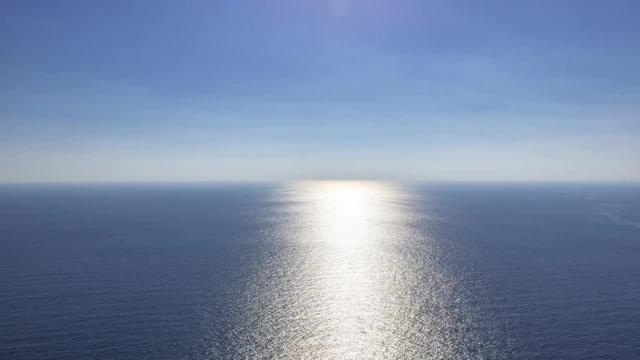 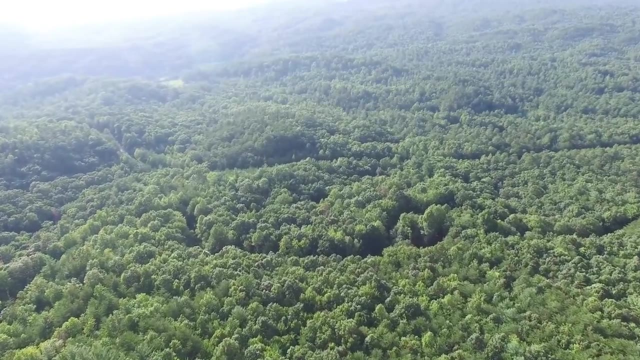 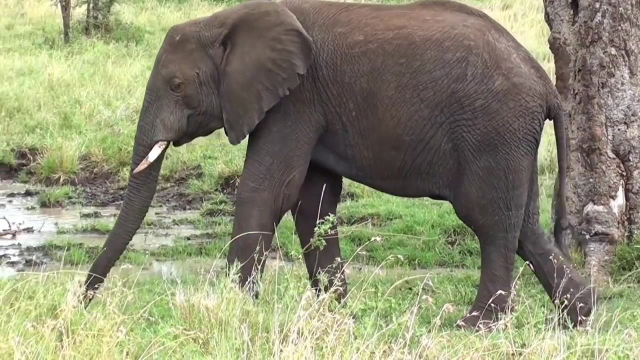 Fish were more complicated than the worms and the other low forms, using a bad terminology. that existed Until the suppression field became long, became longer than a couple hundred million years, And then the land creatures would start to get large and complex. 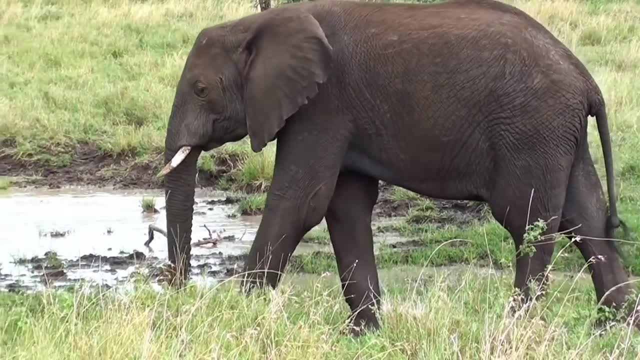 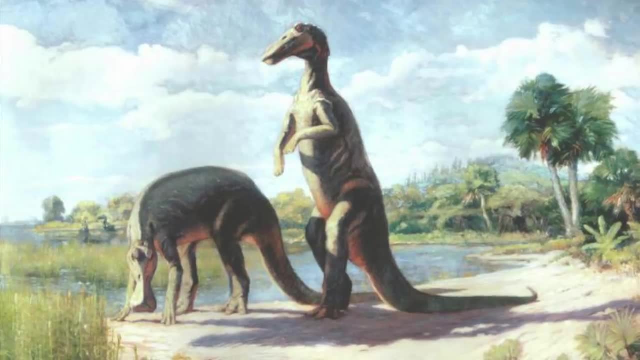 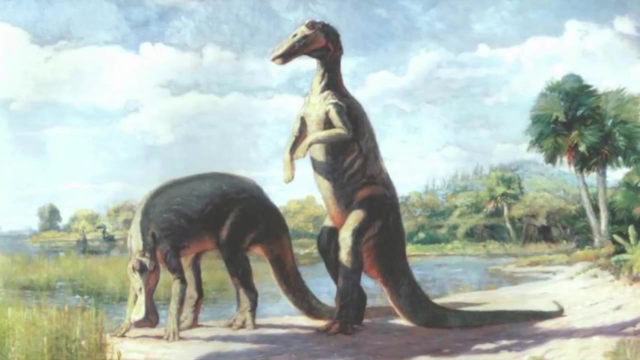 In my paper, I was enthralled with this idea that dinosaurs and all the reptiles that were associated with that class were extremely successful. They lasted for 200 million years and they filled every single ecological niche you could imagine. They may or not have been intelligent. 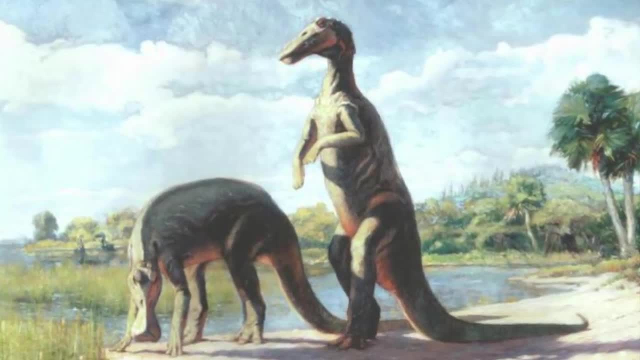 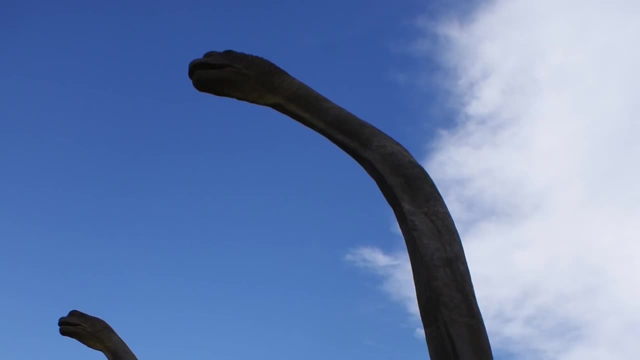 but they certainly didn't produce a civilization that could modify the environment in any kind of big way. Mammals lived with them for a hundred million years and they really didn't do anything, while the dinosaurs filled most of the niches and the mammals filled small niches- burrowing niches, scavenger niches. 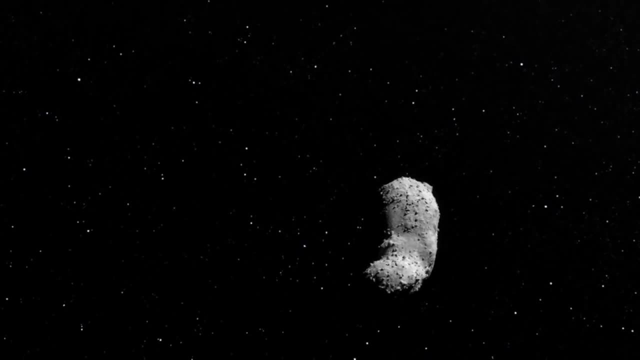 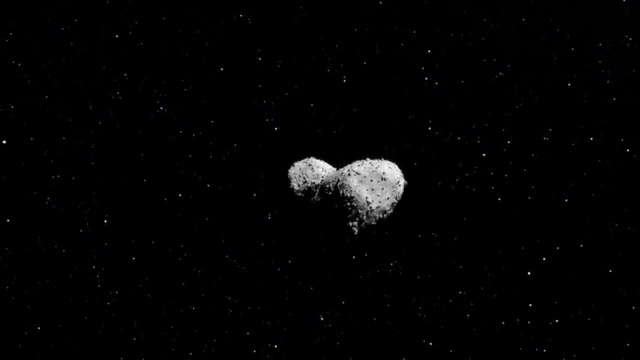 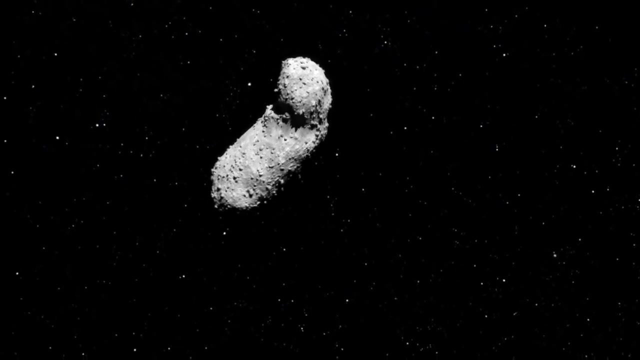 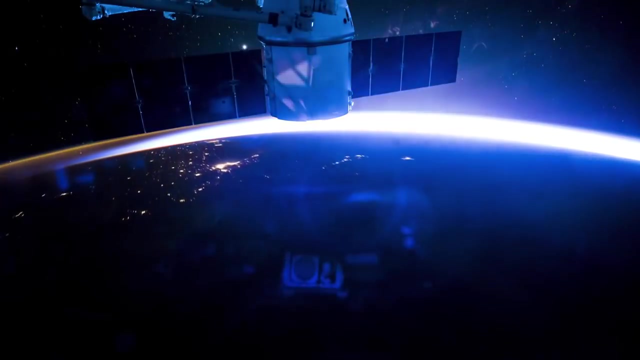 But when an asteroid strike took out the dinosaurs, volcanism, asteroids and bad luck took out the dinosaurs and mammals could actually explore all the different ecological niches and explore body plans and explore how to survive. They got more complicated And it only took 70 million years to come up with primates and primates led to our intelligence. 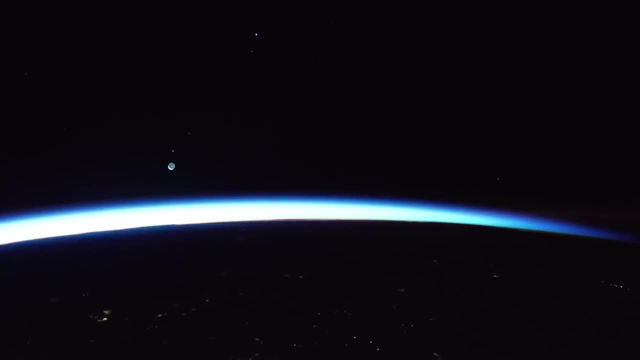 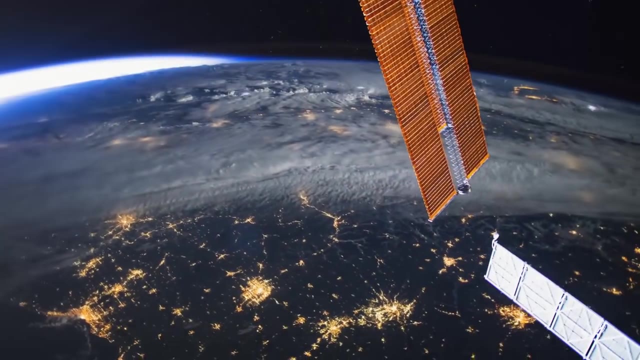 Not a hundred million, but 70 million, which I find interesting. Now you know, our primate intelligence isn't the only way to get at intelligence. I've heard you mention before and I certainly use my octopi. they're really smart and they're mollusks. 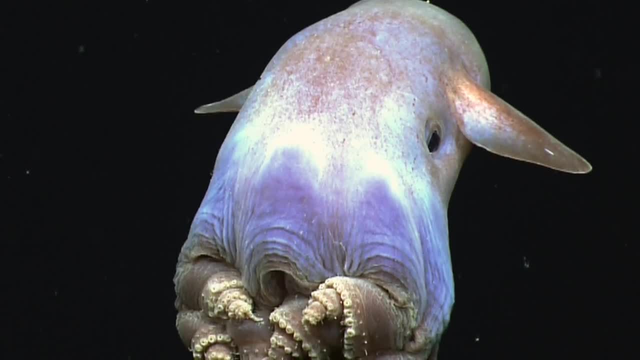 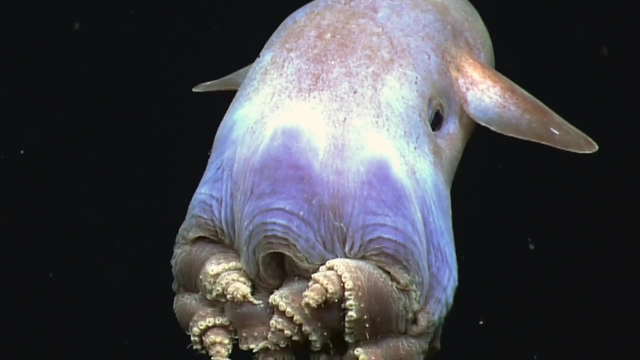 They have nothing to do with primates. They don't even have a vertebrae, Completely devoid of them. but they're plenty smart. But they don't live with primates. They don't look like they're going to produce a metal-smelting industry any time in the next million years. 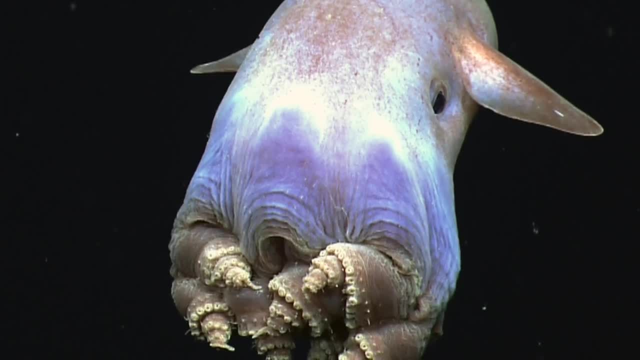 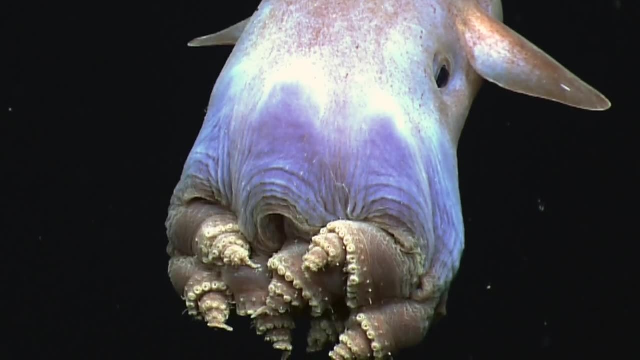 It just doesn't seem to be what they're designed for. That's another solution to the primate paradox is that most life is locked in oceans. It might be very intelligent, but it's stuck there because it can't launch rockets. It can't launch rockets. Now we're on the high end of terrestrial planet scale, so we're close to the edge of being able to launch rockets, but we're able to do it. I don't know I mean. to me this is: We have like at least three different classes of very intelligent creatures on Earth. 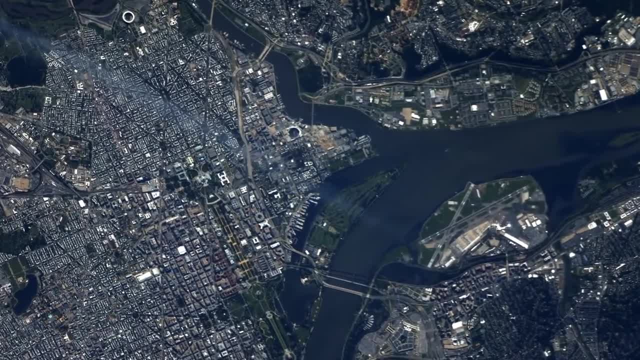 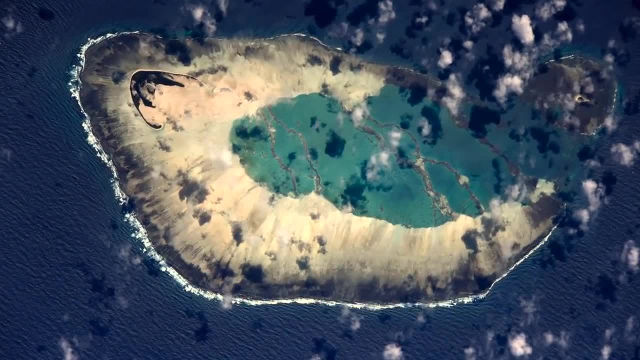 There's primates and there's birds and there's octopi. It seems to me that intelligent life is pretty easy to form, And then we get into what intelligence means. But the purpose of this conversation is: can we make spacecraft? 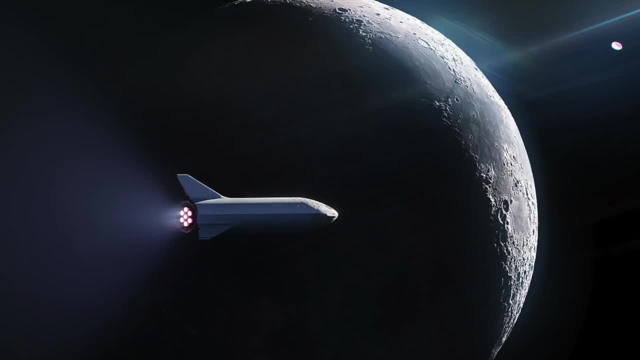 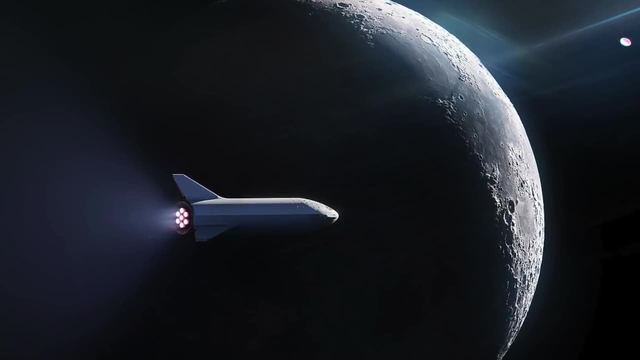 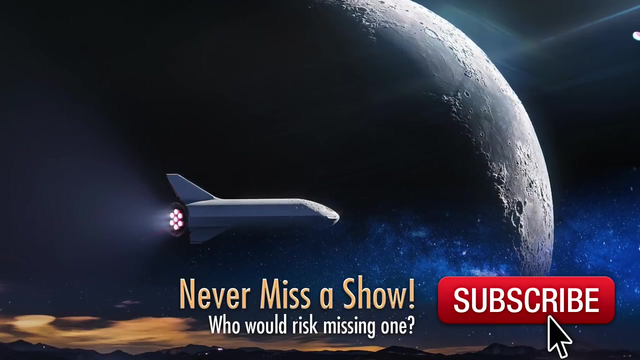 And we haven't gotten out of the solar system yet, other than with probes. Now, this idea that you mentioned, that life is anti-entropic, meaning that it gets more complex as time goes on, at least with our sampling of one here on Earth, that begs a question. 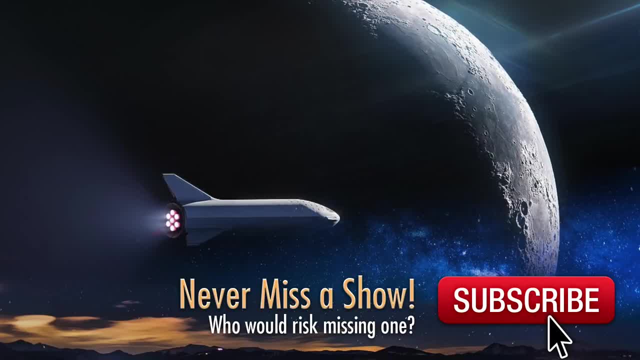 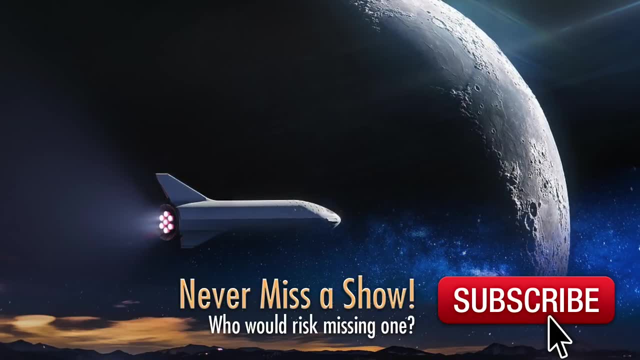 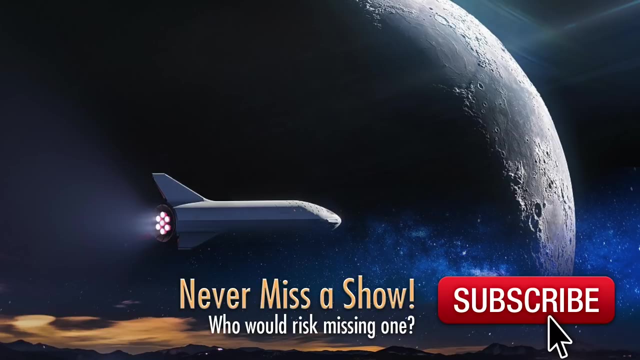 What does life end up? You know what is Earth going to look like 100 million years from now, especially with a technological civilization on it that can alter evolution. So could it simply be that the solution to the Fermi paradox is that, once you get to a certain level of complexity, 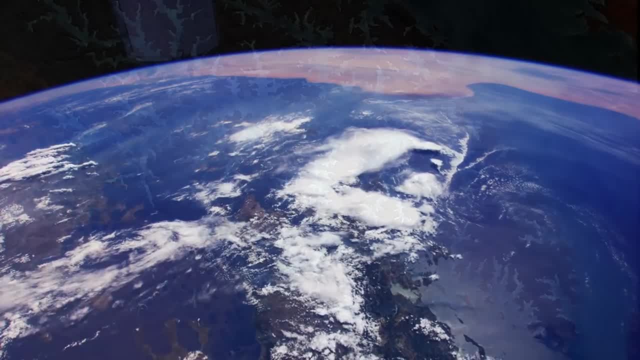 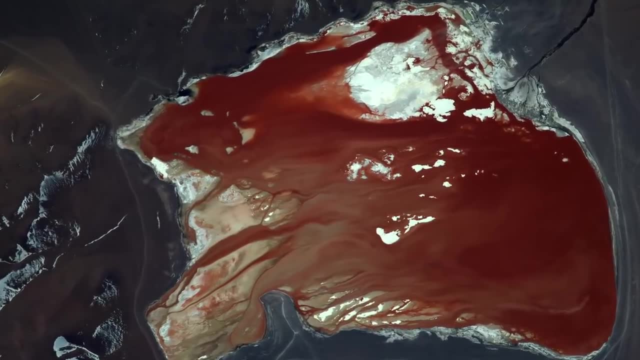 you become unrecognizable as life. Sure, I mean so. Whenever I hear this kind of argument, I mean it's absolutely respectable and it makes absolute sense. I'm just left with. So you're a space-faring civilization. 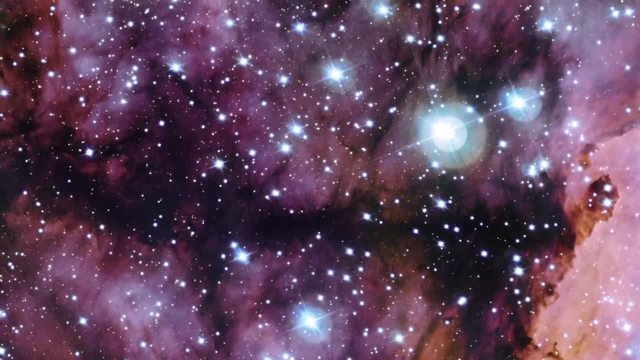 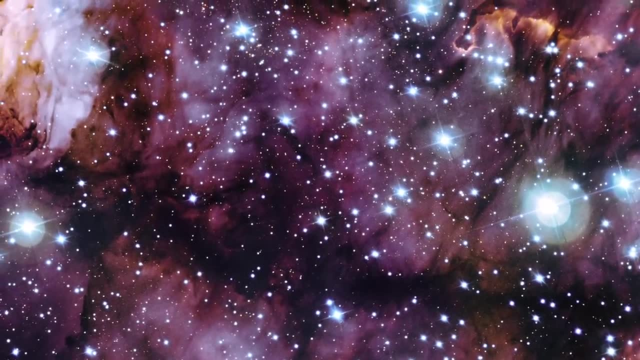 You start moving out to different stars. After a million years your species evolves to a different species, probably in all directions. So now you have a big diversity of species. Maybe most of them go that way. Maybe most of them become crystalline structures that don't need to move and aren't really visible. 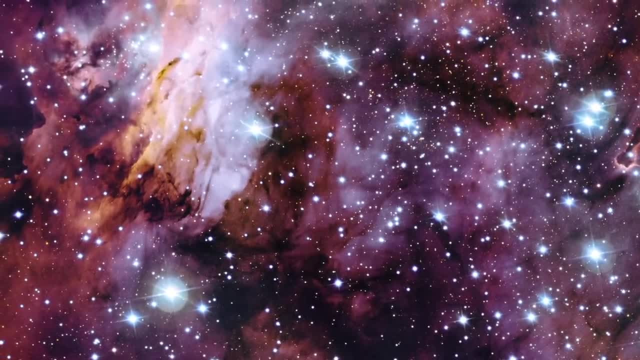 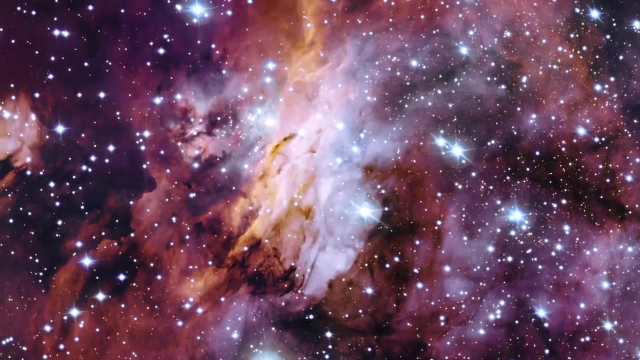 by electromagnetic means, But it only takes a few to keep on this path of going through the galaxy such that you would see them. I mean, the thing that we're looking for is not- may not even be- the average space-faring civilization. 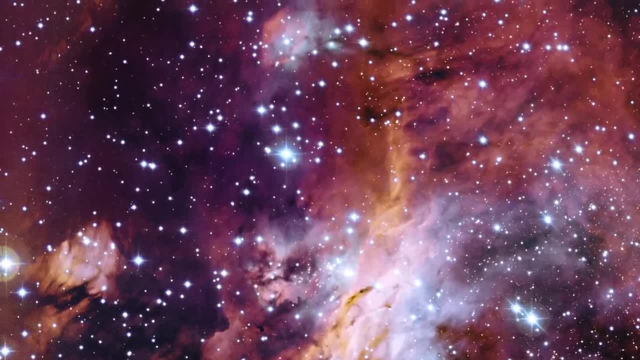 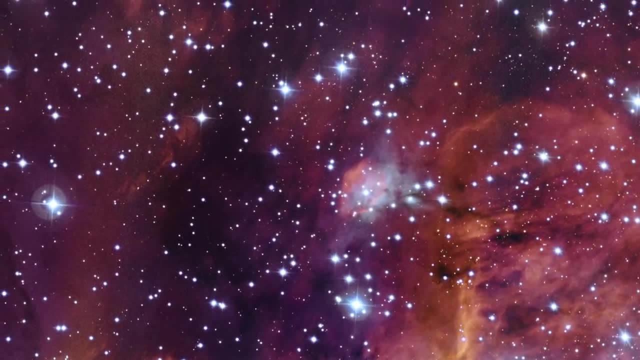 It's just the ones that are expanding. I Who is this? I think it was Cervovic who has this idea. No, it's Jason Wright. He has this idea that we get into this monocultural fallacy. We think of basically the British Empire taking over the galaxy. 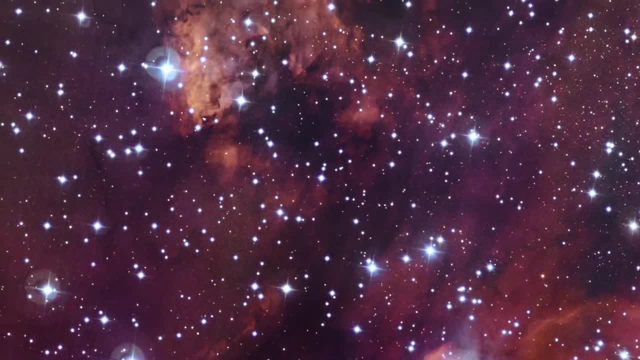 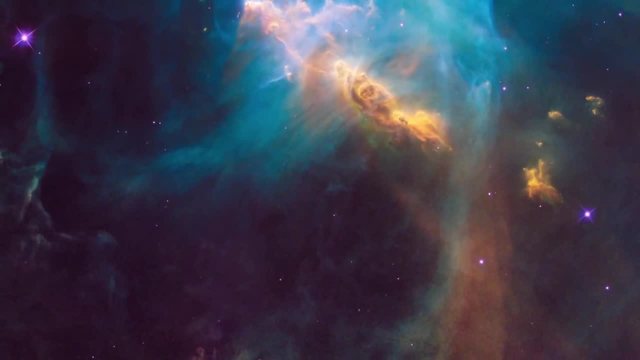 And really it would be. Even if it started off as one species, by the time it got halfway around the galaxy it'd be many, many, many, many species, probably pursuing different ends, each one a different end, in different ways. And at some point it becomes difficult to tell what is a different species, because if you have a civilization that's genetically modifying itself or it's creating custom genetics completely out of nowhere, you start to lose the ability of being able to tell what is actually alien. 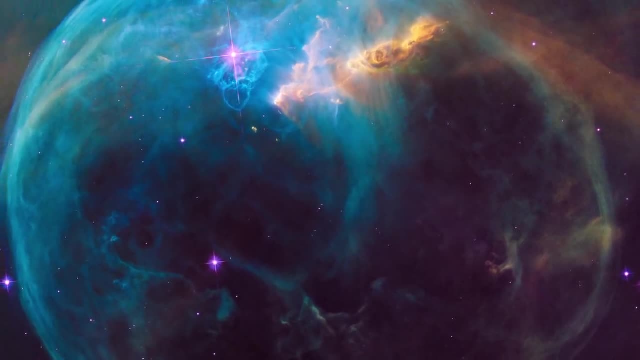 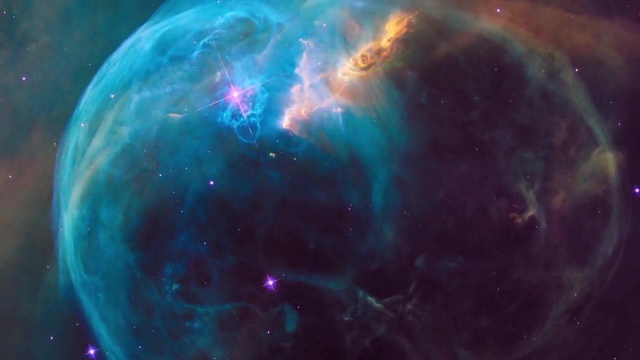 or what was once related to you at some point, Especially as you go out into the galaxy. this gets much worse over time. If you go talk to paleontologists, they have a hard time understanding species on Earth. They're not static things. 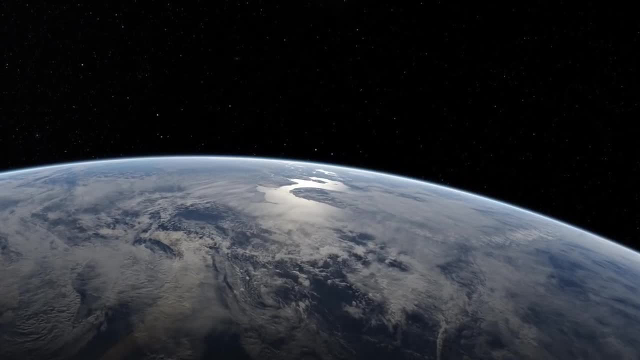 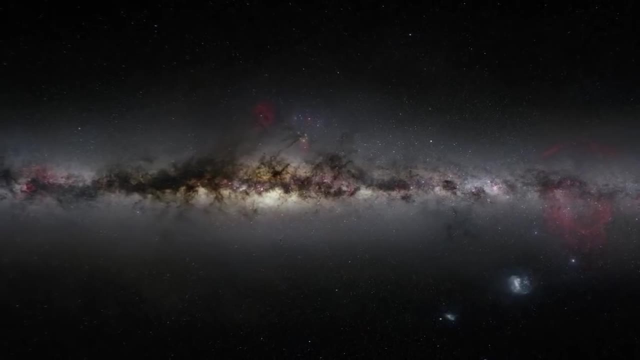 They're not well-defined, They merge into each other. We're just saying that technologically you can make that much more interesting, Absolutely, And you could end up Say, humans, head out into the galaxy and settle it over, you know, X million years. 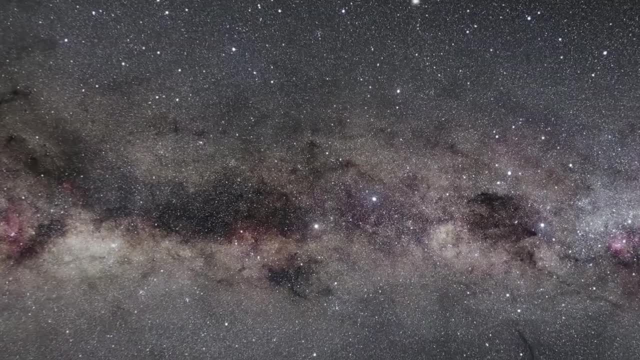 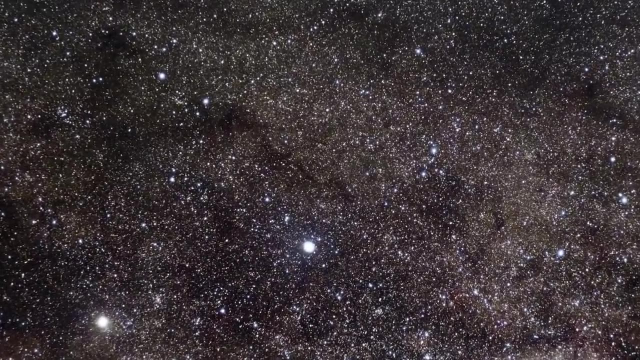 Then they stay isolated from each other because of distance. Eventually you can't really tell you know 100 million years from now, you can't really tell that you're related to this other species that's halfway across the galaxy. So it's this million-year timescale. 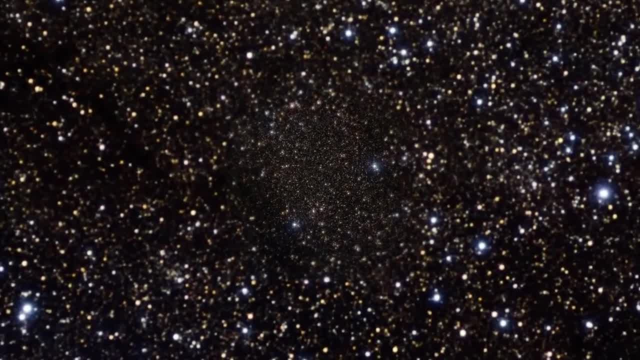 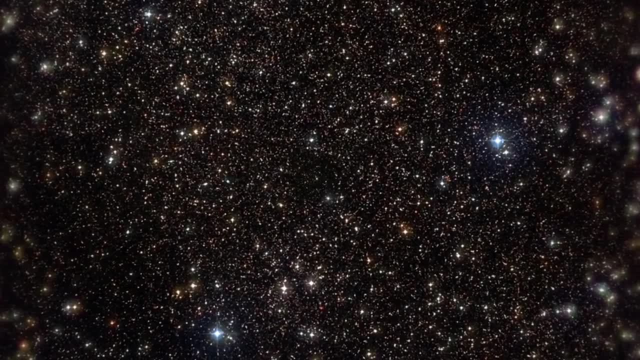 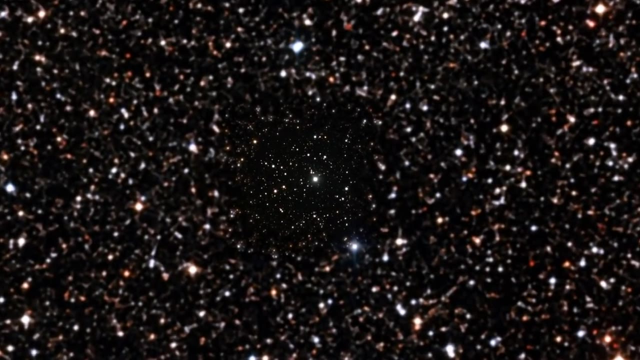 Species are about million-year timescales And I don't think I can imagine humans being humans after a million years. I think we'd just be something else. That's just how evolution works, Even if it's technologically driven. it'll be just different. 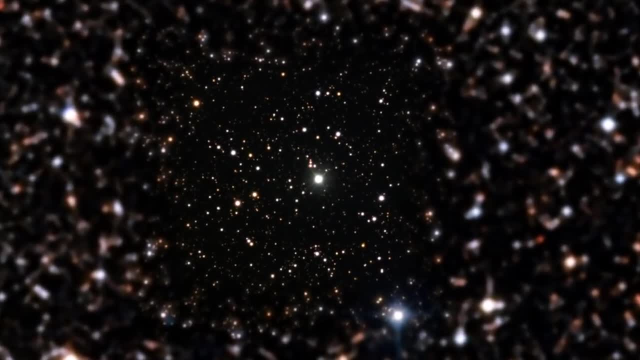 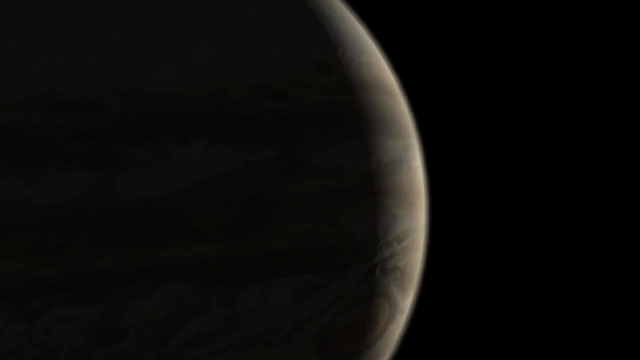 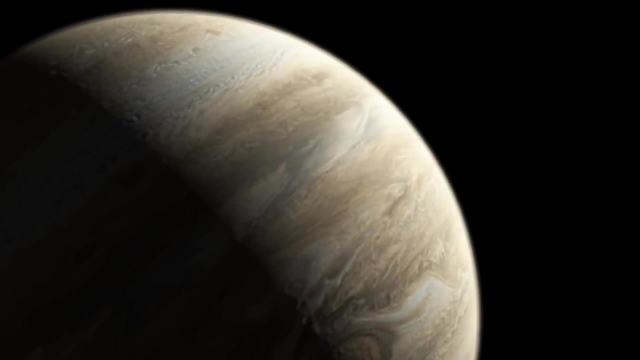 But a million years, Again, a million years. So if there was a million-year civilization in the solar system, the solar system would look nothing like it does now. It's just too long. You'd be so engineered. I continue to be enthralled by how natural the whole galaxy looks. 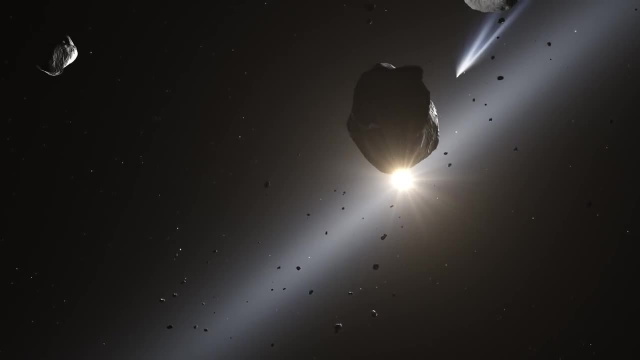 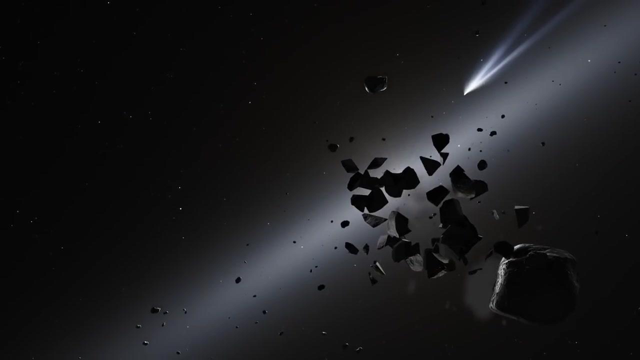 Well, even in terms of simple, simple resources, we look at the asteroids, you know, the meteorites that are falling and they're full of all sorts of really valuable stuff, like iridium and different- you know platinum, things like that. 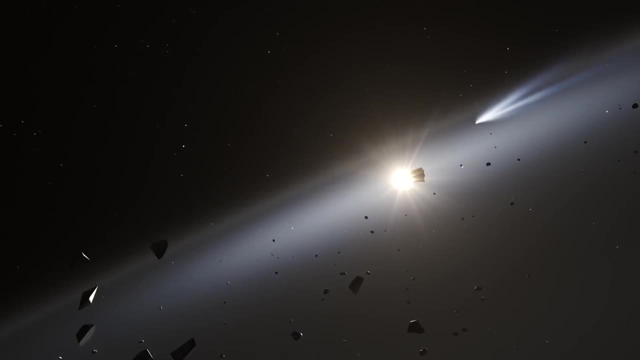 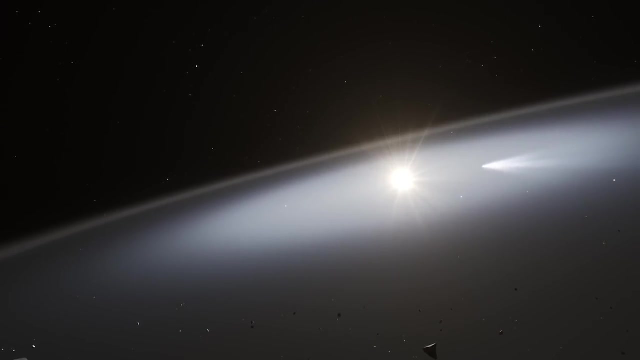 If someone had been here, they probably would have taken that by now. Yes, exactly, Or out in the Kuiper Belt where the water is Yeah, So it's. Why am I riffing on this? We imagine the scenario where civilization is. 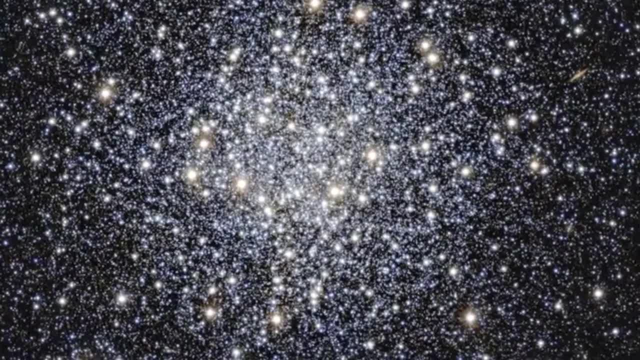 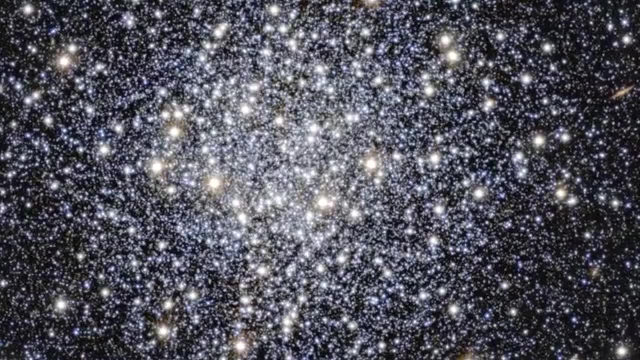 moving through the galaxy slowly in million-year timescales and they're becoming different creatures as they move. Technologically and by genetic drift, they're becoming different things in all directions And yet if they're really surviving from million-year timescales, 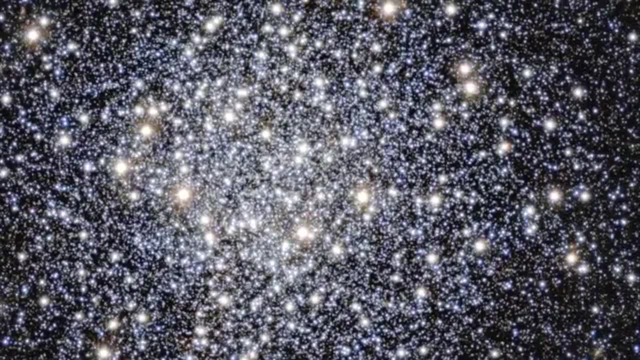 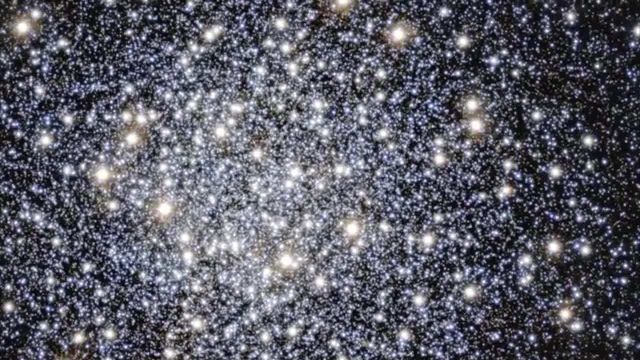 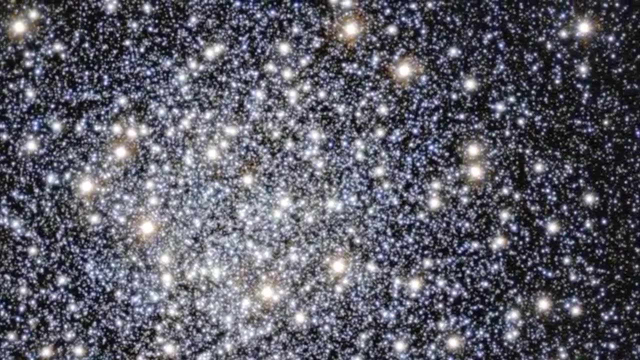 they're using up the resources of the star system they're going to, But most of the SETI and artifact community speaks of is of small probes, nanoprobes and Things that don't consume resources or much, And that's just to get away from how natural this stuff looks. 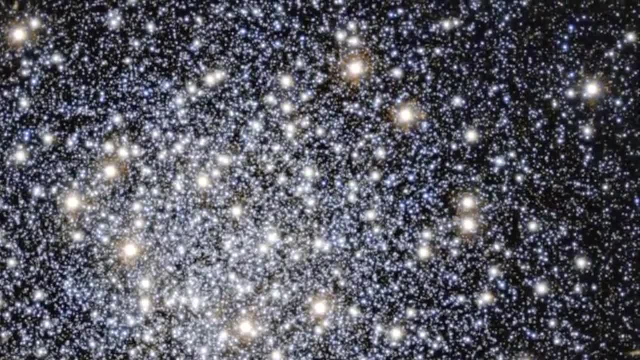 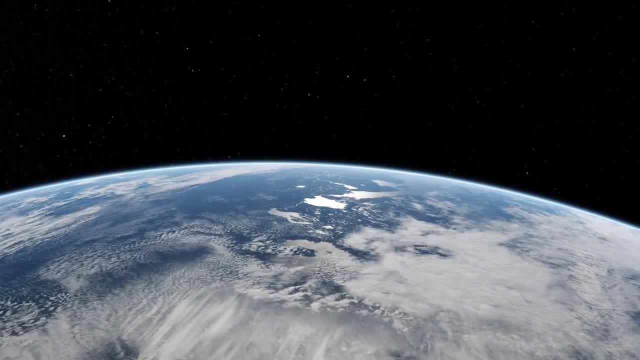 I'm not convinced. I'm not convinced that life that does I mean. so on Earth? I'll come back to this. On Earth, life seems to have kind of gone to every single niche that it can fill, and then some keeps on trying to fill other niches. 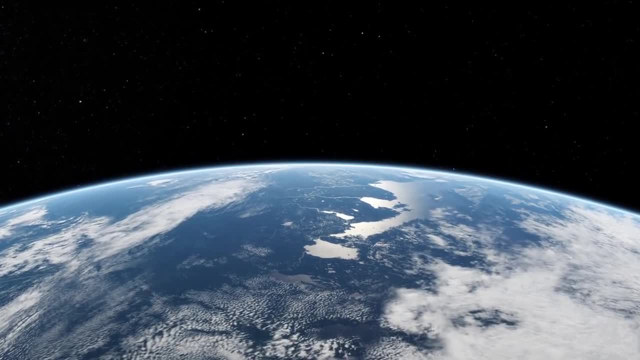 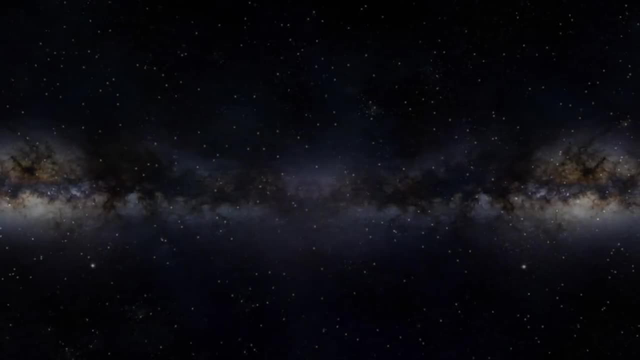 over and over again, whether successful or not, And I just think that's what's going to go on in the galaxy too, And the fact that it's just not obvious is stunning. So that's why I'm drawn to this idea of a phase transition. 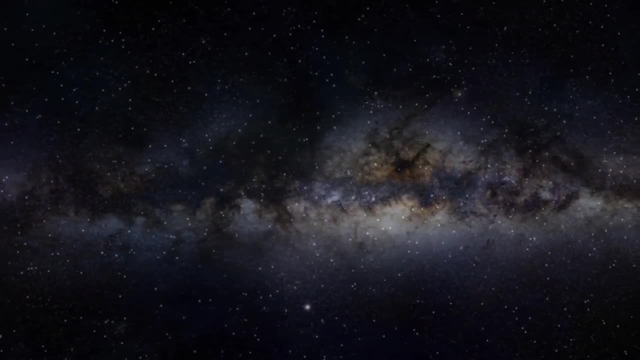 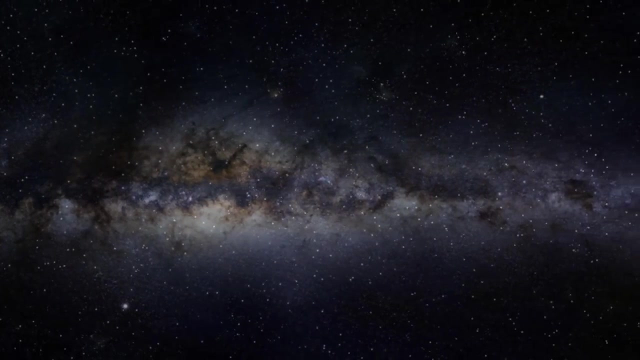 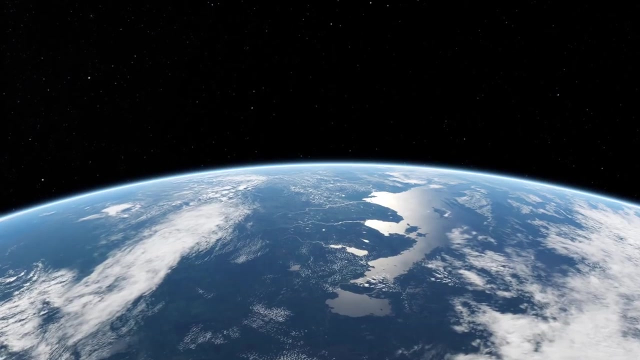 where the universe, this galaxy may not have a billion years of space-faring civilizations in it, but the odds of us being the first, or the zeroth, or the only one, it's just nil. The Copernican principle is very strong in astronomy. 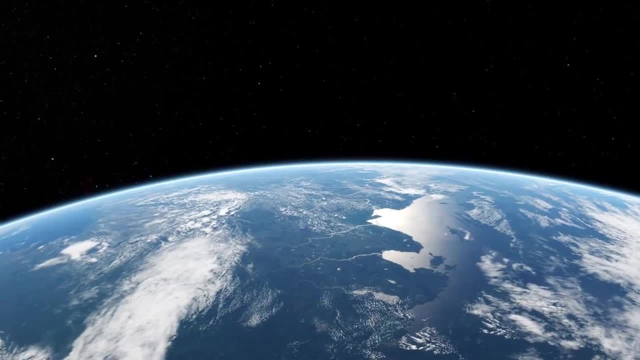 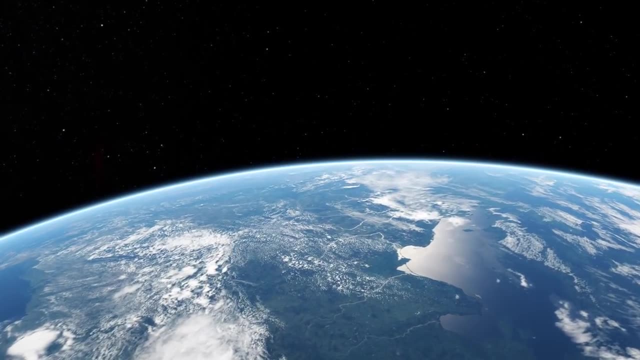 this idea that we're, on average, just common. We're not special. We have no special place in the universe. We're not the result of special processes. The things that happened to get us here may be rolls of dice, And if you rerun history you'll get different rolls of the dice. 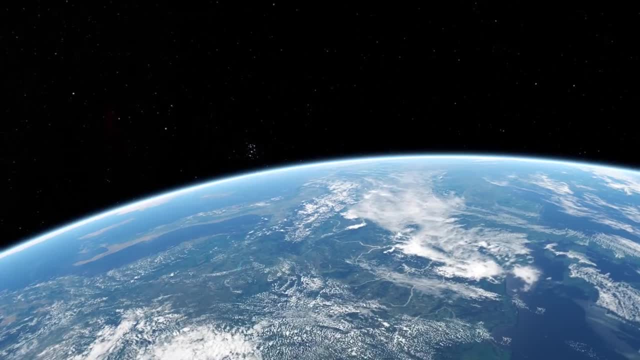 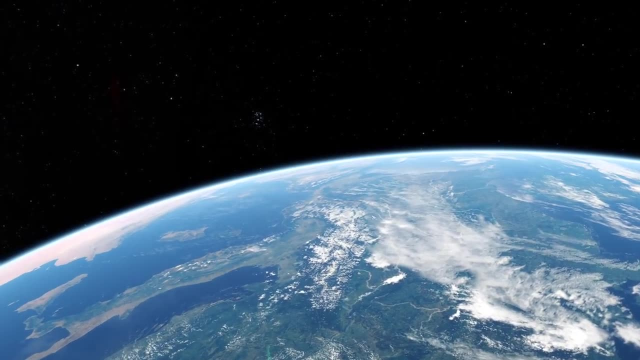 And that doesn't mean that things like us are not easy to get to conversion, to evolution. So how can it be that the universe, that this galaxy, could be full of things that are like Earth-based life forms, and yet we don't see the super long history? 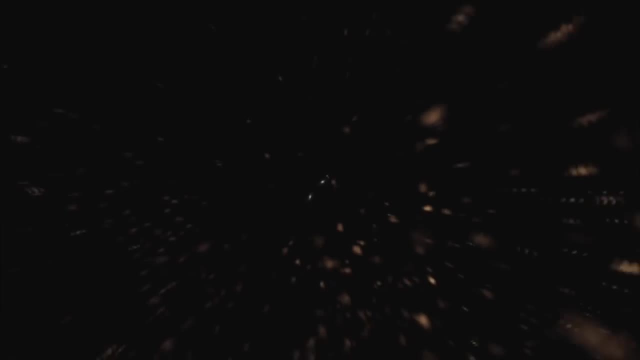 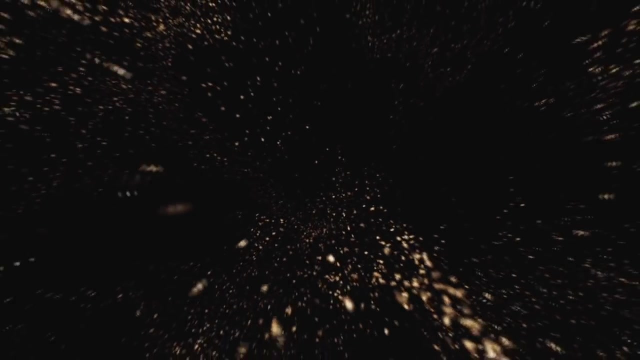 of space-faring civilizations And that's the phase transition idea, where there might have been life in the galaxy for 10 billion years, 5 billion years, 10,000 billion years. but space-faring civilizations are new relatively. 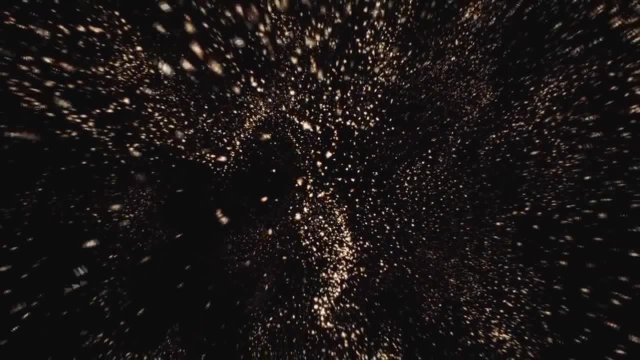 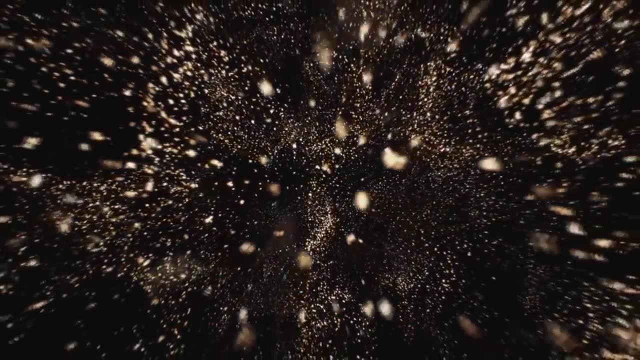 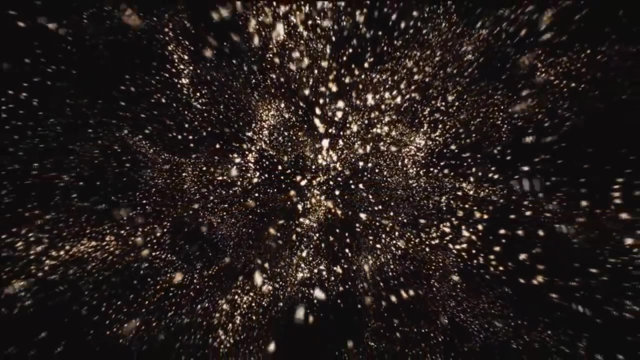 because it took so long to get complex life forms on the ground. complex life forms that can build metalworking tools, that can build spacecraft, that can start expanding through the galaxy slowly. that can take 100 million years If you suppress things for every 10 million years forever. 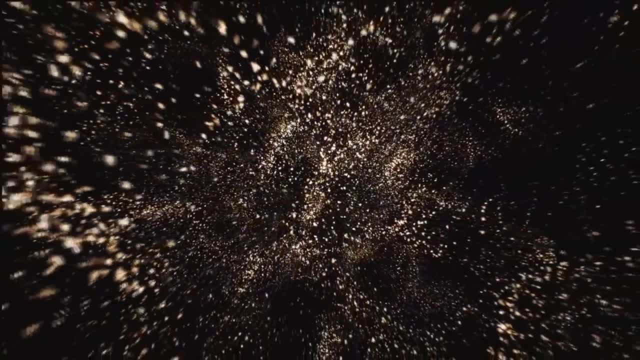 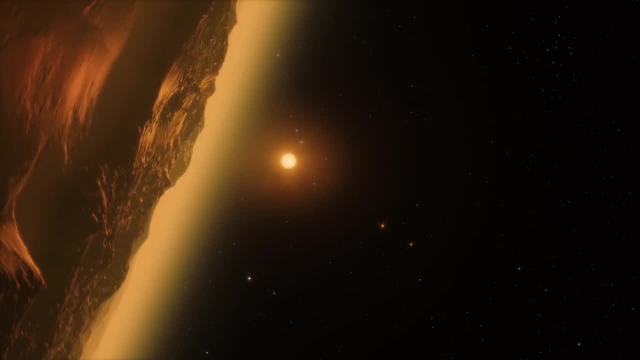 and then, finally, it becomes 100 million years or 300 million years all of a sudden, all around the galaxy, those life forms on all these planets are starting learning how to express complexity in their genetic makeup and in their body plans. They could all be waking up looking at the night sky. 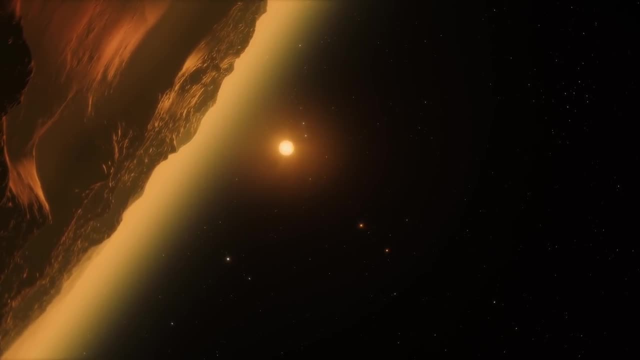 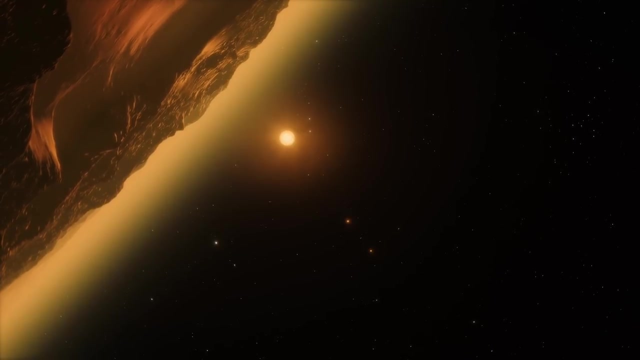 looking at the stars, saying we need to go there. I wonder what we'll find when we get there, Just like we're doing. Maybe that happened 10,000 years ago. Maybe the first one in the galaxy was 100 million years ago. 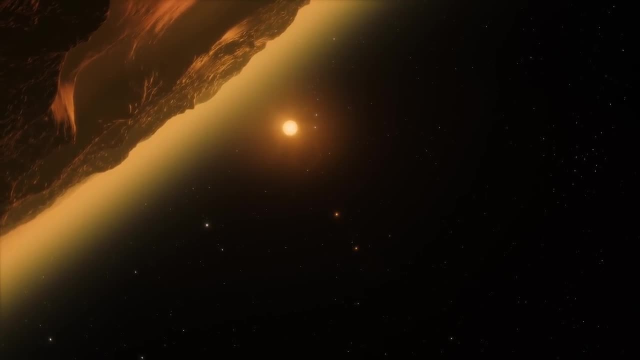 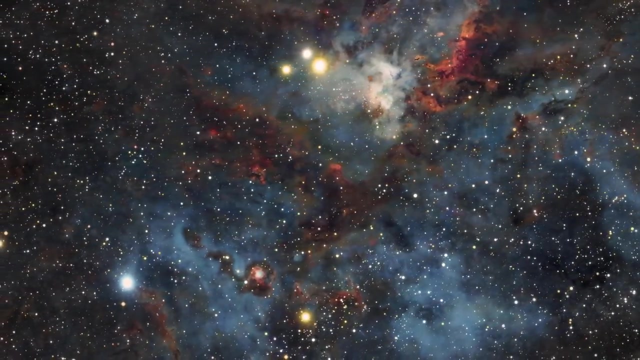 and it's halfway moving through the galaxy. It has certain issues. We might be able to see them by now. We haven't seen anything, But it's at least better than we're alone, which makes us exalted in some exotic way. 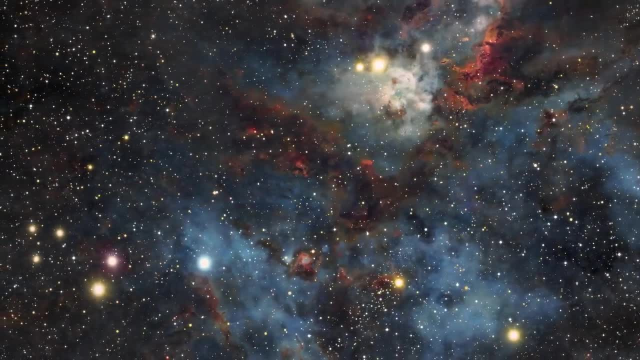 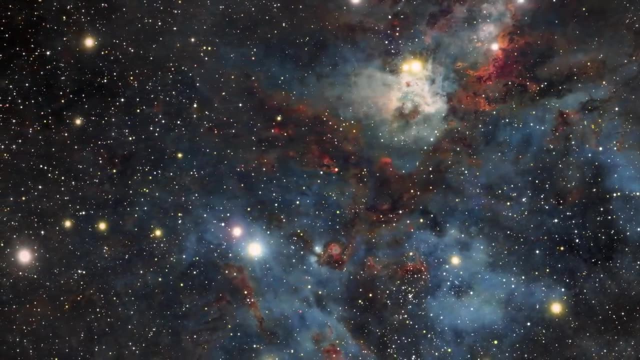 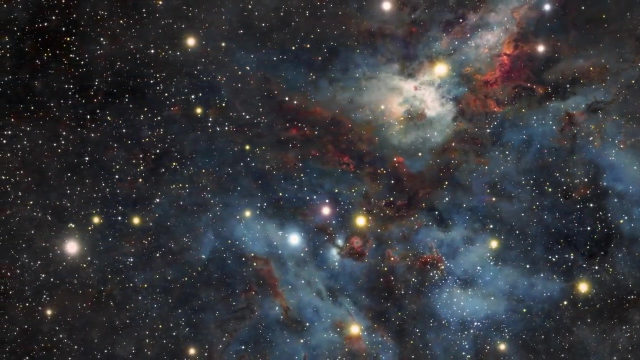 which doesn't seem to be true of any physical process that we know of in the universe. Or we're the first, which seems also unlikely. We certainly can't be the last. Why are we in this pristine-looking galaxy? Well, phase transition. 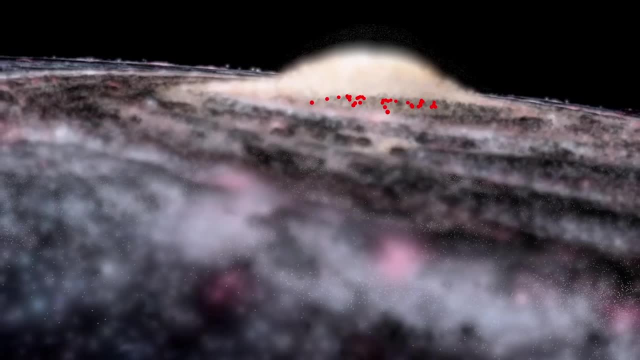 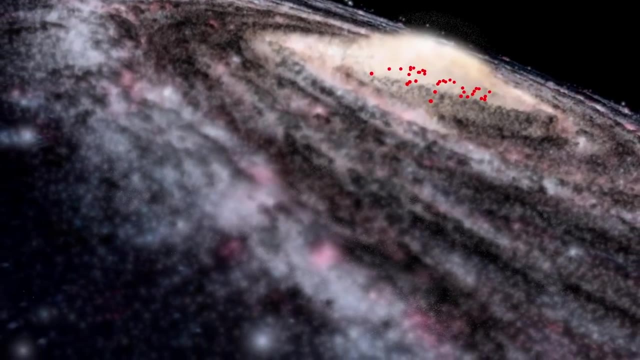 something that suppresses space-faring civilizations. Sort of reminds one of Star Trek, where everybody's starting out and heading out at roughly the same technological level And maybe somebody might be a little bit more advanced, but maybe not, And then lots of people would be less advanced. 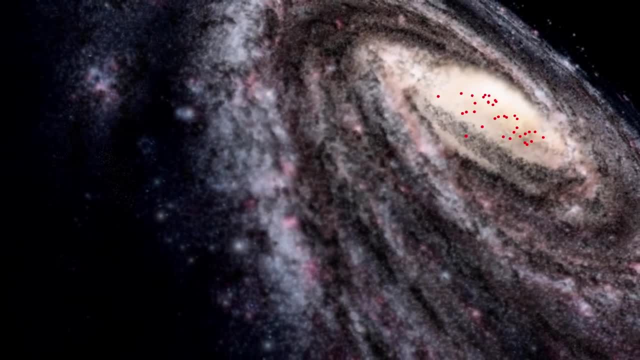 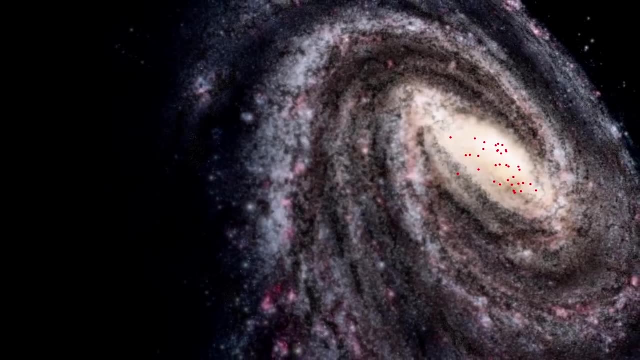 and you know and so on, so that it's sort of this awakening period in the Milky Way where everybody finally can achieve intelligence on suitable worlds and begin to head out. But this sort of bolsters the case for SETI, because if somebody else is just discovering radio, 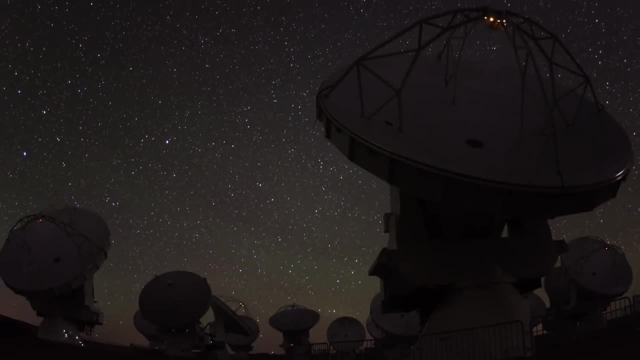 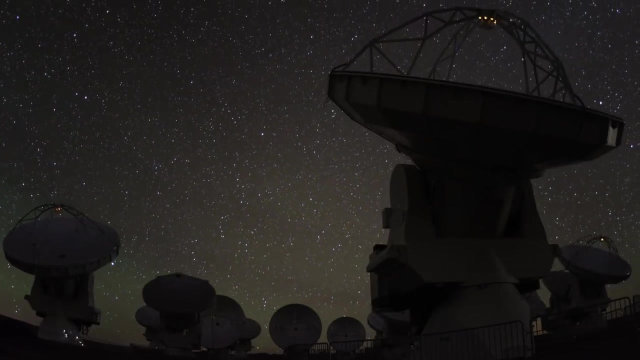 you know and saying: well, let's send a signal out there, then you know, this might be the time to look for that Exactly. I mean, there is a timescale argument. There's problems If civilization, you know, on average lasts for 10,000 years. 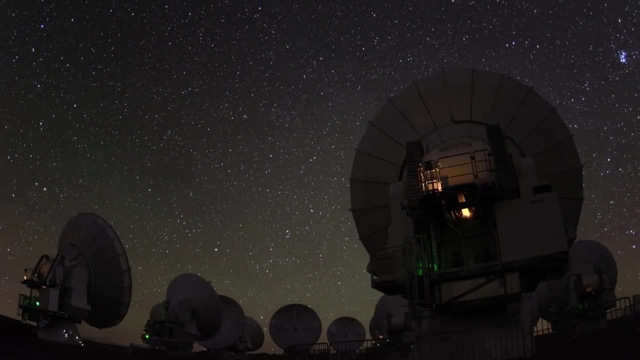 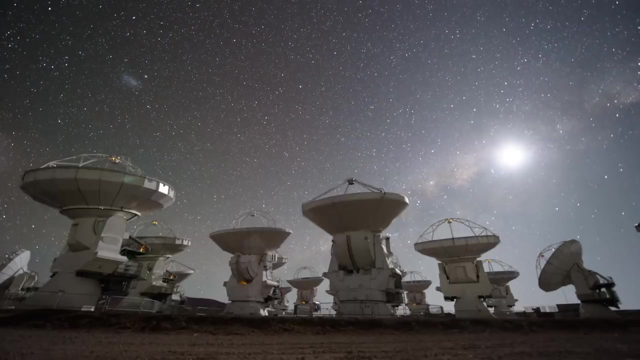 then when you're looking they may not be transmitting in the radio. But those are all problems that are technical and can be worked on. Given enough stars, looking enough places, you're going to find them. by average anyway, It's a real strong argument for doing this traditional SETI work. 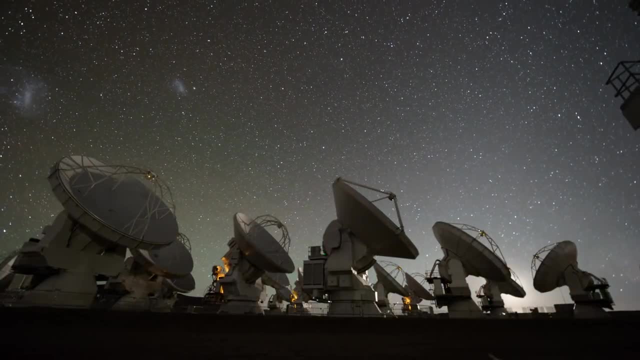 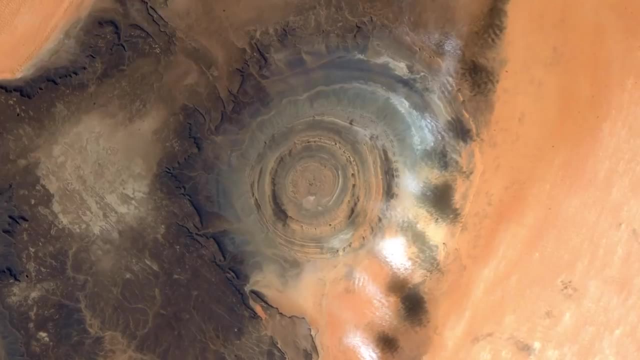 that you know we've been doing for 50 years Now. you also mentioned, too, that nature doesn't really like anything that's unique, And you know, usually you always find examples of you know, you find something. 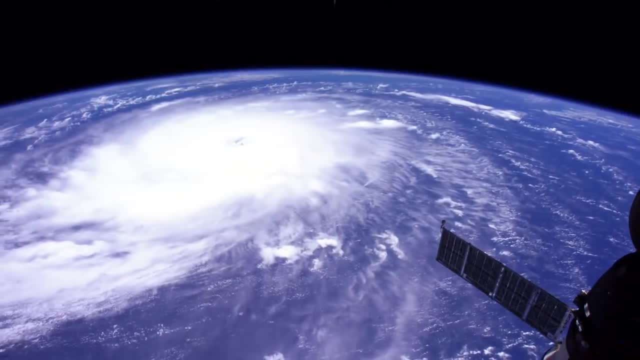 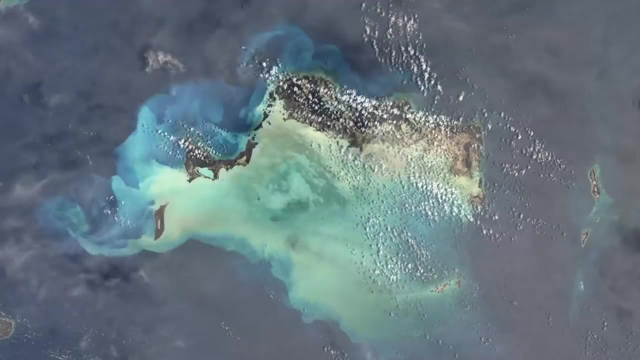 and then you find other examples of it. You know, stars doing strange things or whatever. It would seem really really odd if we were alone, because we would be a one-off And nature really doesn't seem to like that sort of thing. 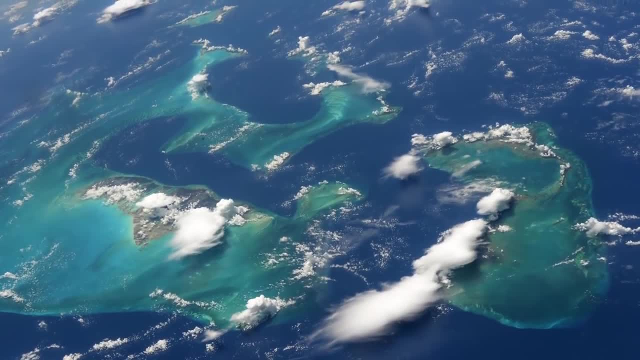 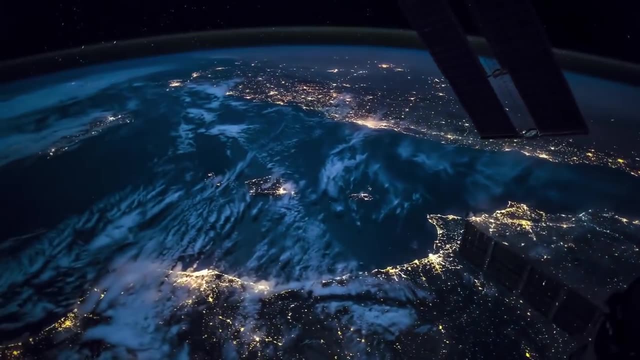 So that alone would suggest that the Fermi Paradox's solution is that no, there's life everywhere. it's just that its intelligence is merely rare, or at least right now. Now regarding extinctions, though, through gamma-ray bursts. 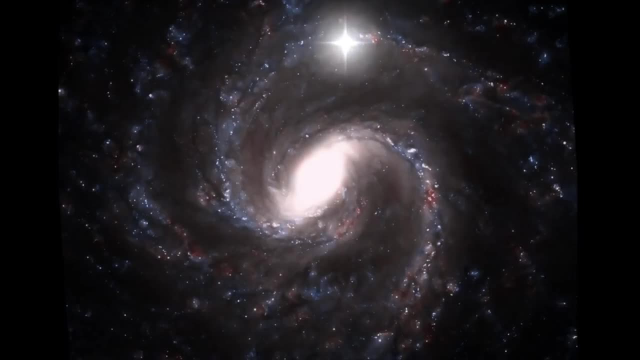 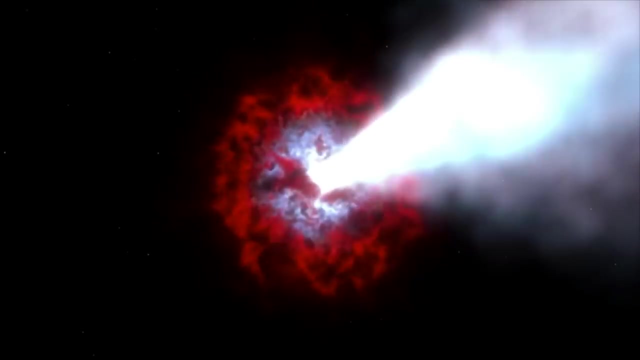 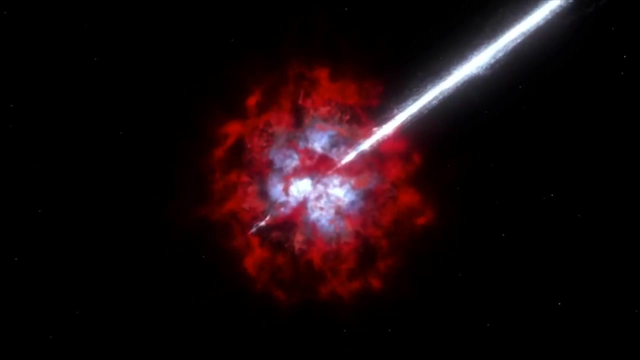 as I recall, one of Earth's extinctions extinction events may have been a gamma-ray burst. That's on the table for having been a cause, because apparently much of the planet was sterilized to a few meters down in the ocean And anything that was deep lived. 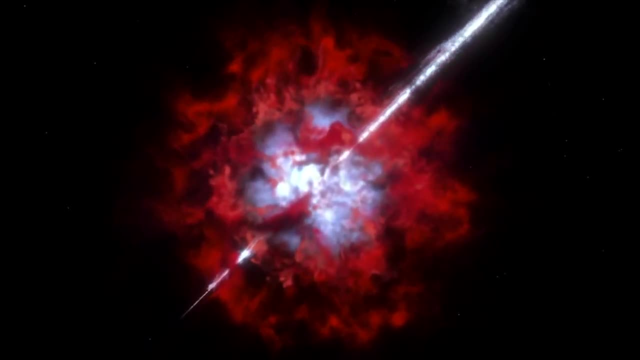 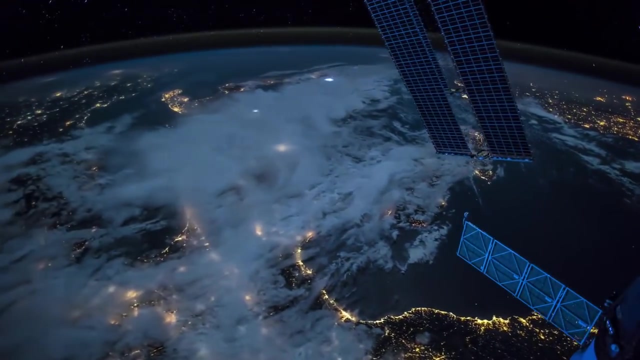 but anything that was shallow did not. So is there any other examples of mass extinctions in Earth's history where maybe a gamma-ray burst was involved? Well, that would be the most recent one. I think that's a Permian extinction event. 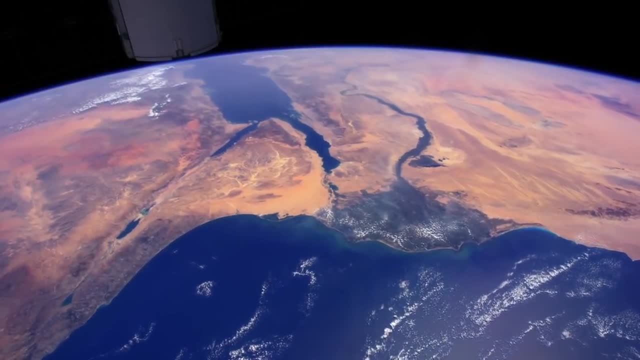 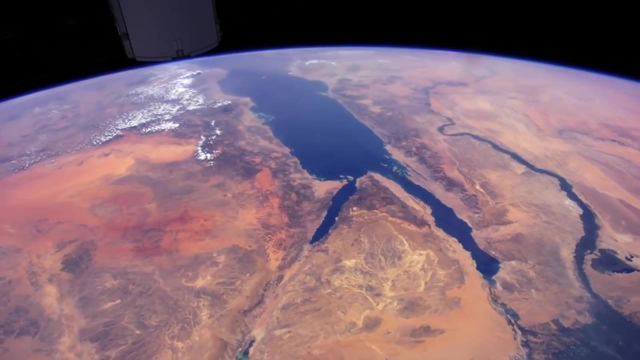 And that was a couple hundred million years ago. Before that, it's ocean-based And so there isn't. I mean, what are you looking for? You're looking for die-off in the shallows of the oceans. I'm not aware of it. You know. it's worth reminding ourselves that the dinosaurs are killed by an extraterrestrial event. Gamma-ray bursts are one of many extraterrestrial events that can affect us here on Earth. Solar flares- giant solar flares- could present a real problem. 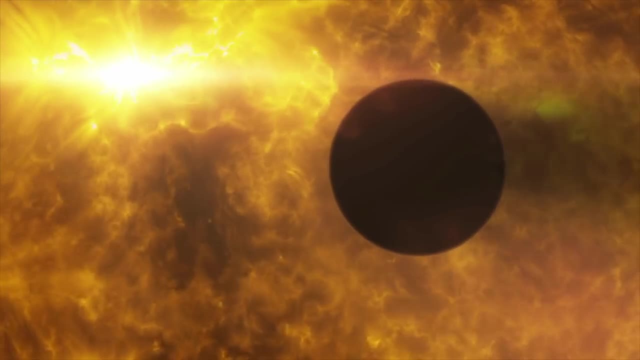 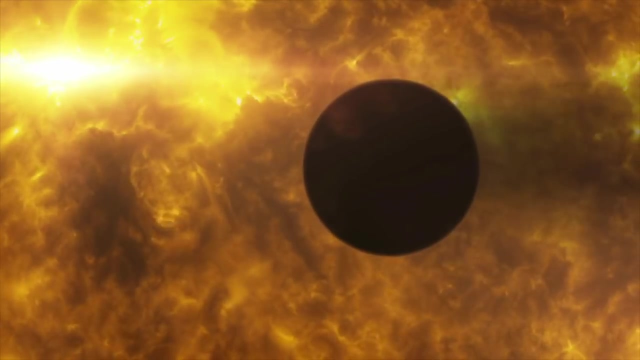 Especially to a technological civilization, Even to a knot. So mass extinctions tend to wipe out the larger creatures. What you're left with are mice, if you're lucky, And it takes a long time to build back up from that. You know tens of millions of years. 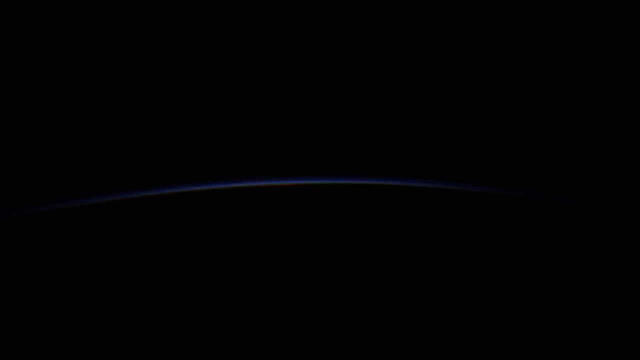 I can't think of another. In my mind the Permian's the best candidate for a mass extinction caused by gamma-ray bursts, Because it did have that kind of feature where most all the land-based and a lot of the sea-based animals died off. But the other mass extinctions, what? there have been? five mass extinctions. four mass extinctions had the feature that they killed off most land-based creatures, But not all, And slowly the ecosystem. we gained its complexity and the missions got filled again. 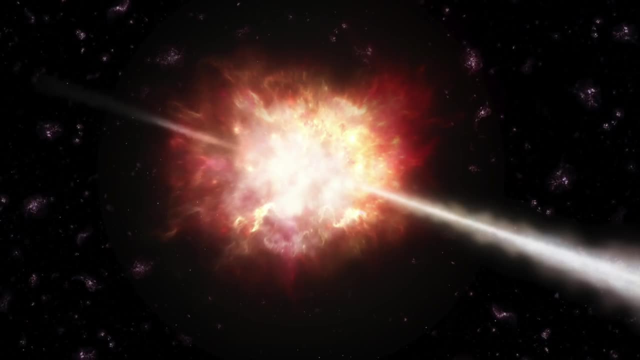 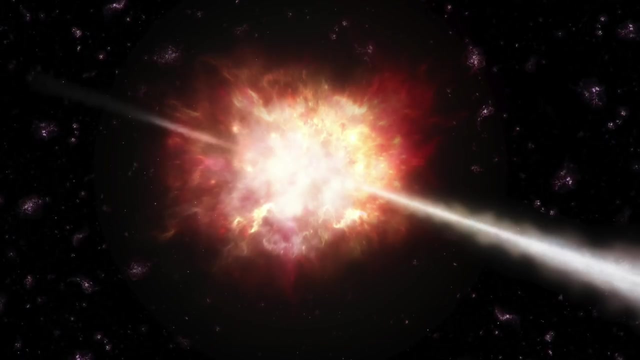 I'm okay with that. I'm not sure. Gamma-ray bursts are just sort of rare And supernovae are less rare, but they have to be a lot closer to causing damage. So, following the way I tend to think, what would be the evidence? 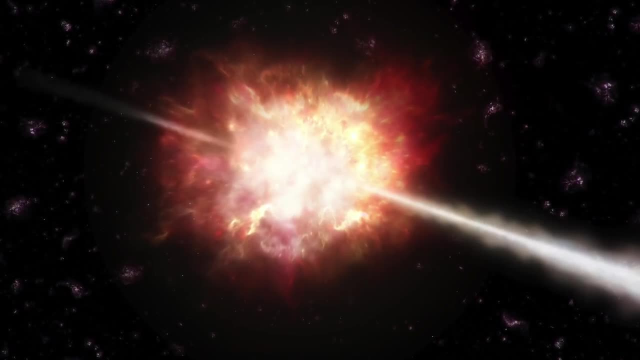 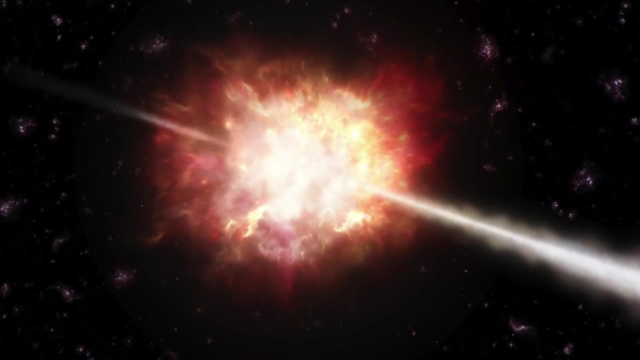 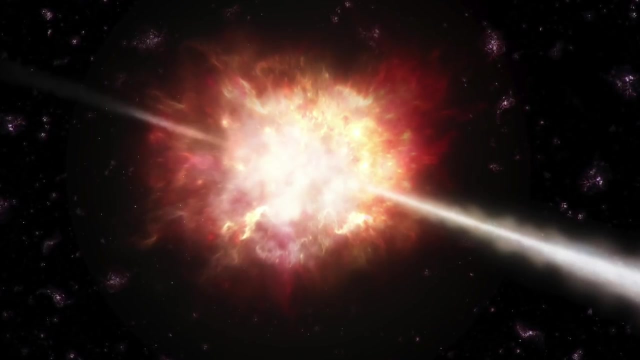 you're looking for, And in asteroid strikes, it's the iridium layer that gives you the evidence that there was something from outside the Earth that causes, as opposed to volcanoes, Gamma-ray bursts and supernovae. Supernovae might give you radioactive tracers. 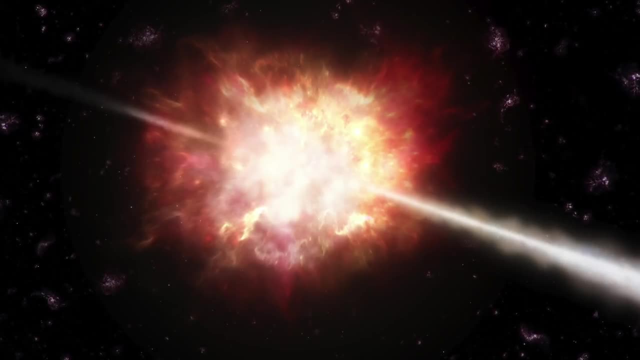 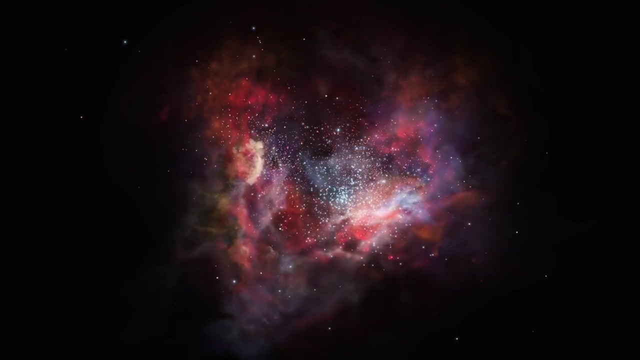 on asteroids that one could look for The gamma-ray bursts. it depends a lot on what the jet looks like, what the details of the jet particle structure is and what they do when they interact with matter. So my guess is we'd want to go to the 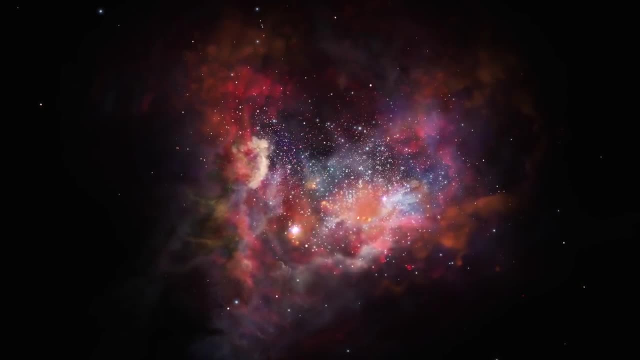 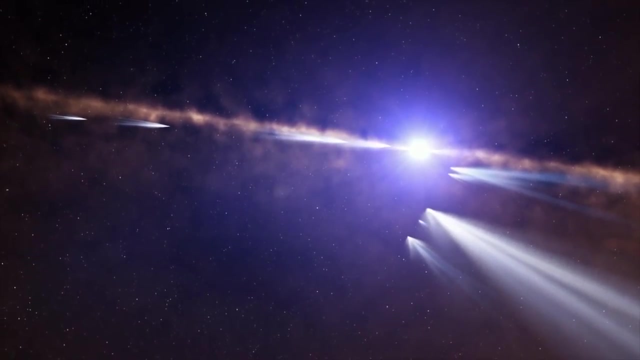 probably to the ice balls, but maybe to the rocks, either the comets or the asteroids, and start looking at them, looking at the surface layers versus the deep layers, and see if you can find traces of events in them. There's this new dark matter model, right. 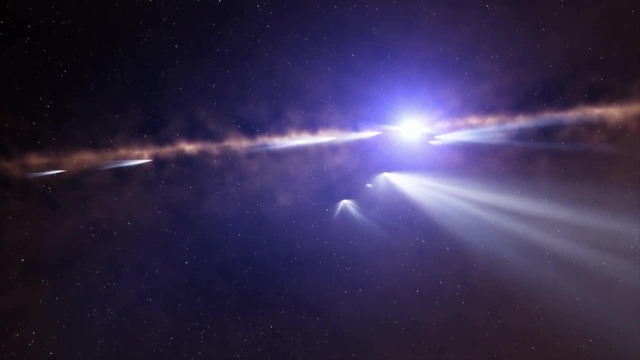 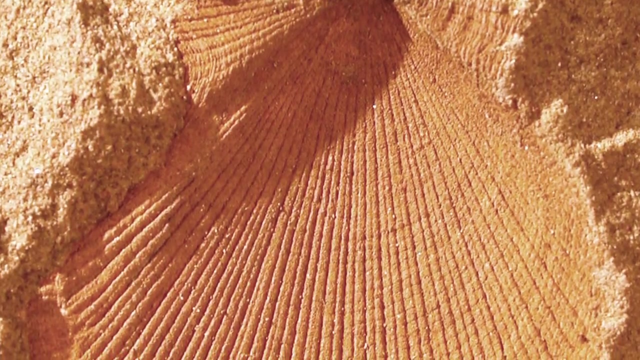 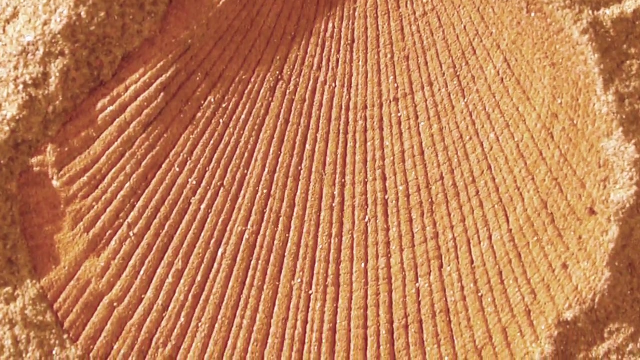 People are looking for dark matter by looking at fossils, by looking at old rocks. It's an idea. It's an idea that has come back to fruition. We might actually gain some technology from the darkness that will allow us to touch this. That was actually of great interest to me. 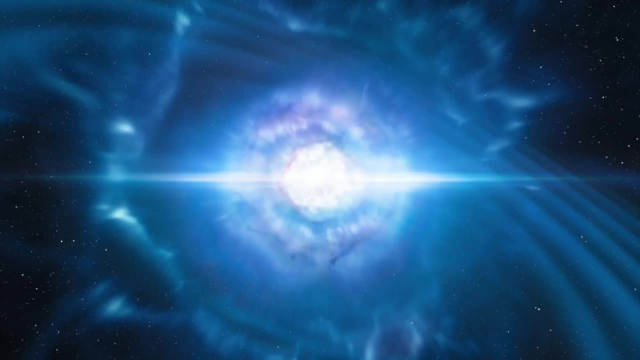 is the idea that you can study dark matter looking at minerals. Now my last question for you is: could we still get hit by a gamma-ray burst? Is this still a threat to us? Could we go extinct if one of these were to go off nearby? 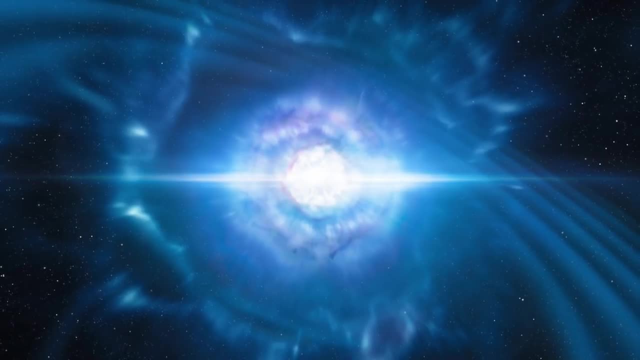 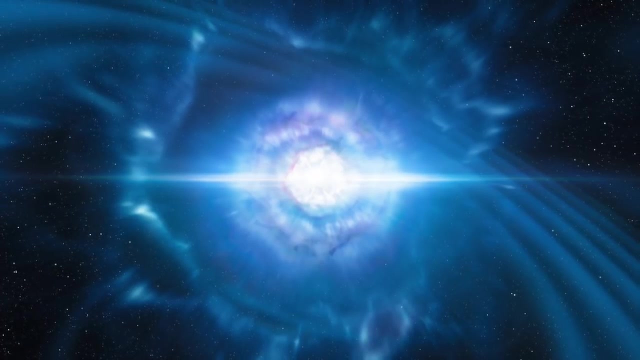 Yes? The simple answer is: yes, The odds are low. The odds are always low for that kind of thing, But they're just a lot less common now than they used to be. You have to get unlucky. So my money on an extinction event for humans. 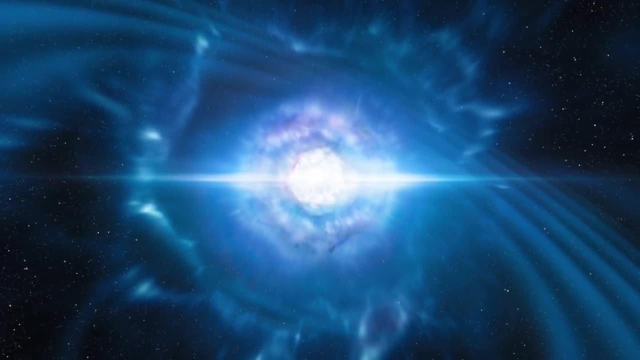 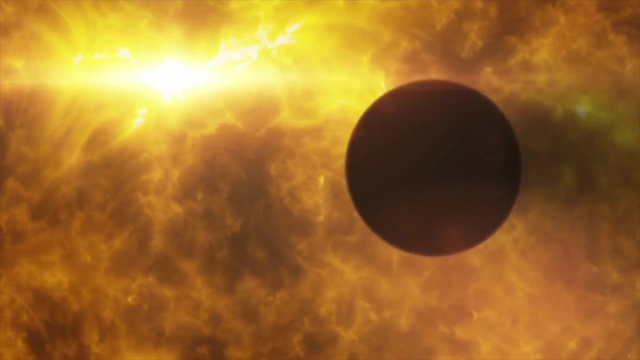 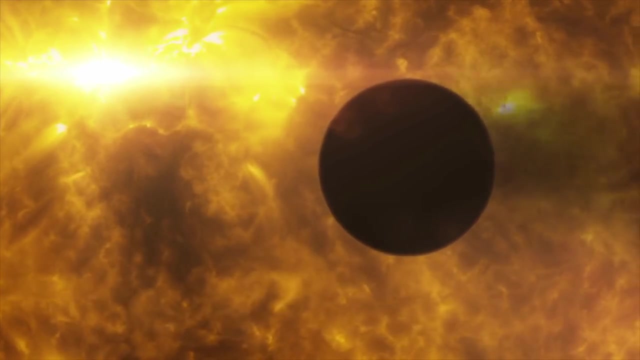 wouldn't rely on a gamma-ray burst, It'd probably be more like a solar flare. Is it possible now? solar flare, of course, is a completely different animal, but is it possible for a civilization to shield itself from a gamma-ray burst, Should they know that these two neutron stars, or whatever, are going to merge? 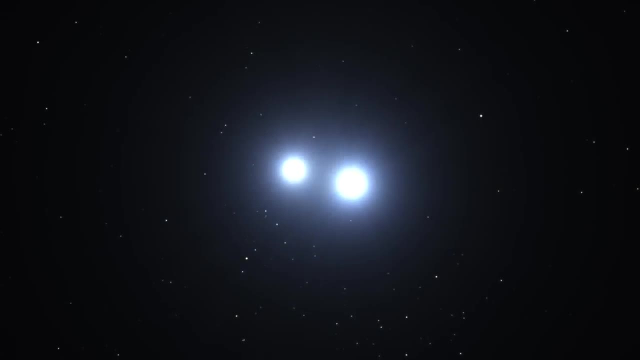 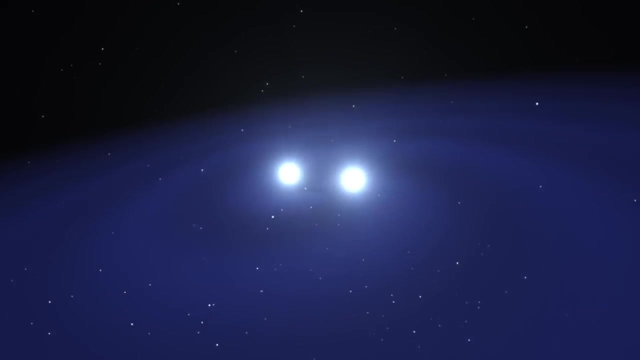 If they have sufficient time, can you avoid extinction. Sure, So, yes. So that's one of the features of the model I put together. You have to do it before you get Kardashev: Type III civilizations, Things that can harness any large fraction of a stellar energy. 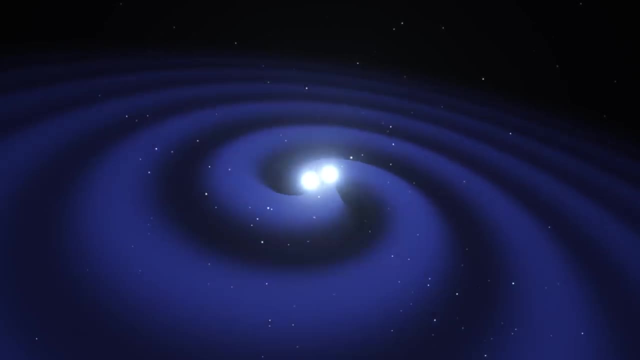 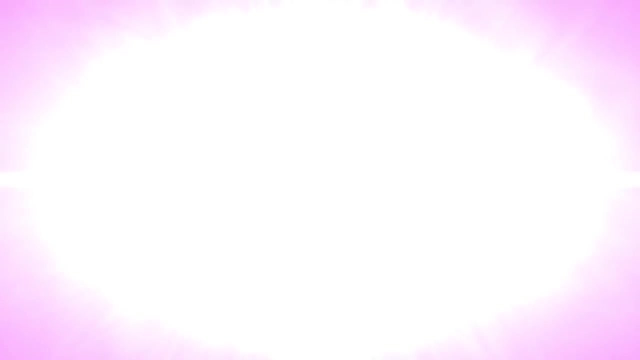 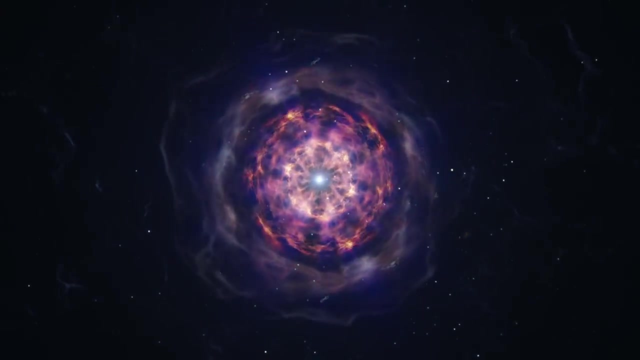 or a galaxy's energy almost certainly can shield themselves Down one side of the planet. burrow down. If you're space-faring, you can just leave the area. It may take a while, Assuming arbitrarily advanced technology, then you can reproduce yourself. if not your memories reproduce yourself by using genetic technologies. So you put yourself in the ground in a genetic form and a database form, wait for I don't know a million years and then reconstitute yourself and upload you from the database. 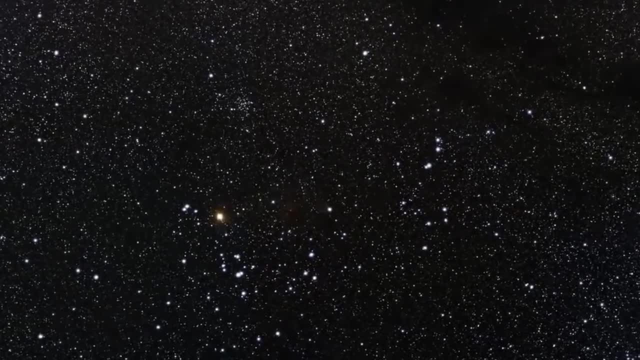 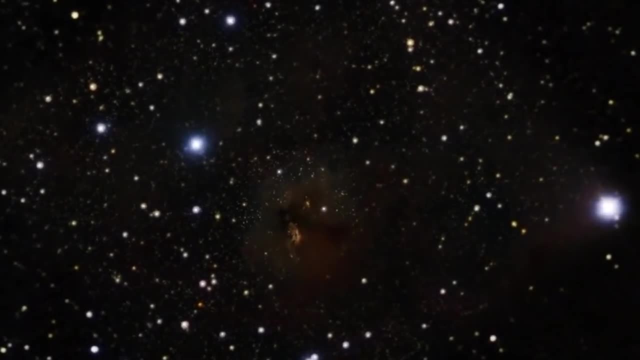 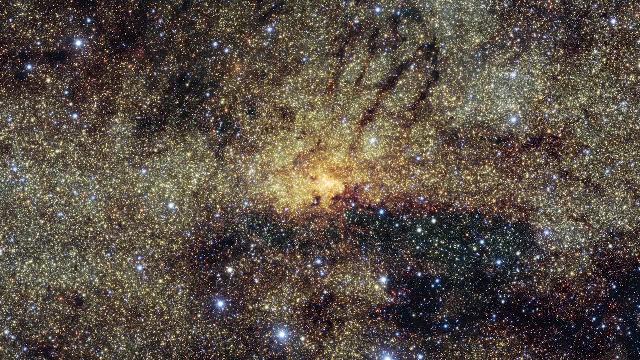 Yeah, So what you have to do is suppress civilizations before they get that advanced. You have to make sure you don't get that happening 500, 5,000 million years ago, so that you would see it all over the galaxy already. You must make sure that all space-faring civilizations 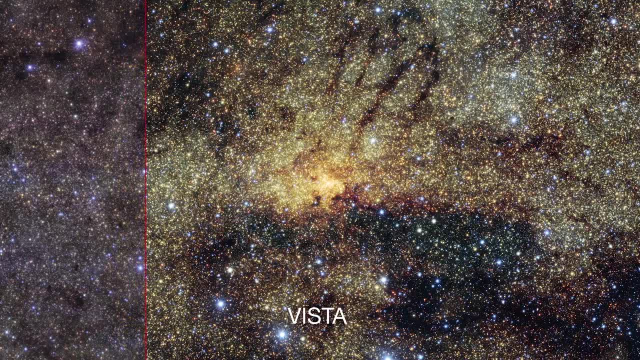 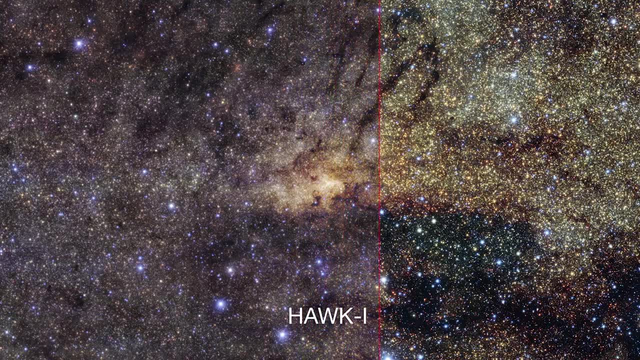 get wiped out regularly all the time, Because once they form and they get this arbitrarily advanced technology- yeah sure they can, They'll figure out some way. Now that's a dangerous galaxy, because then if you have one top dog, 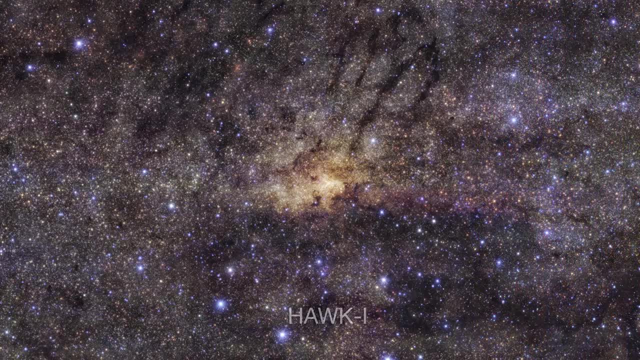 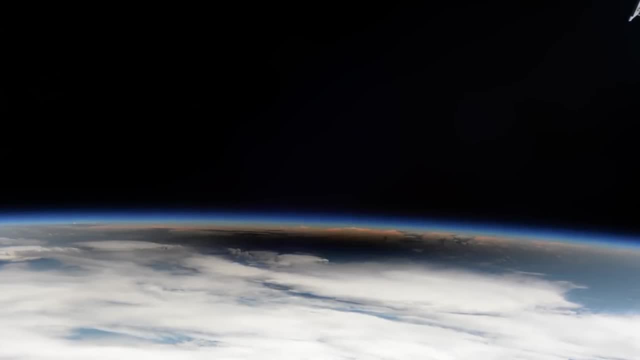 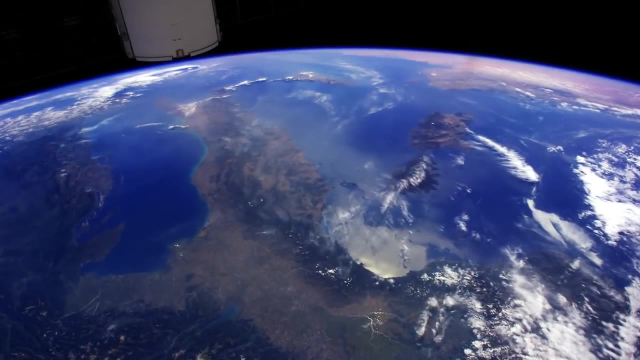 the earliest, presumably the earliest- civilization saying we're going to suppress everybody, then you're in a completely different solution to the Fermi paradox. This is more in the dark forest territory, where something is out there that just keeps everybody down, And I think that's actually even scarier than a gamma ray burst. 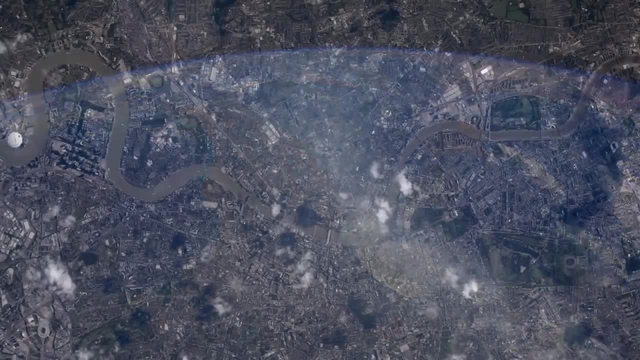 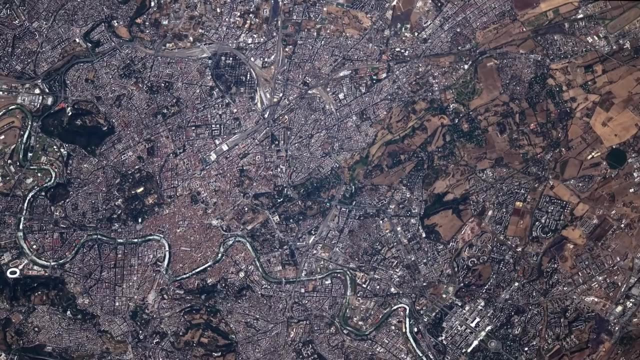 Yeah, I think so too. I mean the way I see it, the way I heard it phrased the first time was in nature: young'uns don't yell, They don't scream, They're very, very quiet. 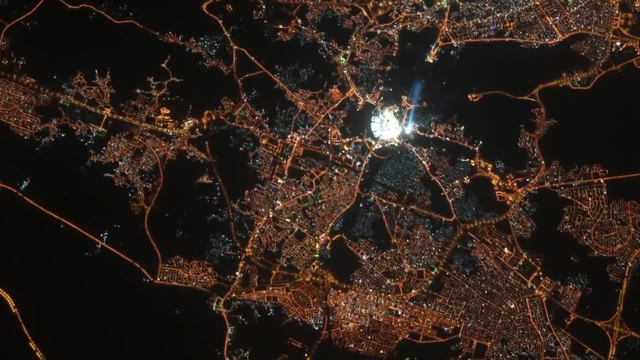 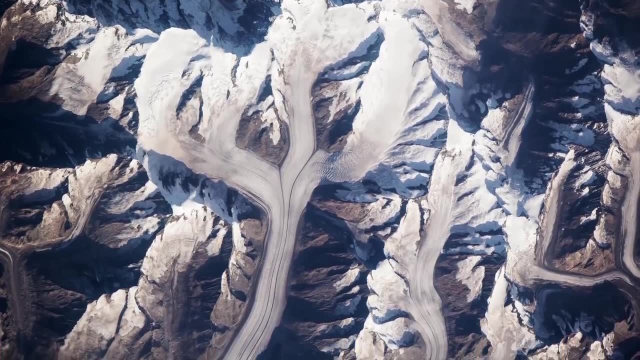 Human babies scream bloody murder because humans are the biggest threat in the ecosystem, the apex predator. in general, Humans in the local universe are acting like human babies. We're just shouting out into the universe like here. here we are, Look at us, Aren't we great? 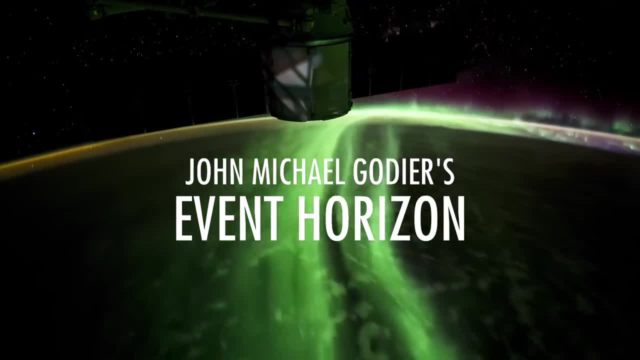 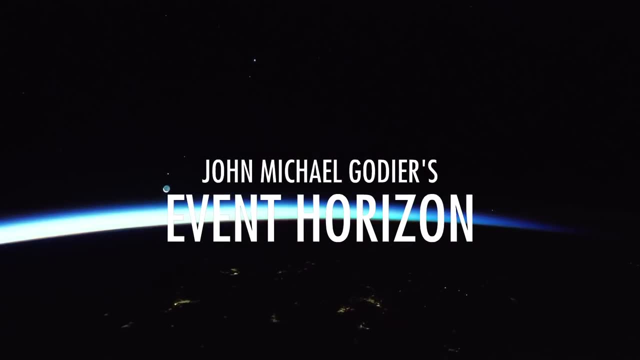 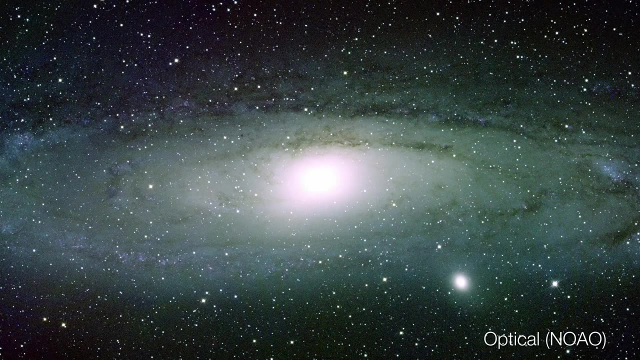 That's. no one else is doing that. That seems like that could be dangerous. I found that argument interesting and a little bit scary. It's hard to imagine human civilization as a progenitor of life in the galaxy. We would be the great old ones. 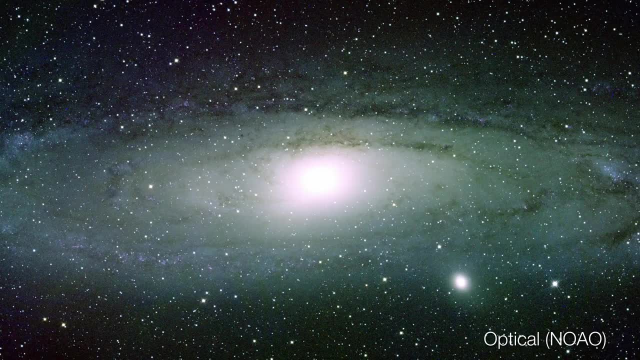 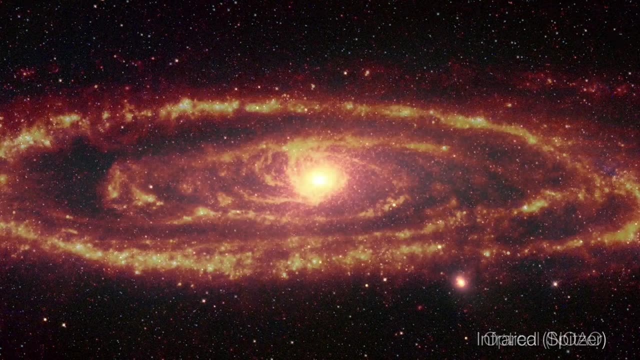 that so long as we haven't gone extinct, could end up the elder siblings in a future galactic community. Maybe we will be the intelligent, advanced, enlightened civilization that sorts out the problems of the galaxy. Some of these new species we may meet. 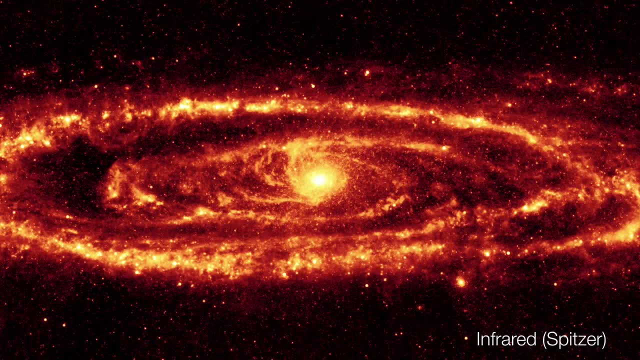 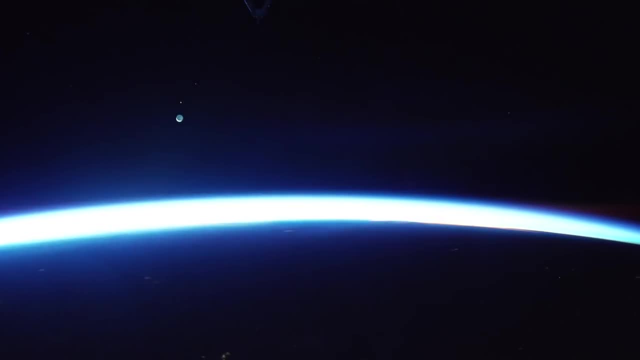 may be completely unrelated, Or still others may be creations entirely of our own design, or even uplifts of creatures who, while otherwise intelligent, lack the physiology or ability for space travel, or even technology. What odd dreams of the future we face. 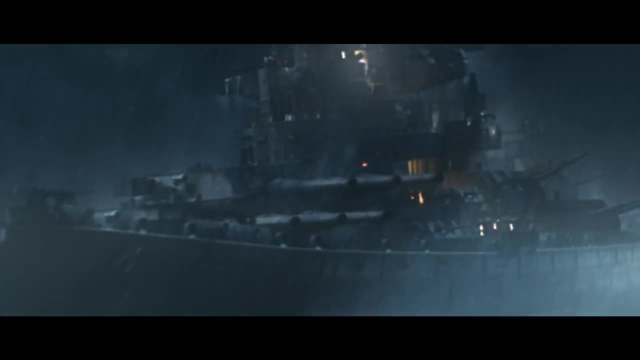 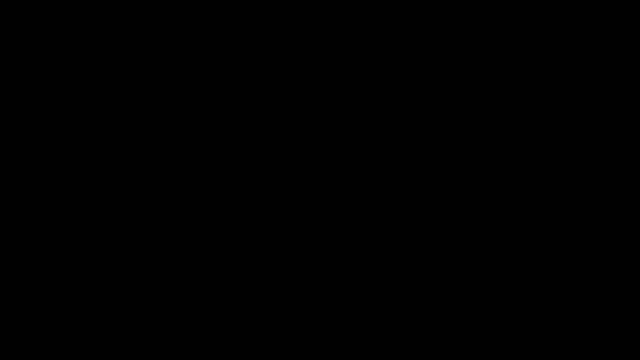 John, What are you doing? I'm playing my favorite game. I haven't even loaded it and my boat's already sinking. They're our sponsors, aren't they, John? I'm happy to say they are, because this is a game that I really love and enjoy.